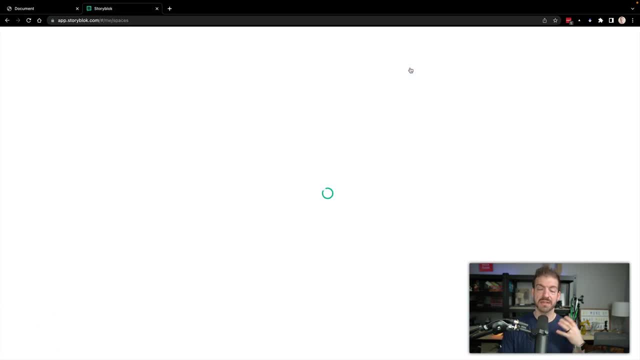 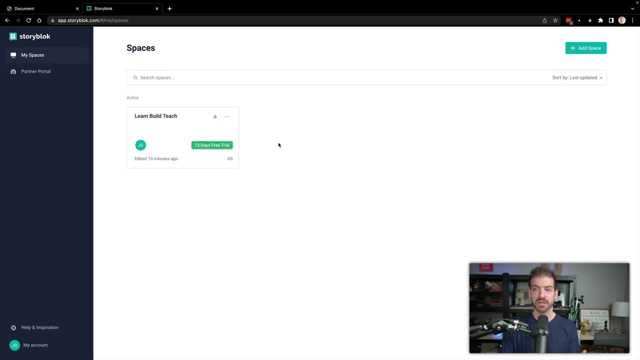 account. This is free. Again, the link for Storyblock is in the description below. I've already signed up before, So after you go through the signup and the login process, you get to a space where you're going to create spaces for your content. So in this case, we're going to create a new space. 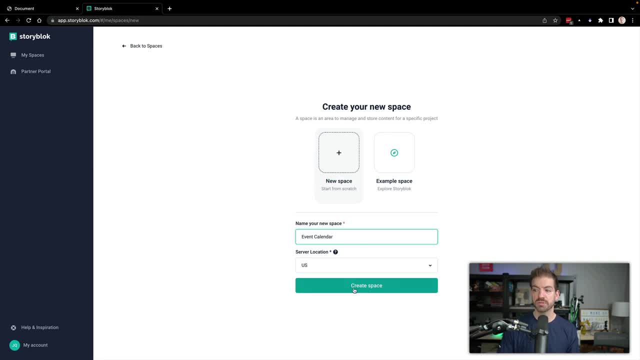 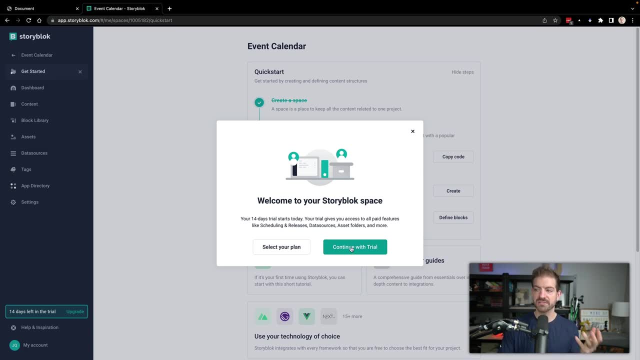 And it's calendar And we're just going to start from scratch. we'll create all this stuff ourselves And notice that I chose us. that's where I'm based, And this is again. free says trial. that's fine. We can continue with the free, free version of this, the community plan, forever, So don't worry. 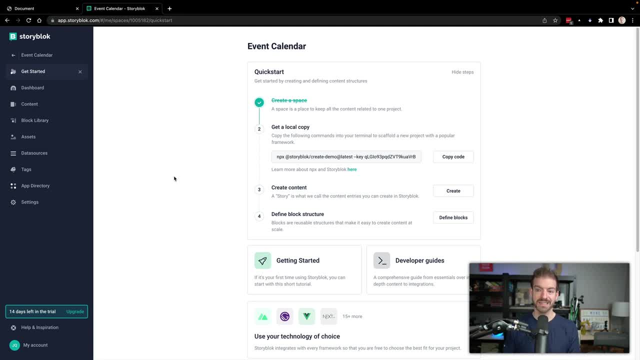 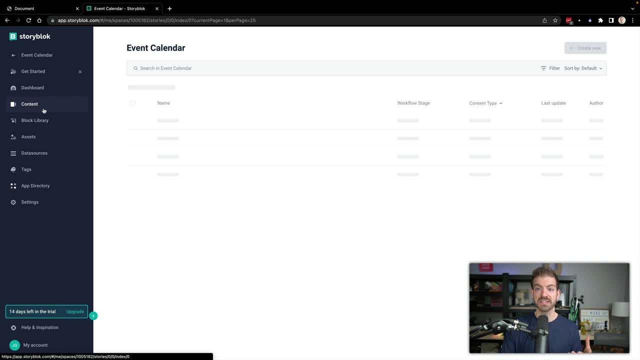 about that. So eventually we'll come back here and start to actually create data. This is what's known as a headless CMS, if you're not familiar with this- a content management system- And so the benefit is that of this is we have the ability to create content in here in a way that's very 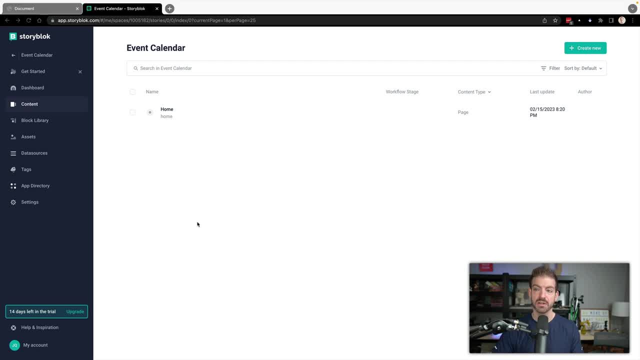 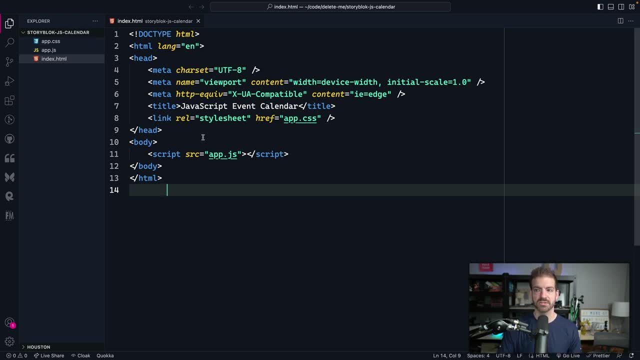 intuitive And then bring that into our applications, which is what we'll see here in a little bit. So let's actually go over to our code. And I've got just a basic HTML file, CSS and JavaScript file. So actually, if you create a new HTML file and do exclamation and enter, you'll get this exact same. 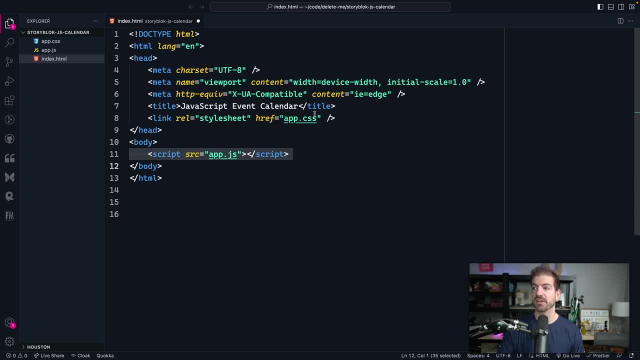 information, except for the links that I added for the JavaScript file and then the CSS file, and then I updated the title to JavaScript event calendar. Now, as we're working on this, one of my favorite things is to use the HTML file to create a new HTML file, And so what we're going to do is 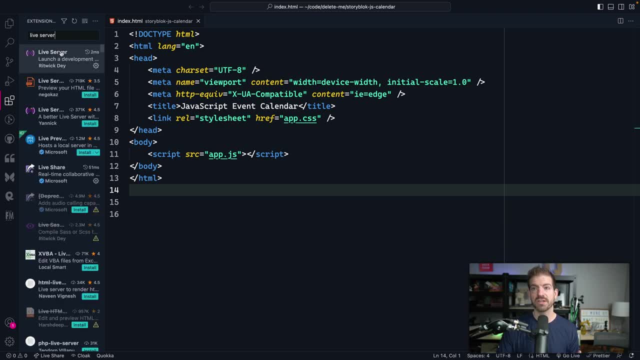 use the live server extension. If you search live server in here, you can click on this and install, and what this does is it gives you a button down here that says go live or run with live server, And this will open up the application inside of the browser And as we add stuff in here, 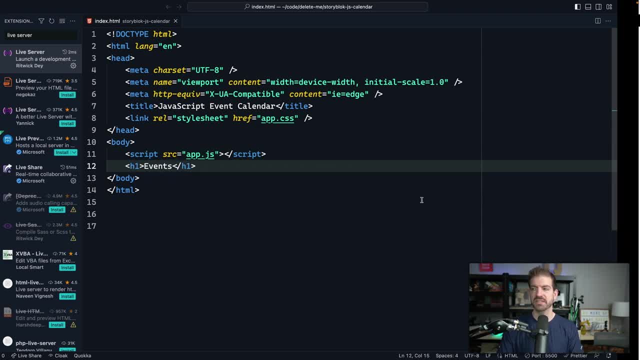 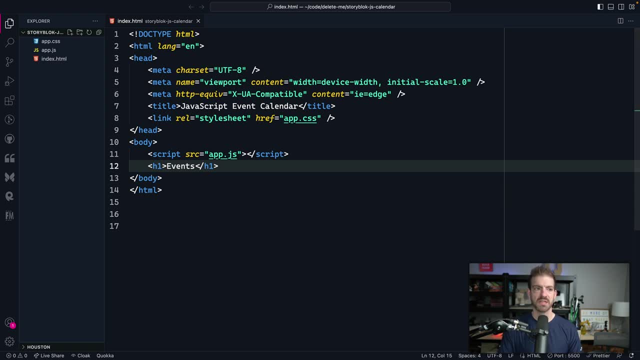 so if we add an h1, with the text events, we'll see that show up here. So this is actually really, really nice. It's my favorite way to just do basic HTML, CSS and JavaScript. So let's start with a few basic styles. These are kind of going to be like reset things, just 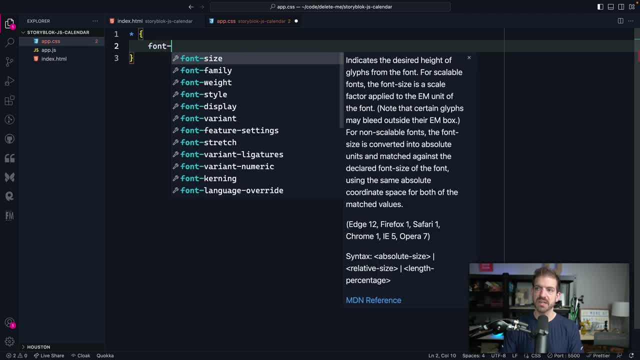 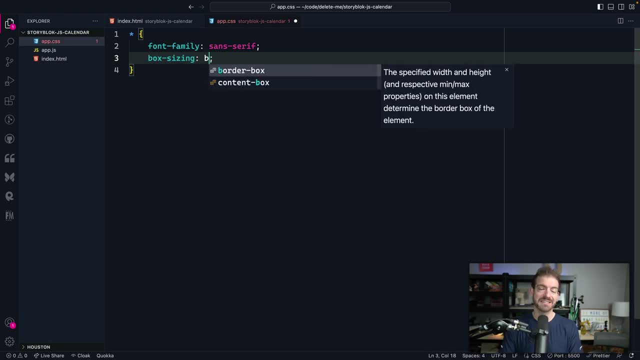 to kind of set the tone for the application. It's not much. we're going to set the font family to San serif- This is a little more modern than a serif- And then we'll set the box sizing to border box. This means that if you give something a width, it's going to include the padding inside. 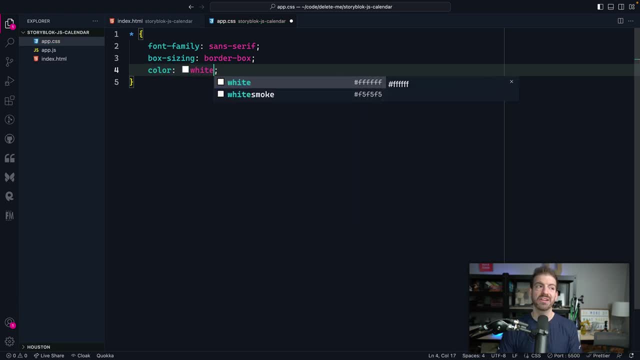 of that, for example, And then we'll also have. I will set the color to be white for for all of our text. then inside of our body we're doing just a reset here of margin zero, padding zero, And then we'll also set the background color to this fun. 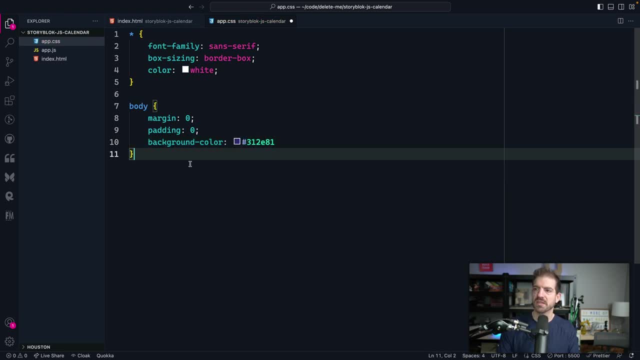 kind of dark blue. So it's 312 e eight one. Alright, so now we should see that we have that, we have our events in here, And the other thing I want to do is add a container. So usually containers are used to kind of center things on the screen and give padding on the outside. 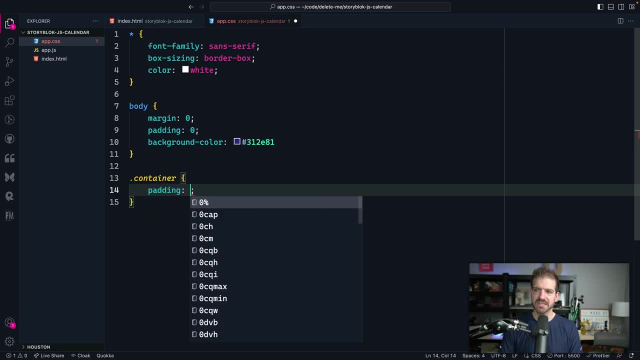 So this is almost the default stuff I use in every one of these demos. So inside of here we'll have a little bit of padding. we'll use the margin. zero auto tricks. this is going to move If we tell it to take up, which we will do. a width of 1200 pixels If the screen is wider than. 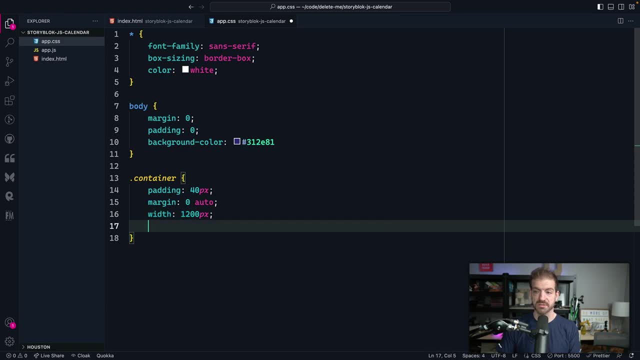 that margin zero. auto is going to automatically kind of shift the content to the middle, which is what we want. Now we're also going to use a display of flux. this is CSS flexbox, which helps you kind of position it And you can kind of mixing it all in just one scale, And then you can. 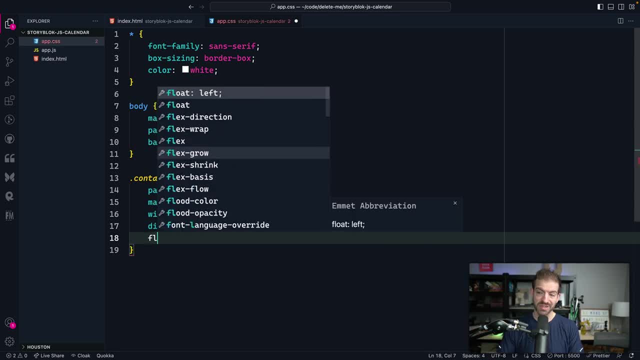 things either horizontally or vertically, And actually in this case we're going to change the direction of this to be column. I'll show you what changes if we don't do that in a second. So what we need to do is actually use this container class. So I'm going to wrap the 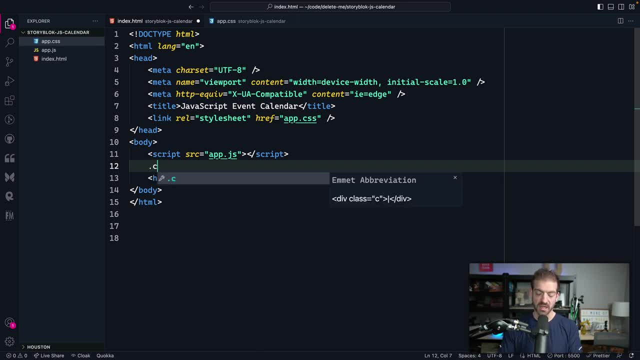 events h1 in a container or a div with a class of container. Little shortcut here is you can use emit snippets to do that. So dot container, you can see, generates that for me. So I can surround events here. And if I do a second thing just for testing of like calendar, we we can see what this. 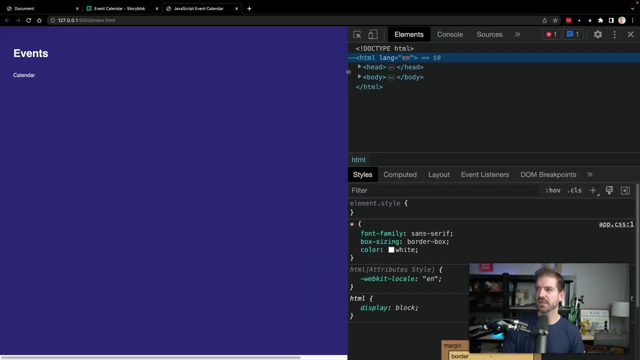 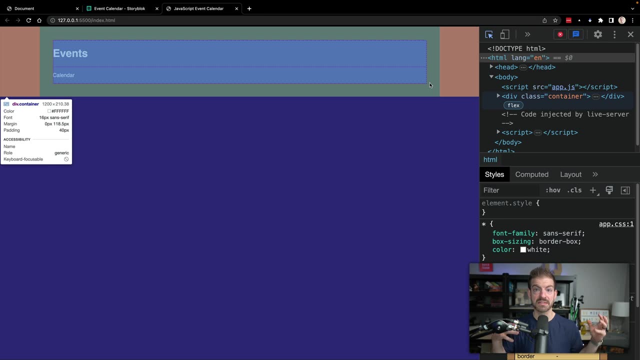 looks like. So notice that it's taking up a width of 1200.. If we come in and do this, so the width of this is 1200. And then you have this margin on the outside. So that's the margin: zero auto to. 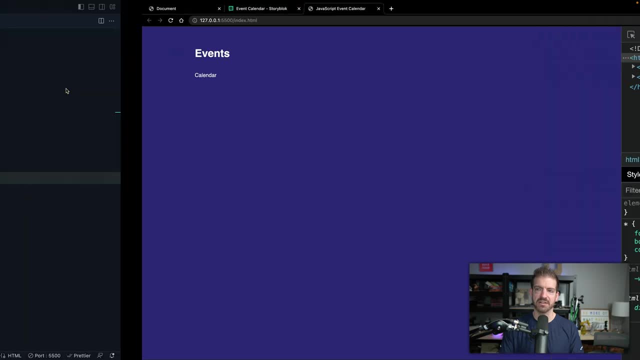 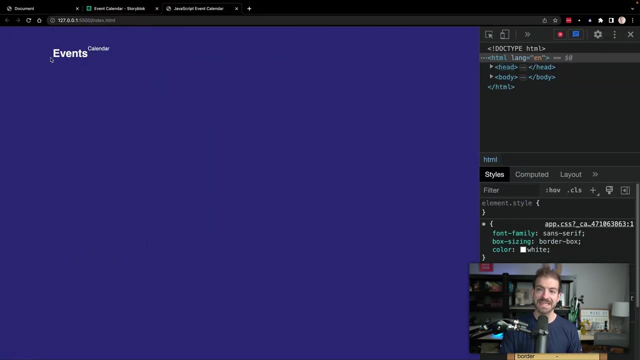 center this stuff And then these things are stacked on top of each other. events and calendar. If we were to take flex flex box and remove the flex direction, by default it's row. so notice that stacking these things. actually it's not stacking, it's aligning them. 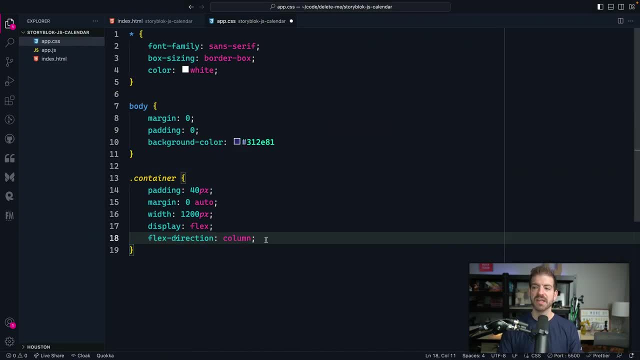 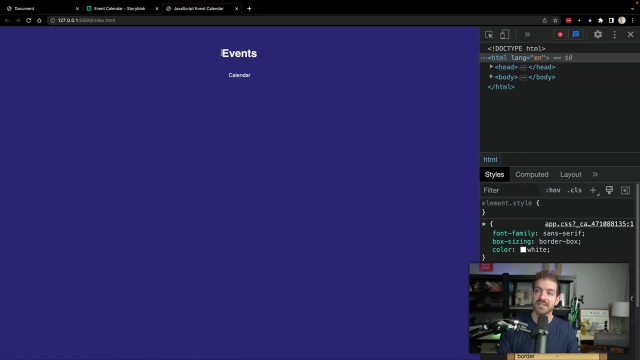 putting them all in the same row. So in this case, we want to actually stack them, And the last thing we'll do is do align items center, And so what we're trying to do there is center this content on the cross axis, in this case, which is centered horizontally. So since we 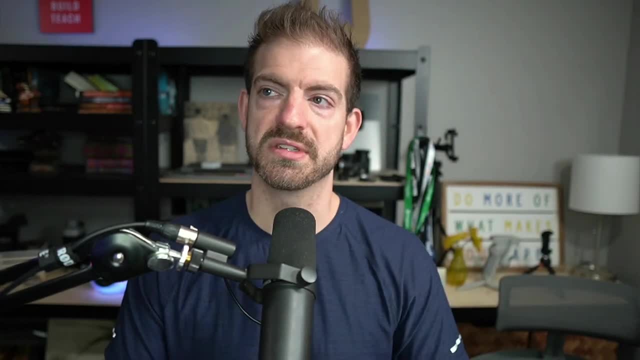 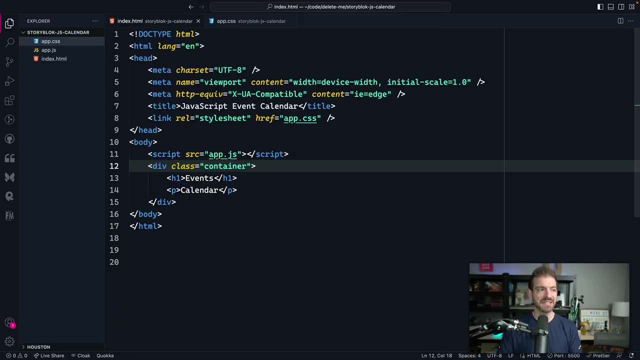 tell. tell it to be column. now the cross axis is going to be horizontal and align items is how we position things on the cross axis. All right, so that's our base kind of styling in here In the HTML. we're not going to have that. 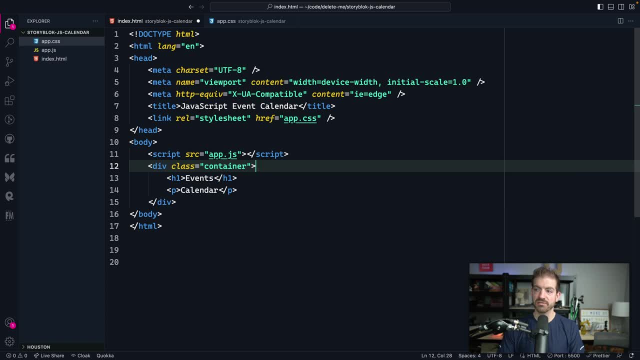 much. we're going to have a another section here for header. So this is going to be a div with a class of header again, dot header. you can type this out, but I encourage you to learn Emmet snippets. So we'll have header inside of there. we'll have our text for events. we're also going 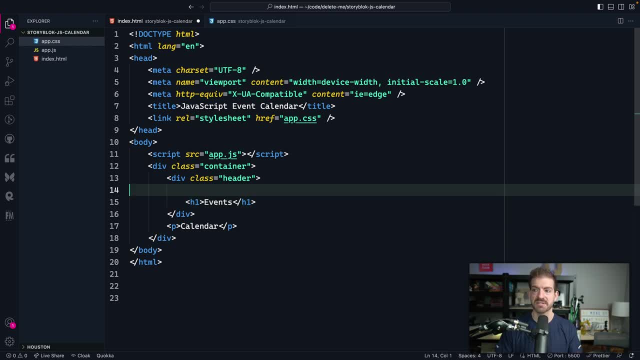 to have buttons to go to previous and next months. So we'll come back to that. But we'll just make sure we have our text for events. So we'll come back to that. But we'll just make sure we have our text for events. So we'll come back to that. But we'll come back to that, But we'll make sure we have. 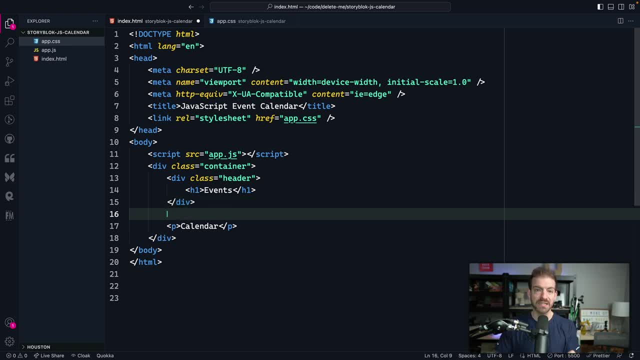 this header already marked And then we want a div with an ID of calendar. So to do this, you can just do hashtag and then calendar and that's going to generate a div with an ID of calendar And that's basically all we need in here. we're going to come back and add these forward and 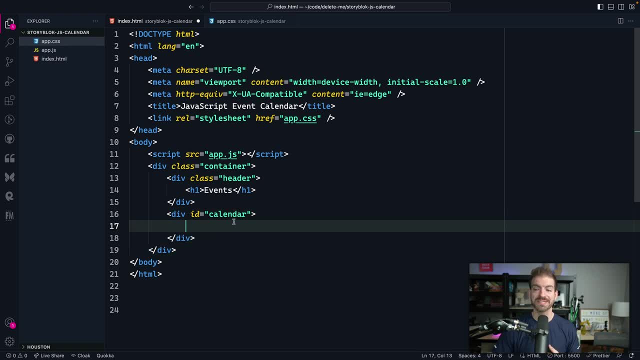 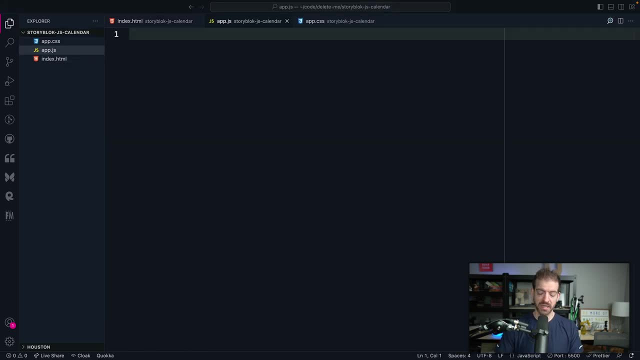 backwards buttons. we are then also going to dynamically generate all the days and stuff for the calendar inside of JavaScript, which is a lot of fun, So let's go ahead and start to do that. So we're going to create a function, draw blank calendar And basically, 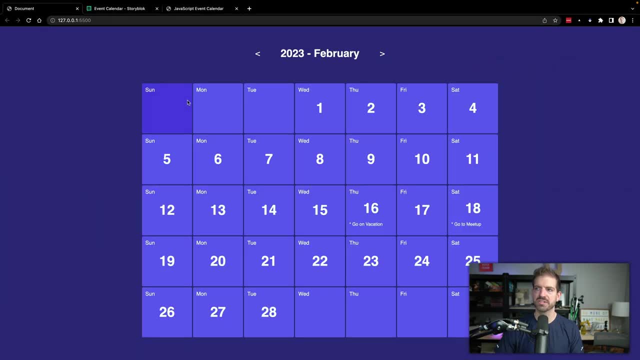 what we're going to do is, if we look at this original version of this, we're going to now create 35 different boxes, So seven across and five down. we're going to create a blank box for each one of those and add on the label for the day. So that's what we want to do, And we're just 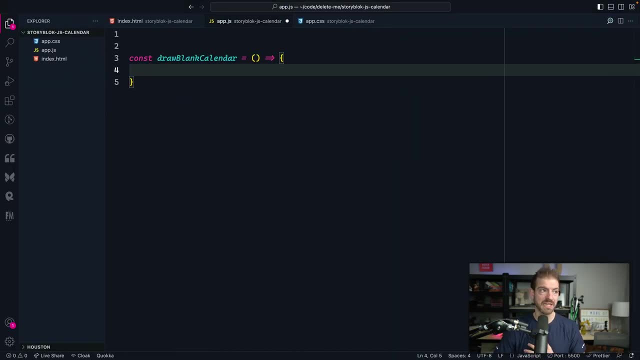 doing this in JavaScript because it's going to be in my mind. we're going to be doing this in a little bit easier, although you could absolutely do this in your HTML as well. I think it's just a fun exercise in in JavaScript. So we're going to iterate through, we're for loop, we're going to. 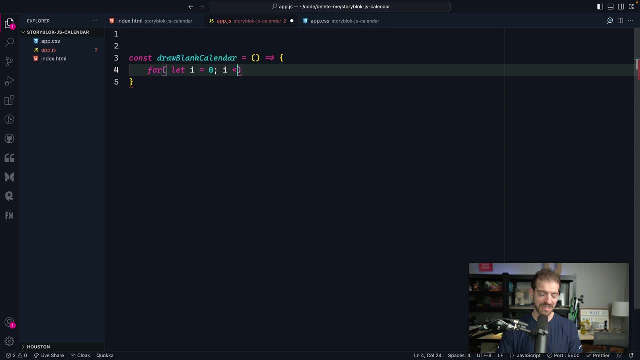 start with, let i equals zero, I less than 35, again, and then I plus plus. All right, and then what do we want to do in here? Well, we want to create the elements for each one of these blocks, So the each block here is a div. 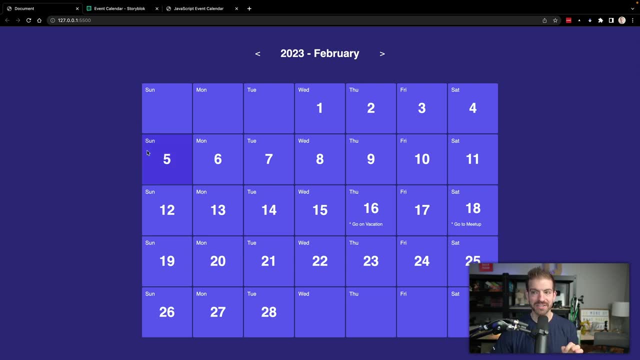 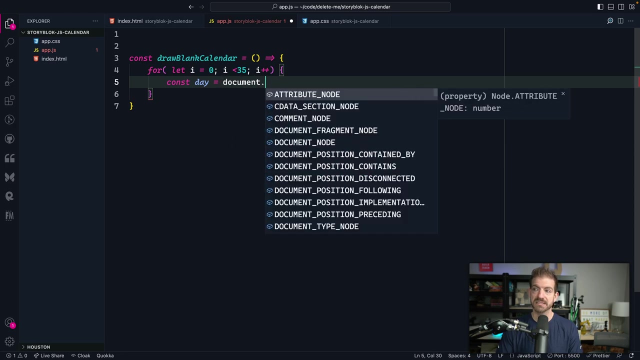 With a class of day and then inside of it it has an element for the day text, the day number, and then what we'll get to is the event name, if there's an event on that day. So we're going to create each of these with JavaScript. So we're going to say our day is going to be document. 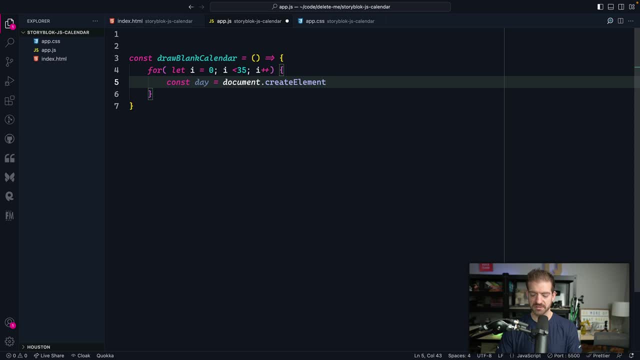 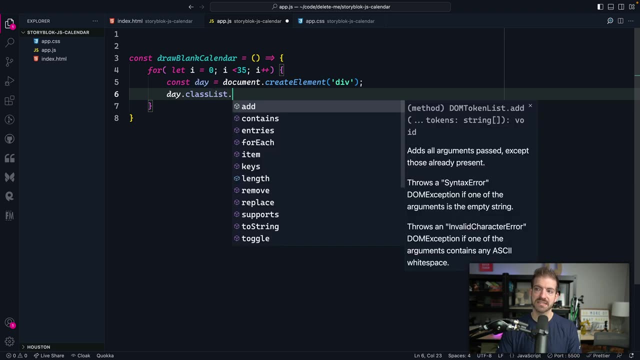 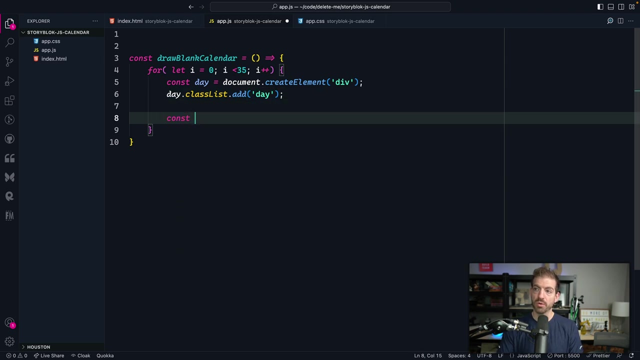 dot create. So this is how we create elements in JavaScript And we're going to create a div in here, And then we want to add a class to this. So we'll say div dot class list or data class dot Add. So this is how we add classes and JavaScript, So we'll have that one. We'll then. 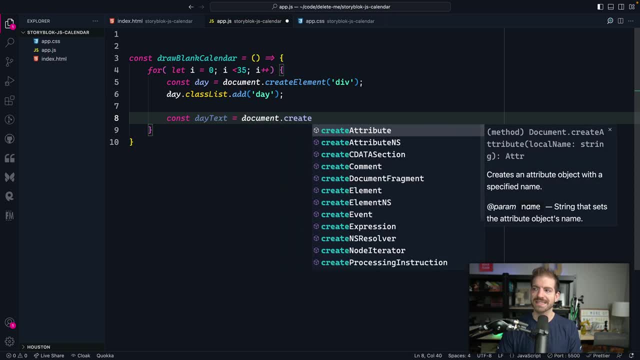 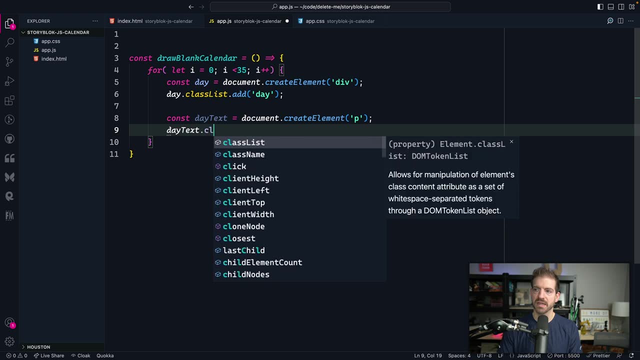 have very similarly. we'll have a day text, So create elements, And this will just be a p tag. we will add a class to that, So add this class of day text. We will also have the day number, so we'll create an up an element. 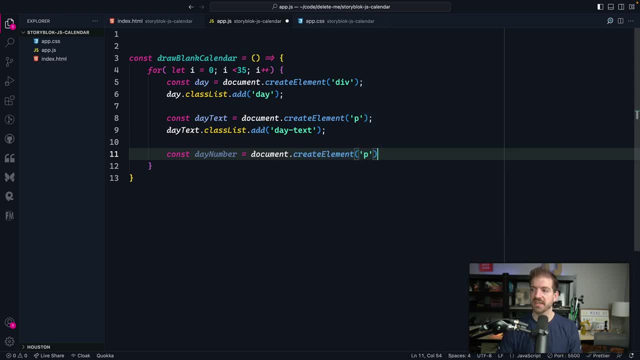 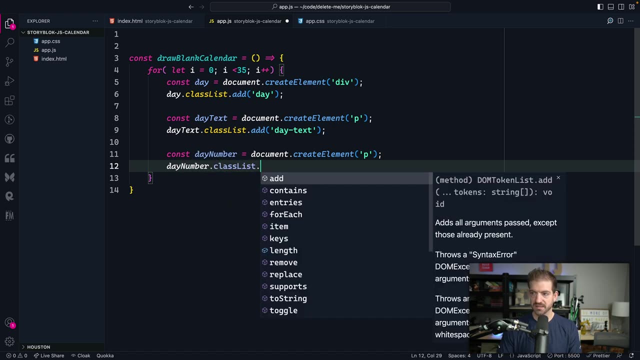 for that create element, And this will be a p tag as well. We'll also add a day number, a class list, And we'll call this day number. Notice: I'm using hyphens and all lowercase in here. That's more of the convention for classes in CSS and HTML that you'll see. And then, lastly, 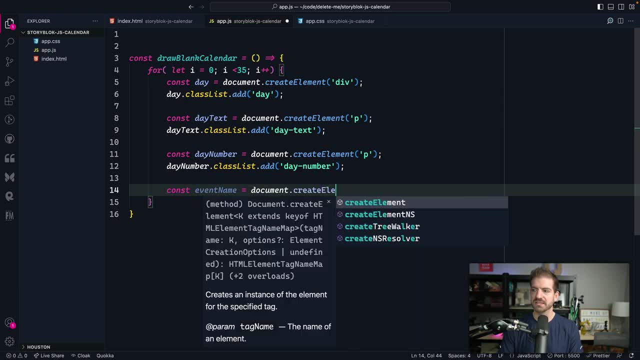 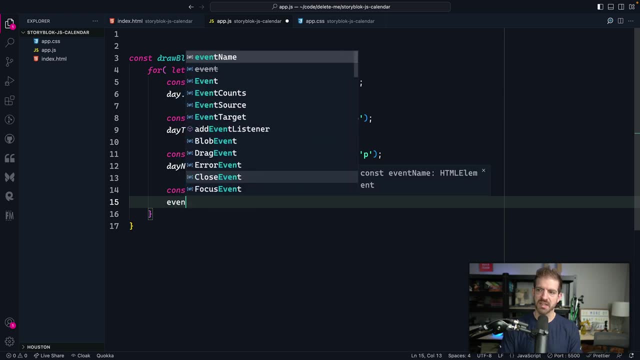 we'll have an event name, So this will be document dot- create element, And this will be. we'll list this as a small element because this is going to be a little smaller than the rest of the text, And then we'll do the exact same thing. We'll access the class list. we'll add a class of event. 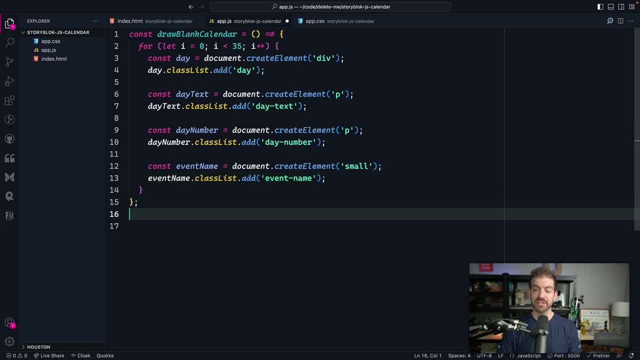 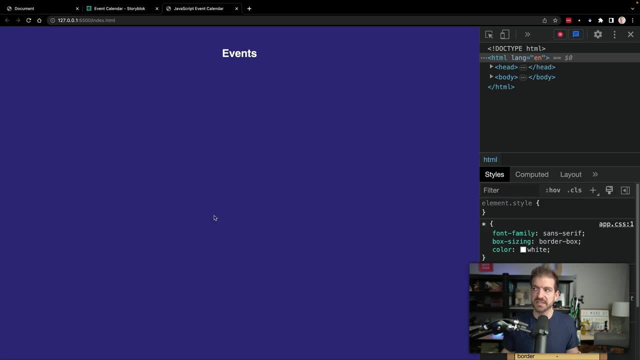 name. So one thing we haven't done is actually call this function. So let's call draw blank calendar And you may expect things to show up, but nothing's there. And the reason is we've created these elements but we haven't actually attached them to the DOM. So what we need to do 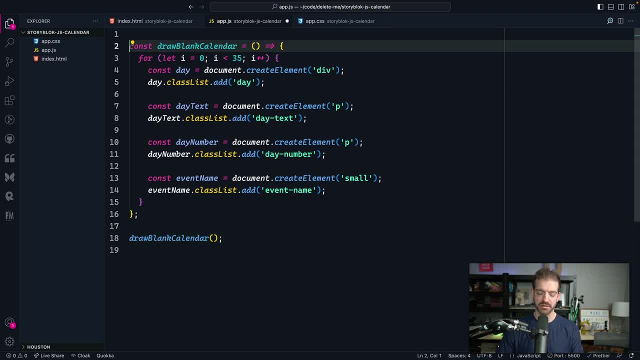 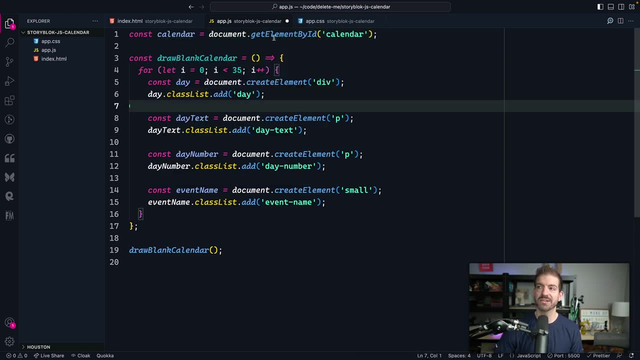 is take these elements and then add them to our actual calendar. So I've got a little snippet in here called get ID, And I'll show you what this does in a second. What this does is it creates a snippet that calls document dot get. 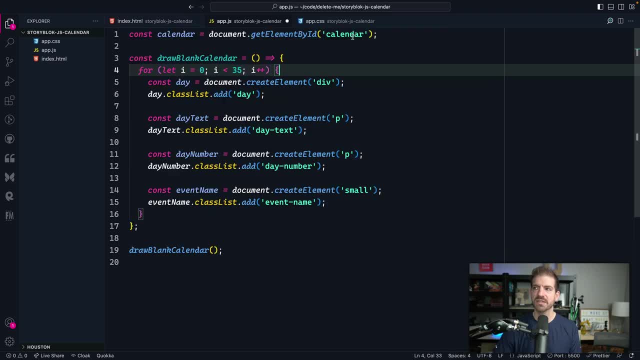 element by ID. If you remember, we have the ID of calendar in here. So, requiring this div element by its ID, we get a reference to it And now we want to take the day and append that to our calendar. So there's an append child function And to our calendar we want to add a document. 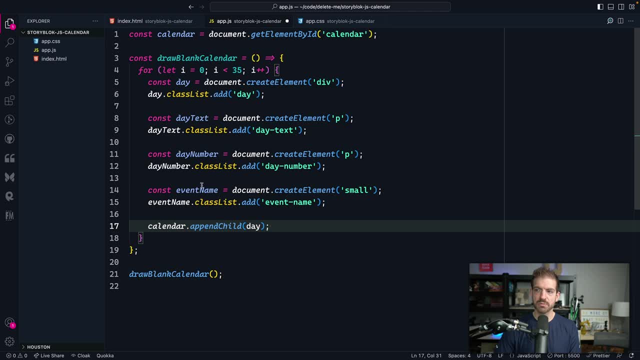 that has a call And then we can show this object that we just created. We'll just see if we can see how this will and I'll tell you where we're going to save this. So we'll just add in the day Now. the other thing we didn't do is we want to add the day text. 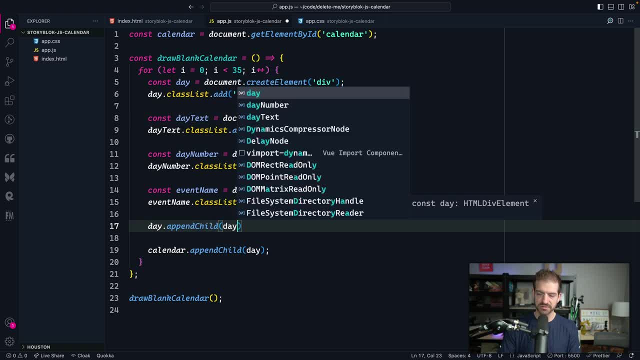 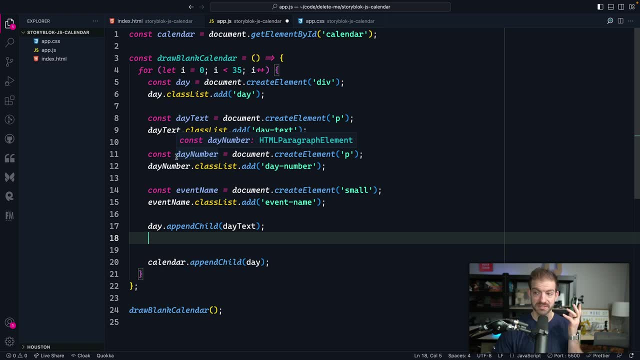 a number and event name all to that day as well. So for the day, we will call append child And I'm going to do something that will be a little tricky. So let's actually show you. I don't know what's called a fancy way to do multiple cursors, So I'm going to click a cursor. 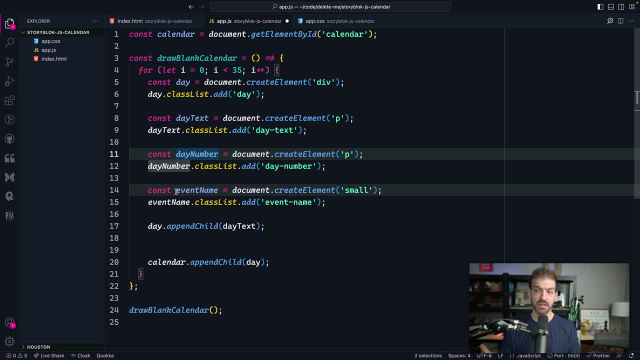 here. I'm going to click a cursor here And the second option, or the second way to click that cursor- the second to get the second cursor- is a hold down option and click on Mac And I guess that would be alt on Windows And then I can select both of these, copy them, And now I can. 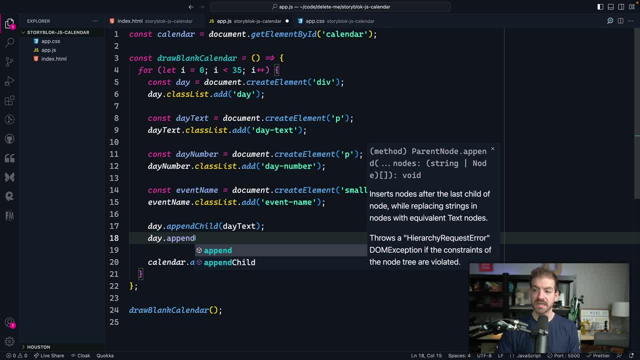 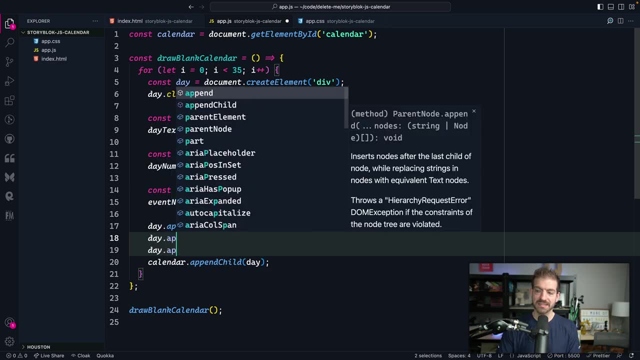 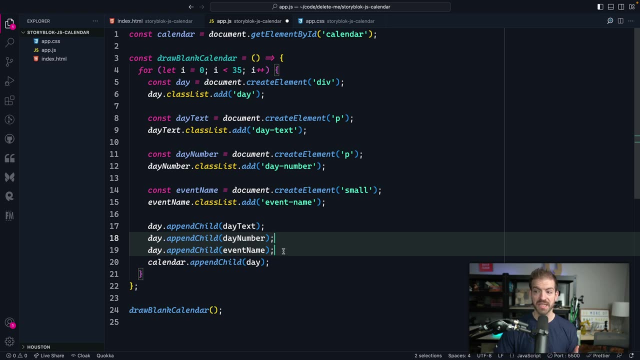 come down and say day dot, append- Actually I need to get a second cursor here, All right- and then call day dot, append child. And then, since I have two things copied to my clipboard, it's going to paste both of them in appropriately. So we add those elements to each day, If you. 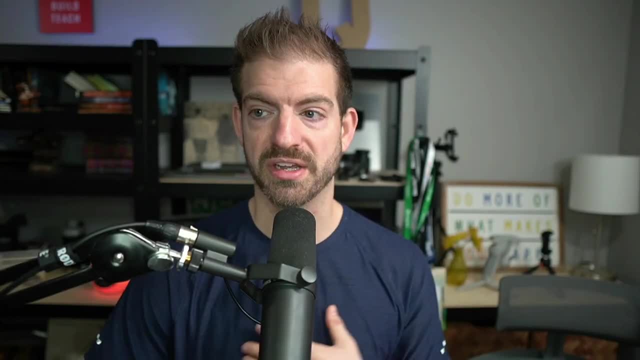 didn't get that. that's okay, the cursor stuff, but it's fun to work with. I encourage you to try them. We're going to add those things to the day And then we're going to add the day to the day And then we're going to add the day to the day And then we're going to add the day. 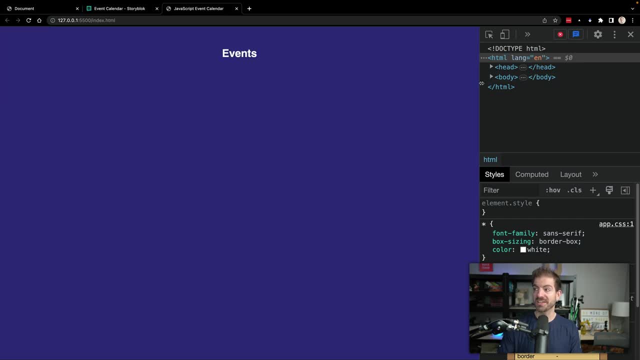 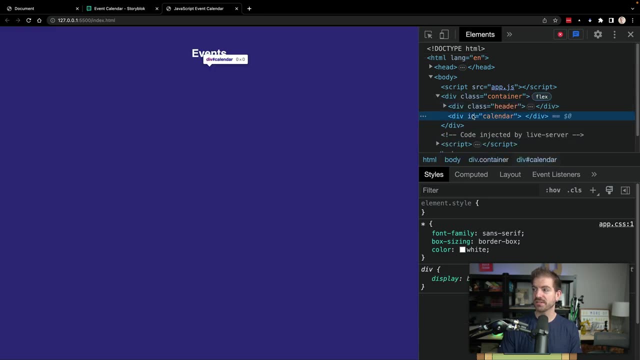 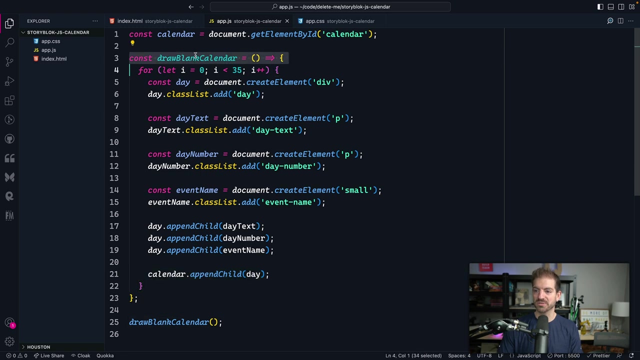 to the calendar. So we don't actually see anything because we don't have any styles. But inside of the body- hopefully we have a calendar in here that does have nothing in it, So we need to actually check what is going on in here. So let's make sure we're calling the right function. 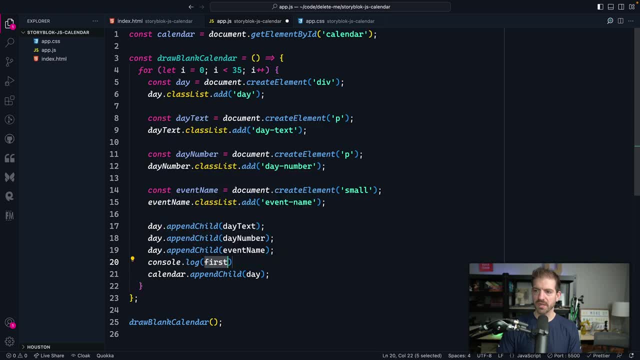 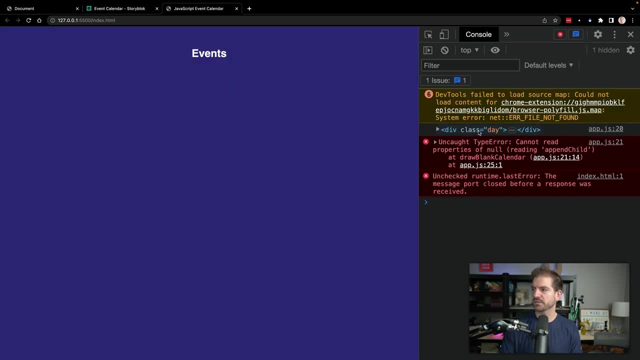 it looks like we are And we can log out a day object in here, just to kind of see if we're getting that correctly. So let's go to the console. it looks like it's logging one And then it looks like maybe we're not accessing the calendar. 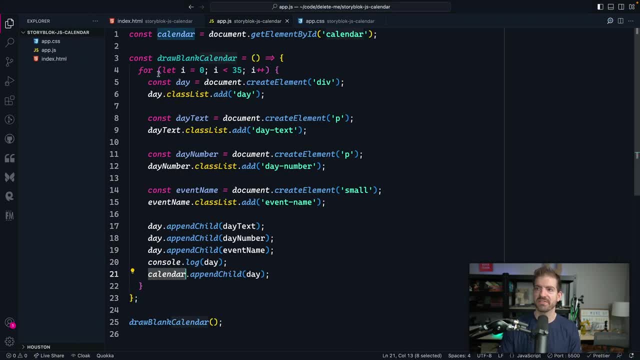 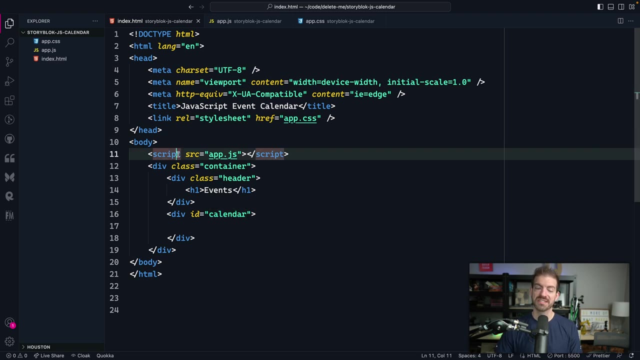 correctly, So we're able to create the day, But when we try to reference this calendar, it's not fine again. So let's make sure in the HTML that this ID matches up with what we have here, And it does. But I think we're missing one core thing, which is that the JavaScript should: 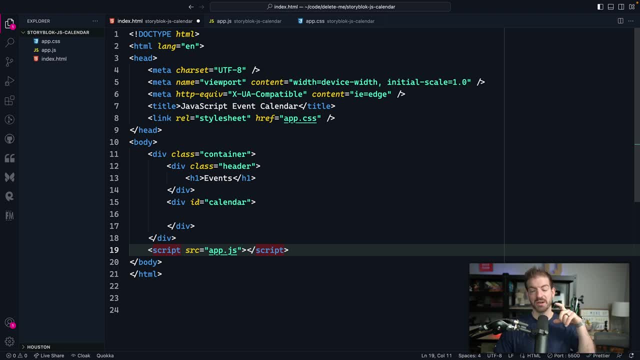 be loaded after all of the DOM elements. I often go back and kind of put them in the wrong position, But this is a good learning experience of the script tag should go after these elements are loaded, Otherwise it won't have it won't have access to those elements. 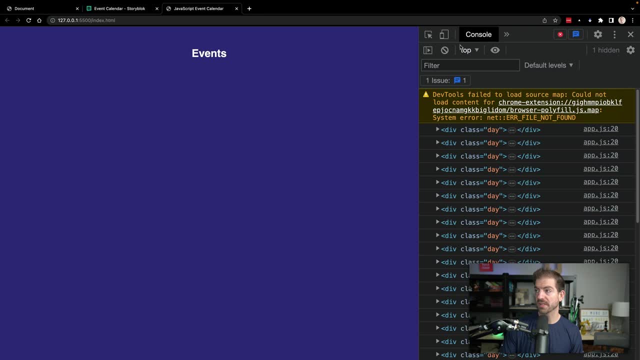 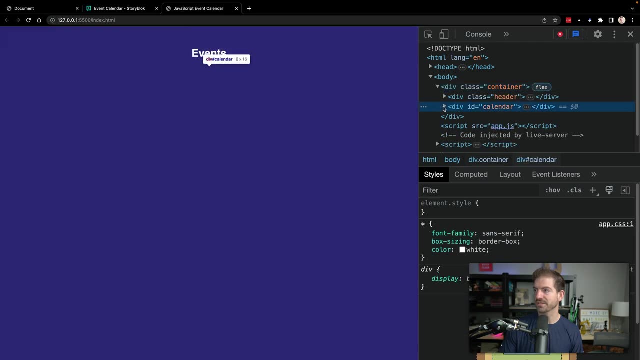 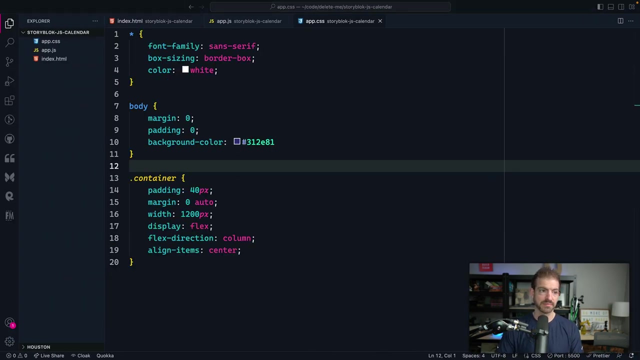 So let's save this. we shouldn't see much here, although we see the log, And then, if we go inside of our events and go down to in the container in the calendar, and then you see all of our day classes. So now we can start to do some of our basic styling with our days. Alright, so let's. 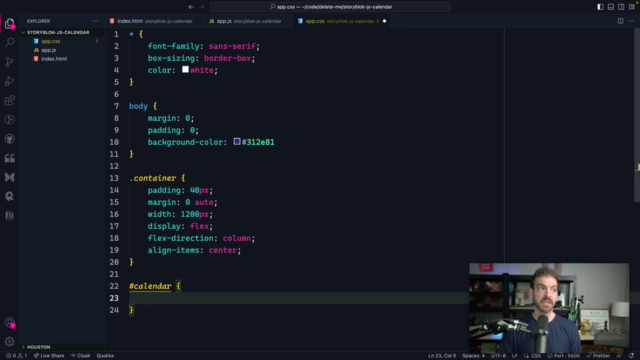 go back to our calendar, So our ID of calendar and we're going to use in this case display of grid. So with our grid we can define rows and columns and we can actually have them like automatically wrap. So we're going to say this is a display of grid, then we'll use grid template. 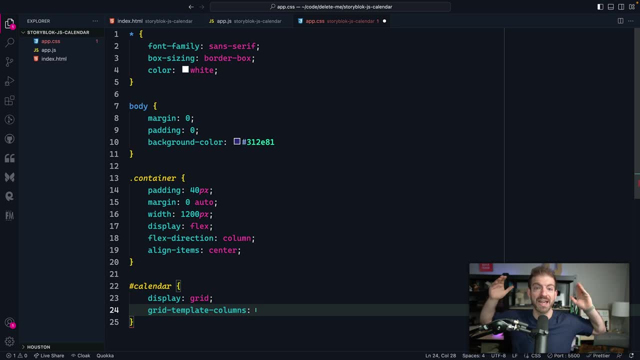 columns, And what we want to do is we want to define. this thing is going to have seven equal columns, So you could. you could say 100 pixels, 100 pixels, 100 pixels for each one. But there's also a repeat function And so we want to repeat. 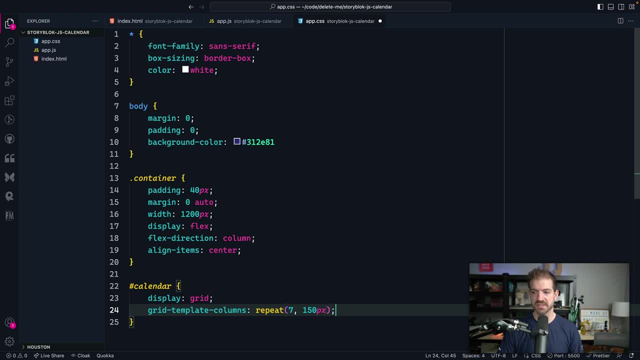 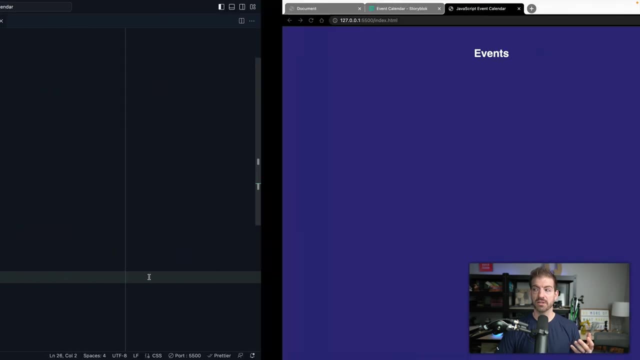 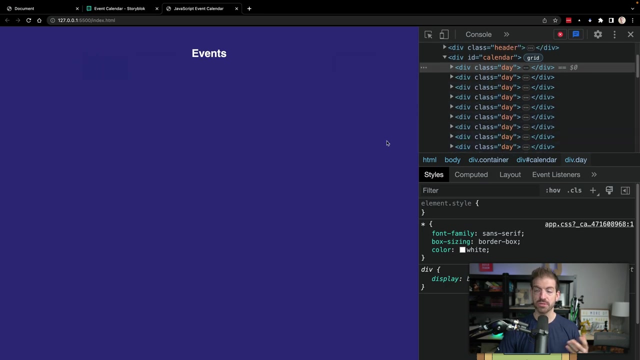 times, with a pixel width of 150 pixels in this case, And then we'll see. I'll show you gap here in a second. So that is our calendar. that should now be laying these things out. If you look at this, they're now laid out horizontally until they wrap and come down to a new row, So that 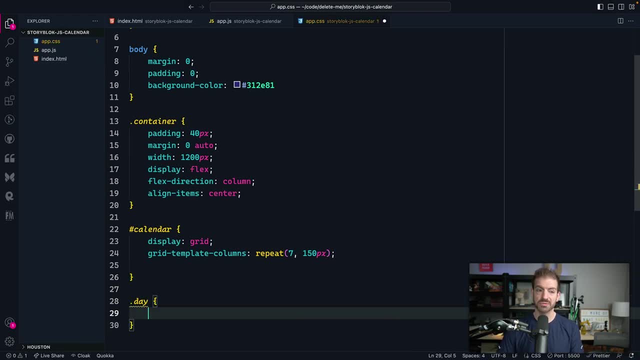 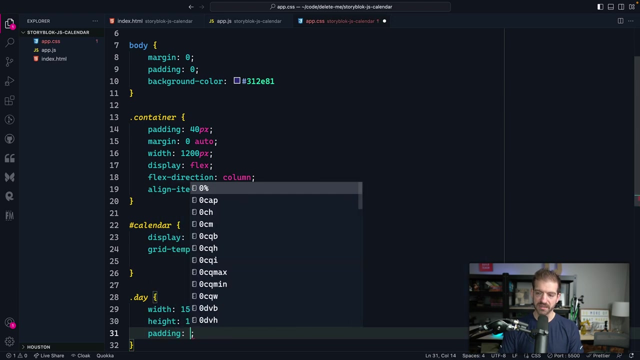 looks good. And then now we need to start to style the actual day objects, And the main thing we want to do here is give a width and a height. Actually, those are individual things. So 150 pixels and then a height of 150 pixels. We'll add a little bit of padding, so 10 pixels for 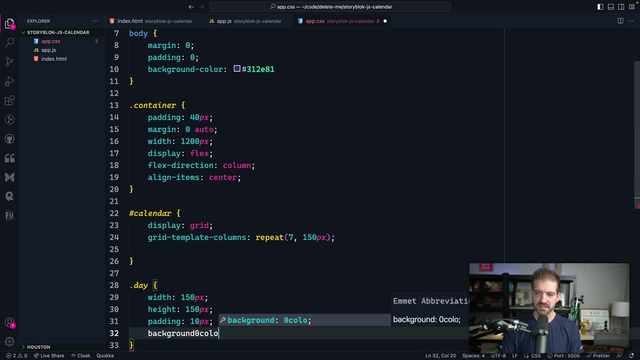 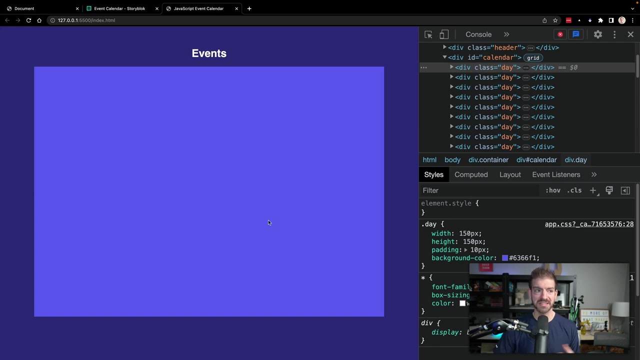 padding And let's do our background color, background dash color of 6366 F1.. All right, so at least we'll be able to see these now And notice these are all basically just look like a solid block, So we can't tell the difference between them. So one of the things that we can do, 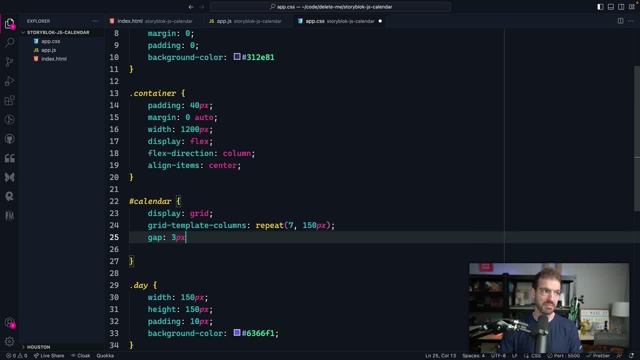 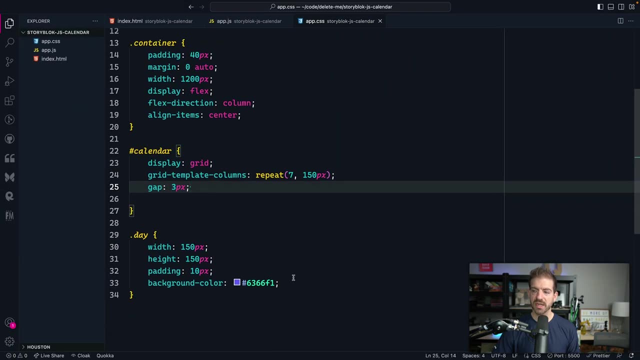 is, add a gap in grid So we can give this a gap of three pixels or something, And basically this is going to create space in between each element, which is really cool. And then I also want to add a little bit of border radius to this, to round the edges just a tad, So you'll see this. 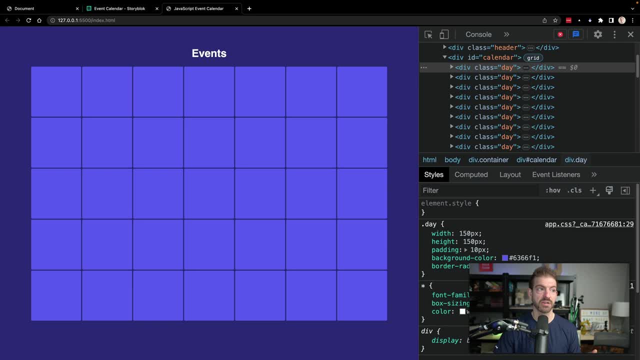 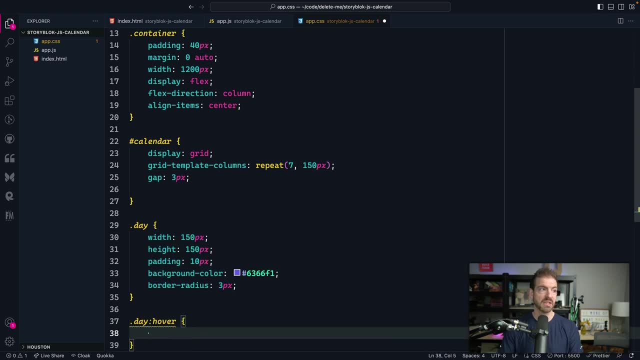 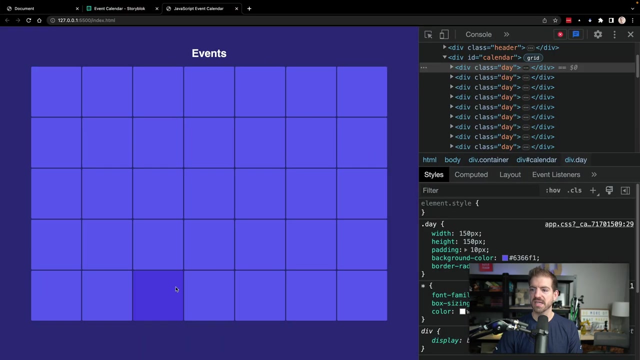 rounds them just a tad, But it's starting to look pretty good Now. the other thing we did is add a hover effect. So if you take day and then add the hover pseudo selector, we can change the background color. we can change this to a slightly different blue. So for f, for six, e, five, And so as we go. 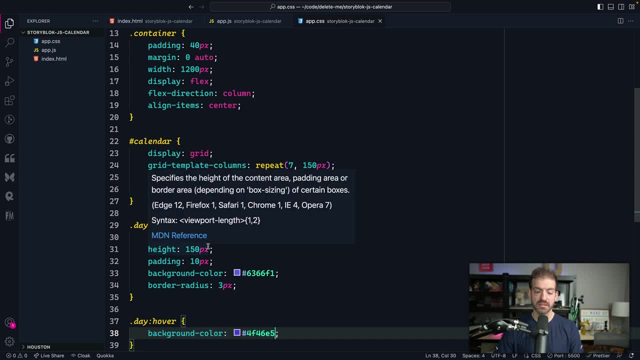 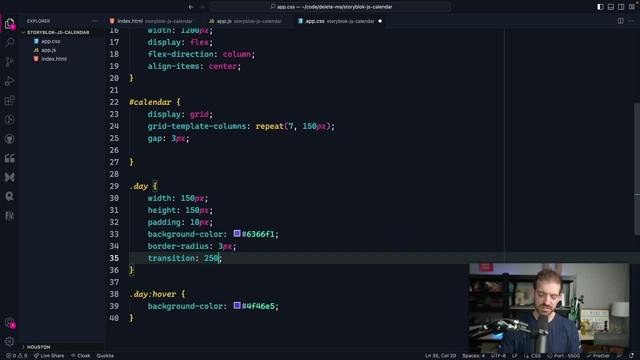 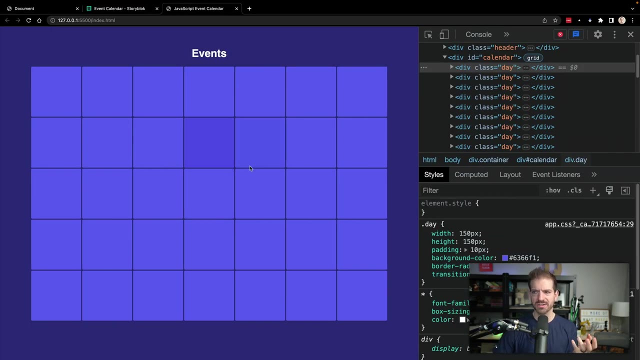 we'll see it change colors, which is great. The other thing, The other thing that we'll do, is add a transition of 250 milliseconds on all properties, So this will just make that not like kind of fade in or change colors With a with an effect- transition effect- instead of just automatically becoming that thing. 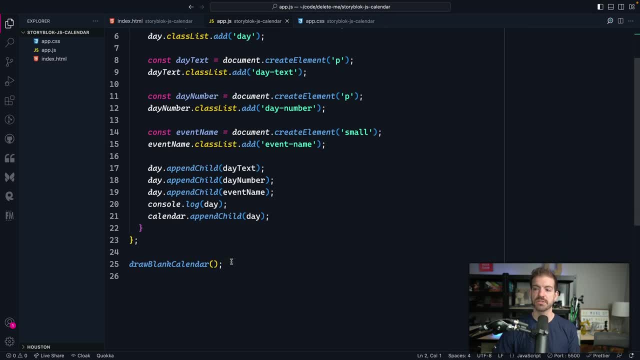 Alright, so that is looking pretty good. Now our next thing is to start to start to actually update the calendar, And so we're going to have an update calendar function- update calendar- And we're updating this by month. So what we need to know is the month, the year. 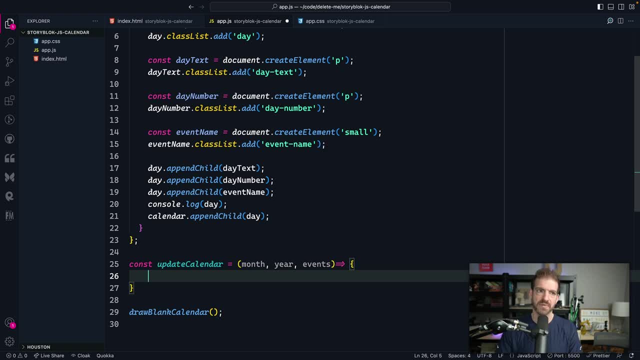 and then eventually we'll get to the events that we display on here, but not yet. So we want to do, we want to query for all of the day elements, So all of the ones that are inside of the document. So we'll do a document query selector, all with a class of day, So all those elements that we just 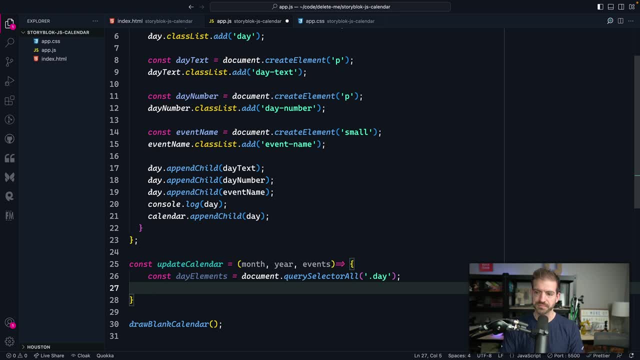 created. each time we update this calendar we're going to get a reference to each one. Now I want to get a reference to the first of the month And I'm going to call this the first and just call new date. But when we create a new date, it doesn't give you. it doesn't give you the first. 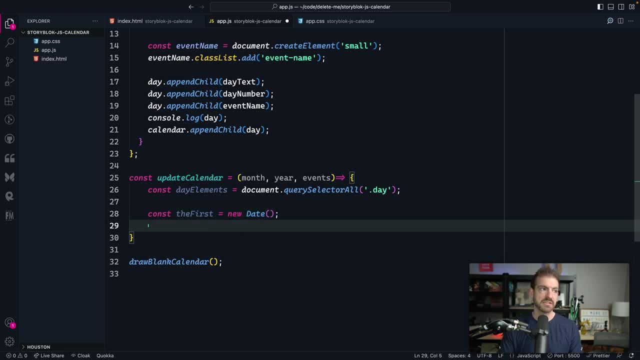 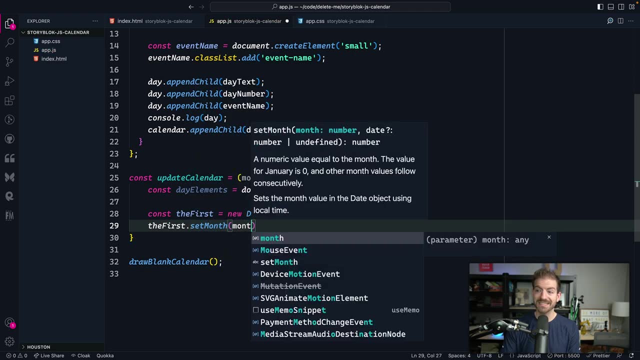 of the month. it gives you, like right now, the time and day of right now. So to change this, we can say the first and say: set month, And then we want to set it to the month that we're getting inside of here- All right, that parameter. And then we'll do the same thing for year. So whatever. 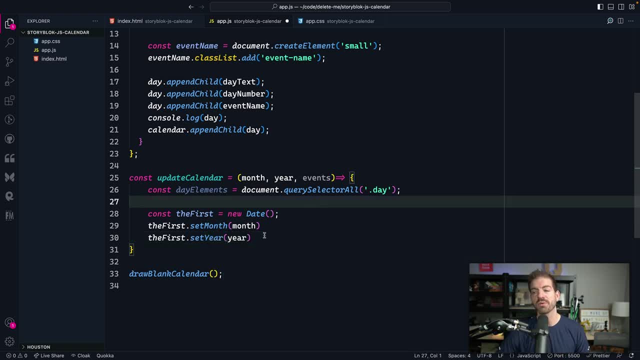 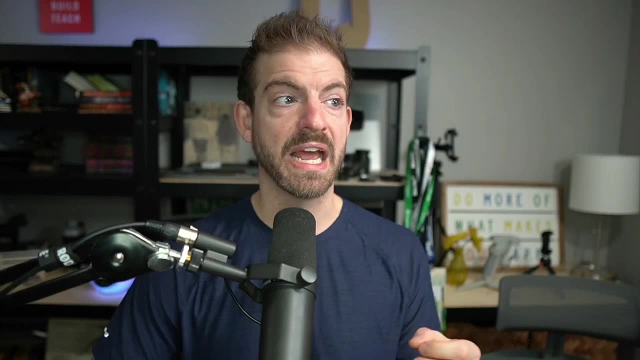 that parameter is that we are getting for both the month and the year. we want to get the first day of that month in that year, if that makes sense. And now we're going to use that to kind of iterate, And then we're going to go through the days inside of our grid and update them accordingly. 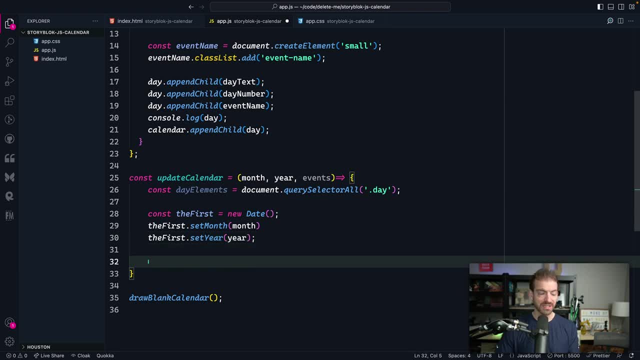 All right. So the other thing we want is the first day of week. So we want to know, like, basically, what day of the week does the first fall on? and so this will be, we'll take the first and we'll call get day. So this gets the day of the week, Cool. 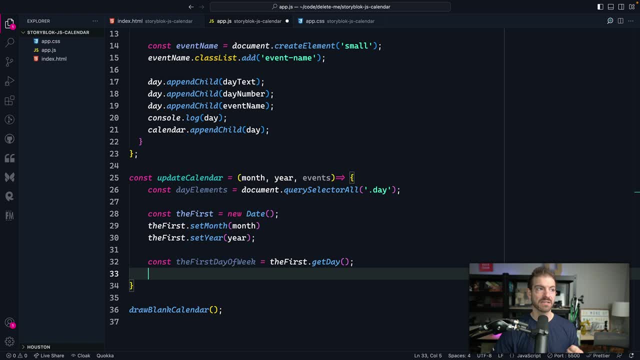 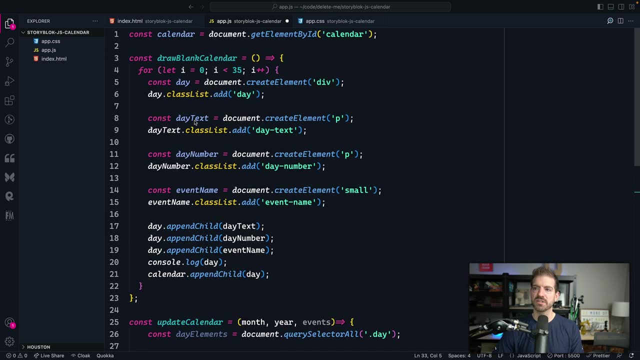 And then now we also want to be able to do that, So we want to display what the month and the day are. So I'm going to copy in two arrays here, So one for months and one for days, so that we don't have to type all of these manually. Again, you can. 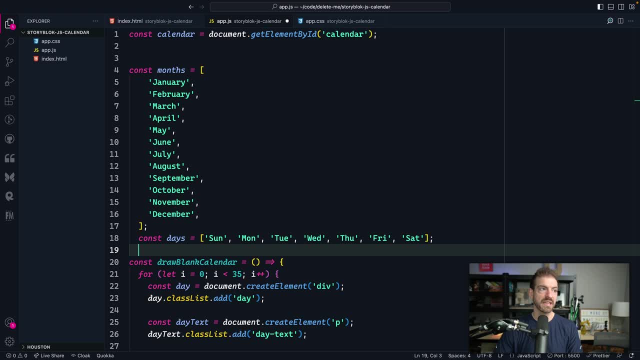 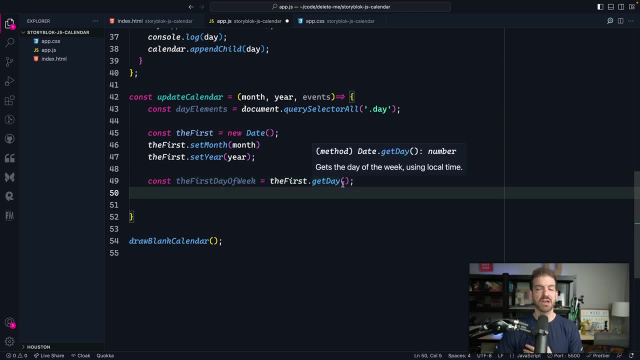 go and get this in the source code, But here's an array of all the months and an array of all the days, And so if we scroll back down, we want to now get a reference to the month name. by calling them months array and passing in the month that we're in, Again, the parameter comes in here. 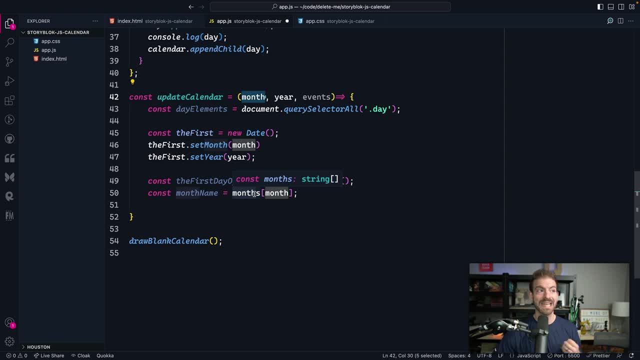 So we say, hey, update the calendar for this month, And then we go and get the text for that, And then we can create a piece of text called month with year, And this is going to be a combined year, and then month, I guess, year and month. Now this is using the template literal. 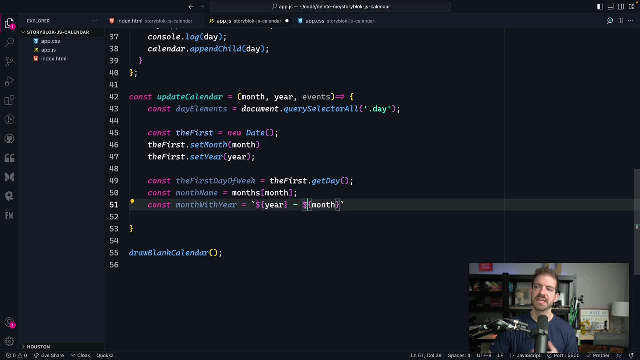 syntax for string. So this is a way to concatenate variables inside of strings. So use the back ticks and then use the dollar sign and brackets to be able to use the actual variables inside of that. Now one of the last things we want is the days in month, So we want to know how many days. 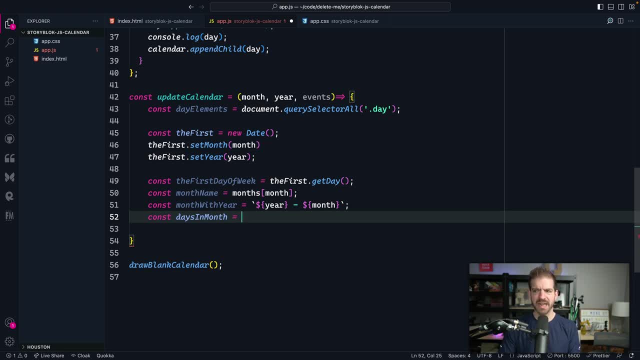 are in this month And this was a little bit of a. I guess it's not a hack, but it's something I found out. So if you create a new date with a day of zero, it'll actually so if you create a new. 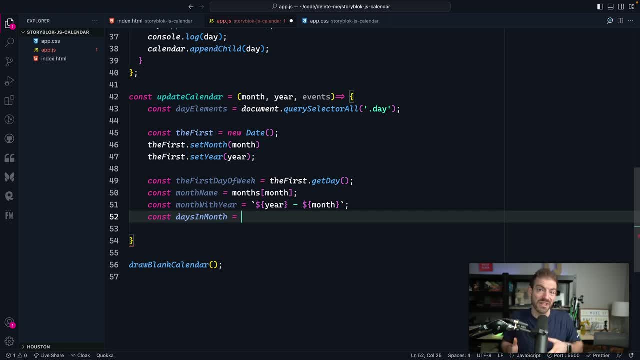 date with a month and a day of zero, it'll actually give you the last day of the previous month. So if you create a new date with a month and a day of zero, it'll actually give you the month that makes sense. So we'll create a new date with year. we'll increment it to next month. 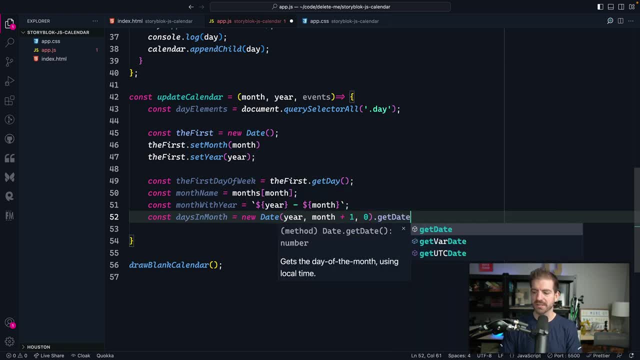 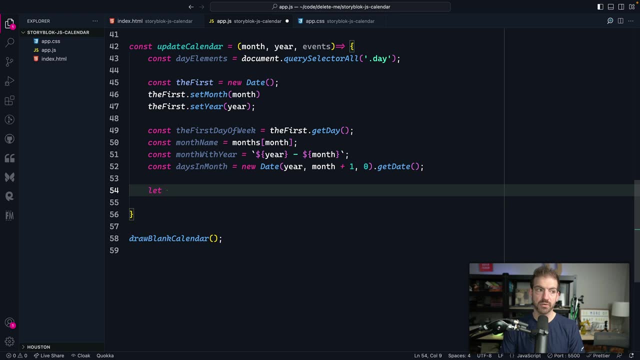 but with a day of zero, which will give us the last day of this month, and then we'll call get date, So that's how many days are in this month. So let's start a for loop And we'll start with a day counter And we'll start this at one. actually, we may not, we may not even need the. 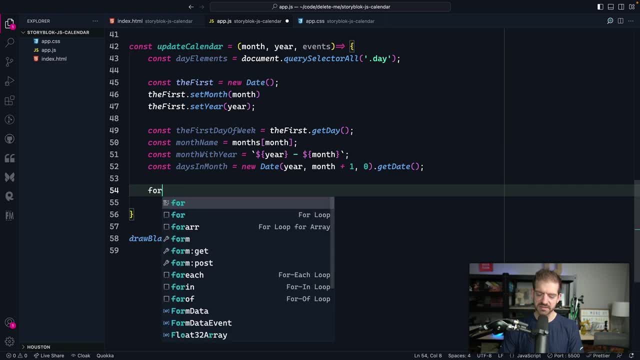 day counter. I think we can actually get rid of this and just use our I. So let's actually write our for loop. So we'll say: for let I equals starts at zero. it's going to be less than day elements, dot length. So we're iterating through each one of those elements And then we're doing I plus plus. 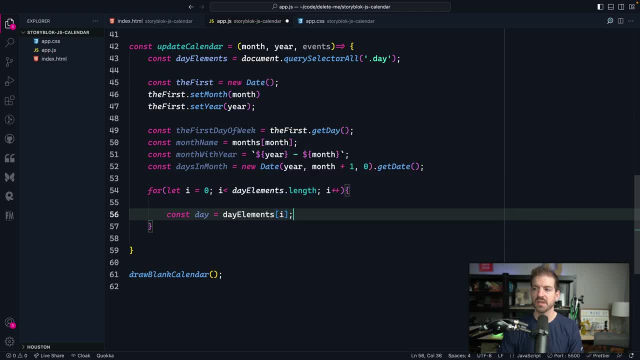 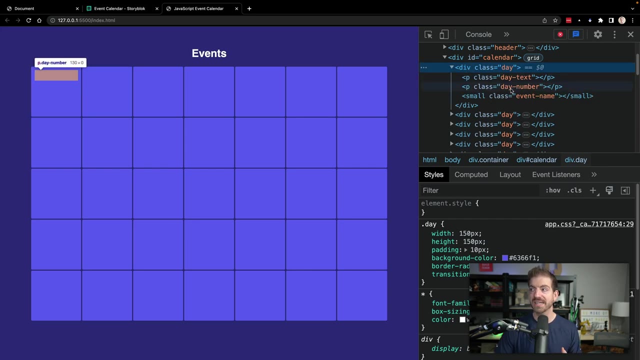 we can get a reference to that day from the day elements array And then with the index of I, and then inside of each of these elements- remember, they have their own property or they have their own elements inside. So they have day text, day number and event name. So we can get a. 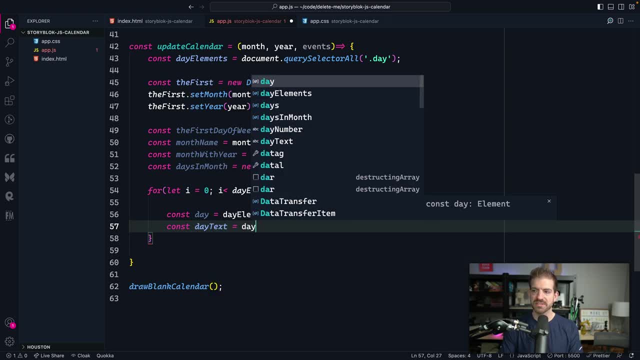 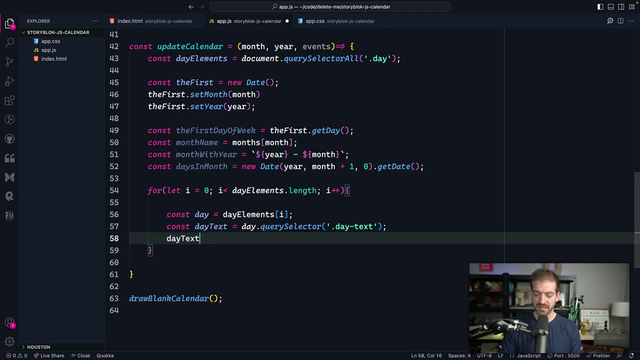 reference to those. we can say that the day text is going to be our day, And then we can call query selector on it And we're looking for something with the class of day text. So just a way to get a reference to the text element that's inside of the day, And then we can take our day text. 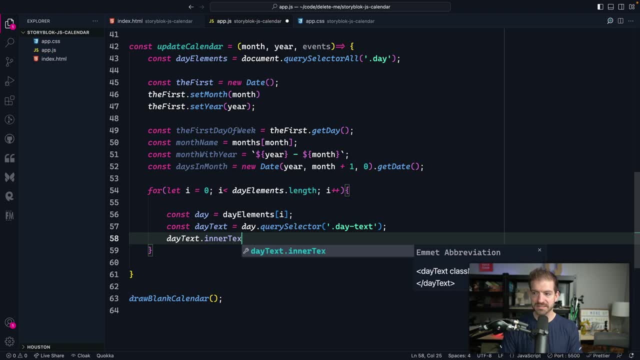 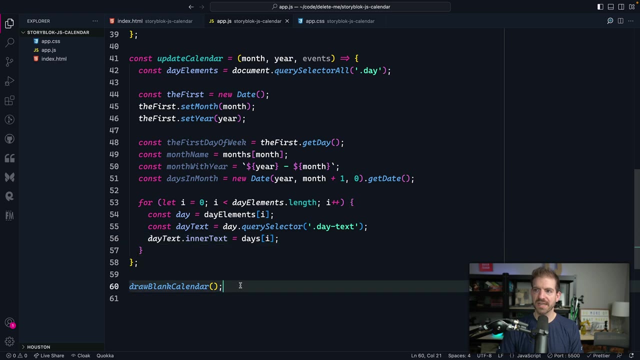 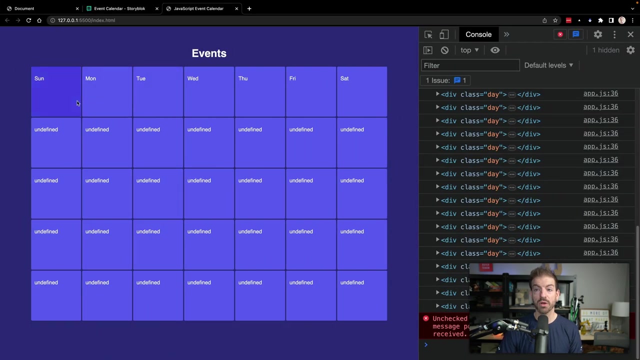 And we can set the inner text property inner text. And we can set this to days of I, mod seven. So let's actually stick with days of I. So let's go ahead and call this function So we can start to test this out. So let's call update calendar And hopefully, what we'll see? well, we start to see. 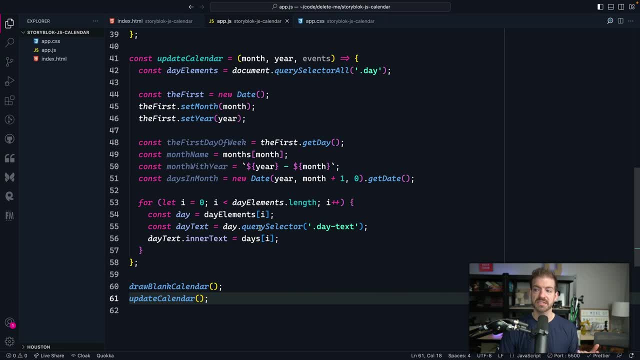 that the first week has the days correctly, but it's not after, And this is because we're going to need to update the day text. So let's go ahead and do that. So let's go ahead and do that. So we are incrementing I above the length of the array, So we want to wrap this down and mod it by seven. 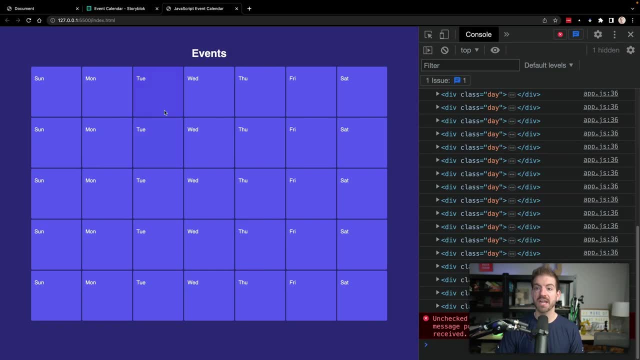 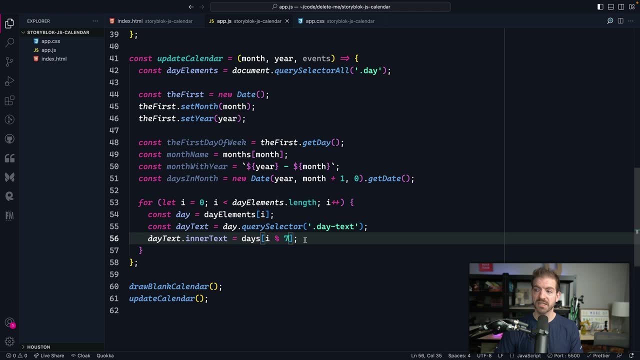 which means if it becomes eight, it will round it back down to zero. So now you can see we have our Sunday, Monday, Tuesday, Wednesday, Thursday, Friday, Saturday, and that is displaying correctly, which is great. Now next up is we can get a reference to the day number. So we also want to. 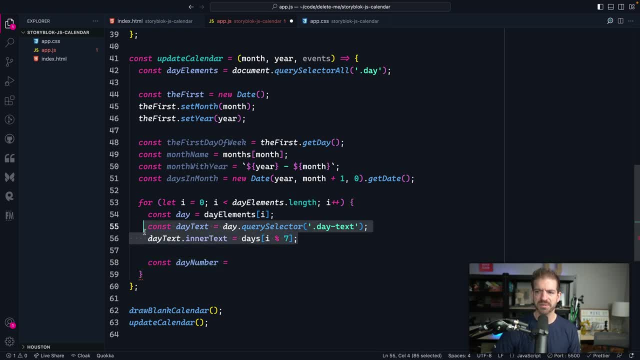 update the number of the day. Also, you could refactor this to put the day text in here, which would probably make sense. Let's go ahead and do that, So it should probably make sense. Let's go ahead and do that, So it should probably make sense. Let's go ahead and do that, So it should. 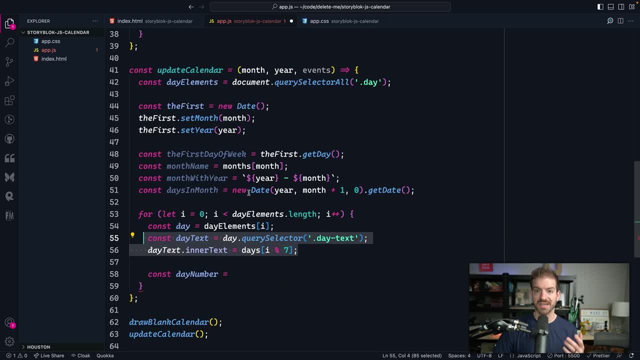 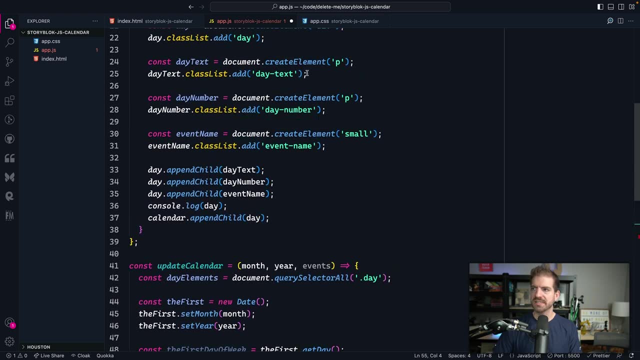 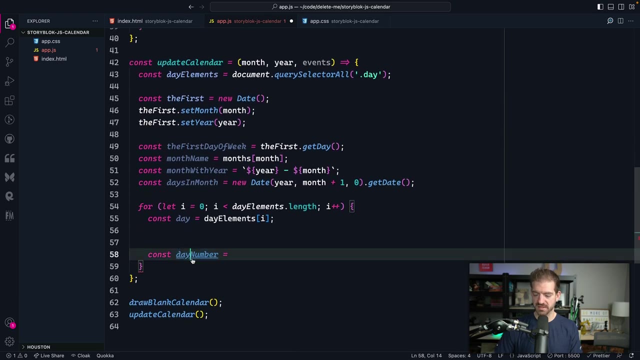 actually work when we draw the blank calendar, because those day names are not going to change. So let's, let's actually take this up here, And when we do the day name, let's just do this, And that should work as well. So let's comment this out and just make sure that still. 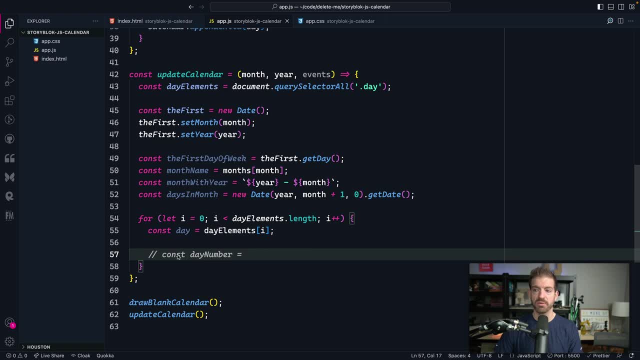 looks good. So Sunday through Saturday for each week- Cool, That way we're only doing that part once. But now we want to get the day number So we can again query selector from our day, And we want to get a reference to the day number. That's a. 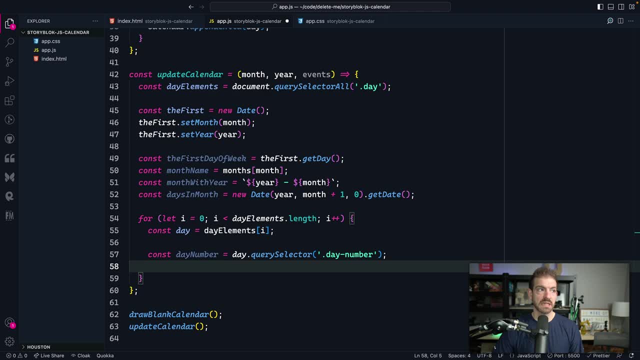 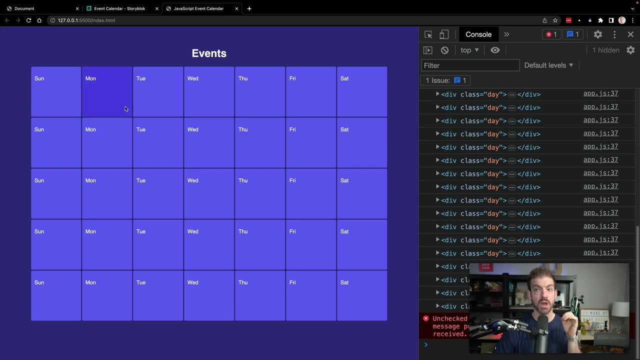 text element that we want to update. So we want to make sure if we're going to add in a number, we don't want to add in numbers that are not in this month. So we only want to add the number text if we're actually 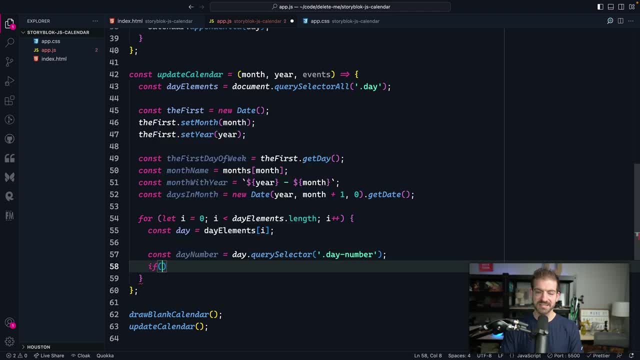 if it's an actual day in this month. So we can have an if condition to say if I is greater than or equal to the first first day of week. so remember, we got the first day day of week up there, So we want to make sure we're greater than or equal to that And I is. 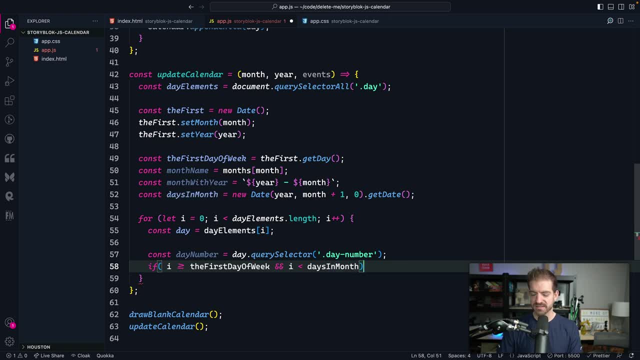 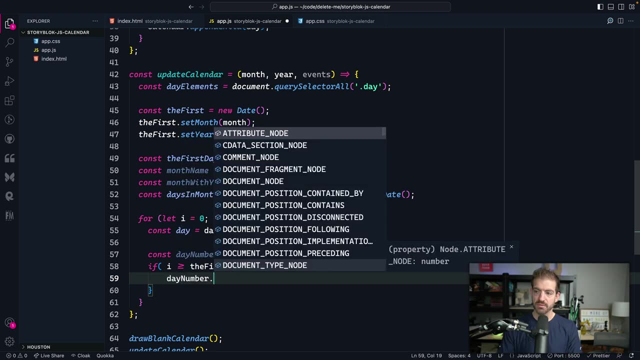 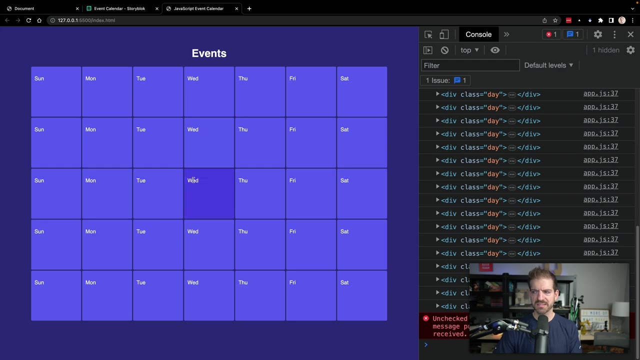 still less than the days in month. So those are two conditions to make sure that are met. So then we can take our day number and we can set the inner text property to I So we can go and look at what this is showing. And it's not showing anything. And I realized that we didn't actually 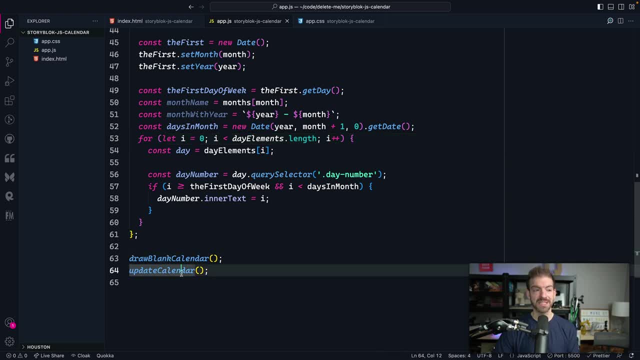 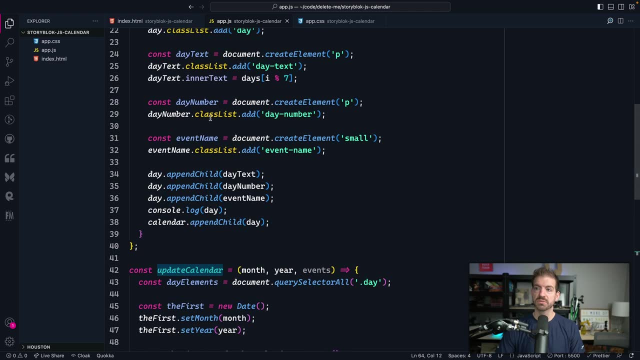 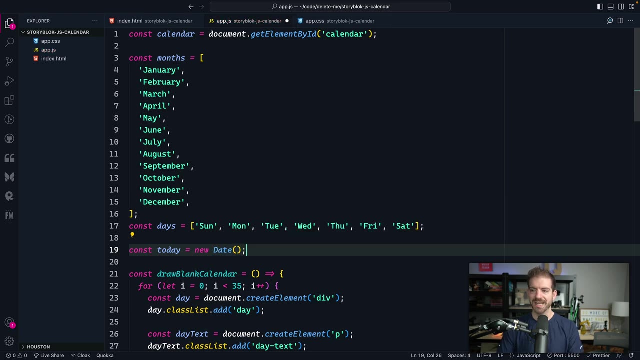 call the blank calendar or, excuse me, the update calendar with the month and the year that we want to be working with. So now it has no idea. So what we'll do is we'll start with creating a variable at the top. we'll call a new date called today, So we'll create the new date And then we'll get. 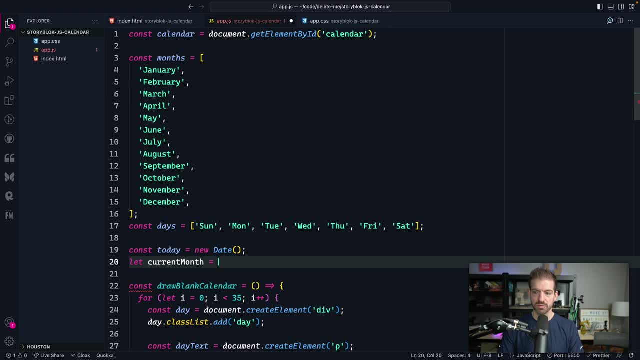 the month and the year. So we'll say current month equals and this will be from today. we'll call get month And then for the current month we'll call get month And then for the current month we'll call get month And then for: 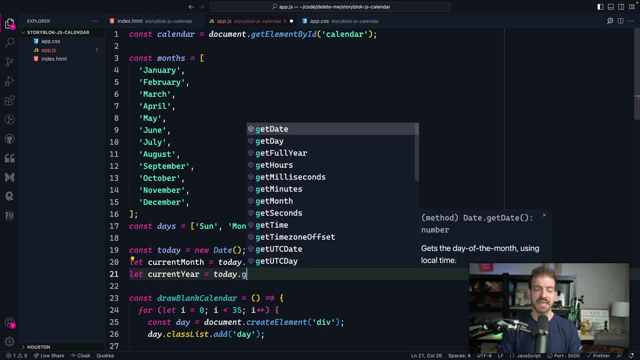 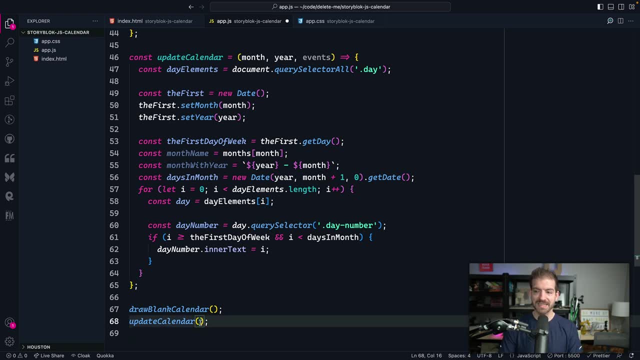 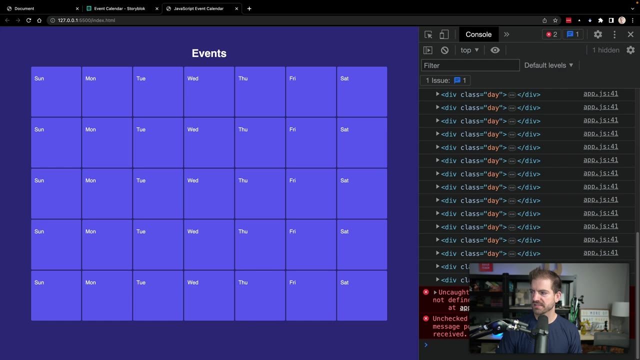 day, our current year. we'll do today dot get full year. And then when we call the update calendar originally, we want to pass in the month and year. Alright, let's see if we get something. Now, let's see, month is not defined. That's because these are current month and year, So current month and 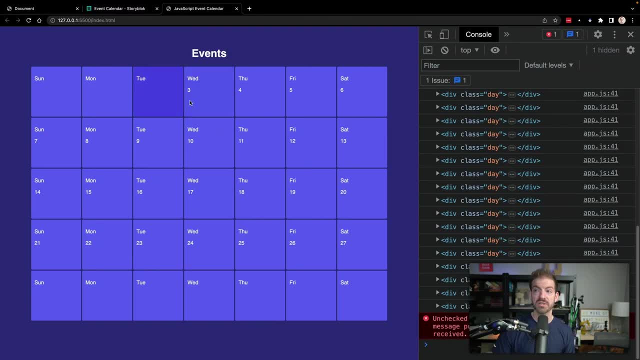 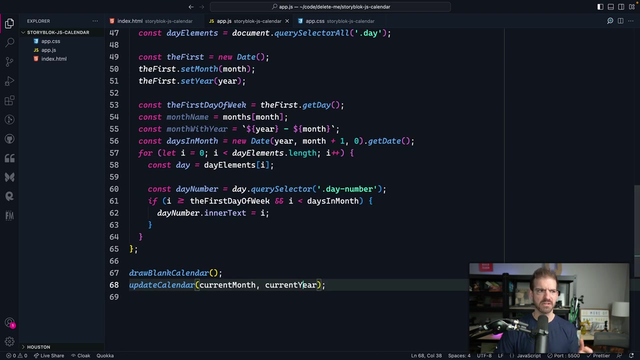 current year. Alright, so now we actually see the numbers coming through And it looks a little odd because it's starting at three and it's going to 27.. And this is actually where we need that day counter that I mentioned earlier. So I thought we could get rid of it And maybe we could do. 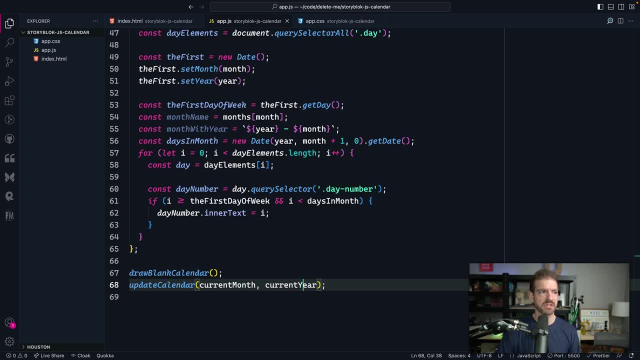 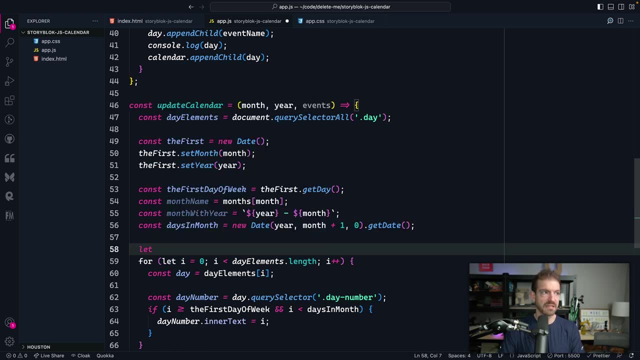 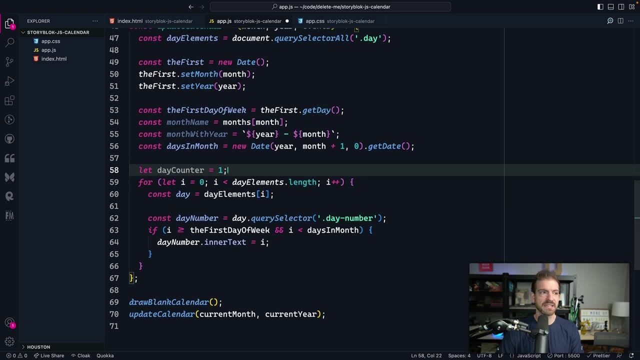 something interesting, how to put this together in a different way, But I say we just go ahead and add this variable. So what I mean is we are before this for loop, we're going to create a day counter and we're going to start it at one, And then we're going to increment this every time we 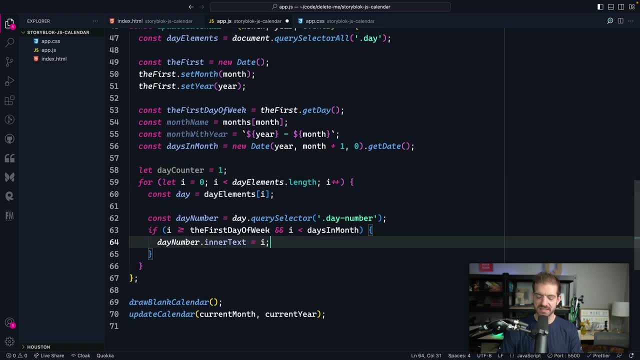 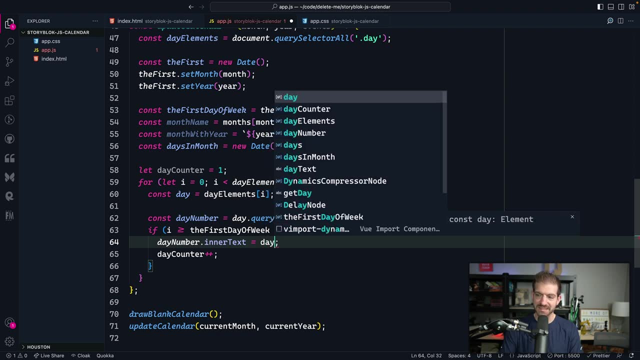 find a legitimate day, so one that we care about. So that's going to be inside of here. we're going to call day counter plus, plus, And then we want to set the inner text in here to the day counter. So this way we're 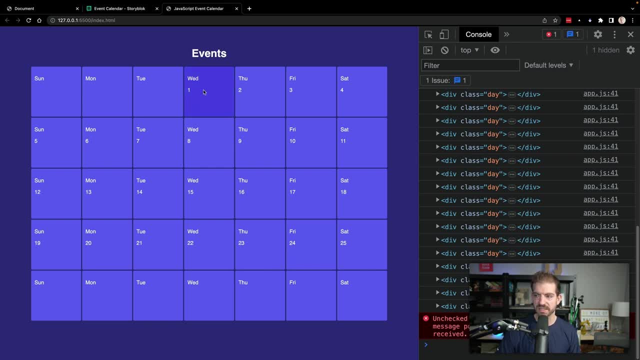 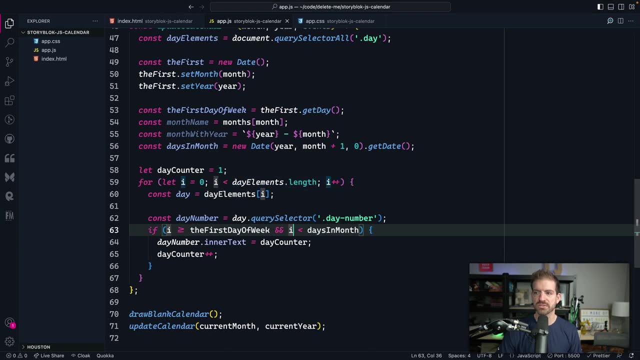 separating out, iterating through each item from the actual days that get displayed. So you can see we go: we start at one, which is great, we then end at 25, which is a little short. So we want to double check our conditions here. 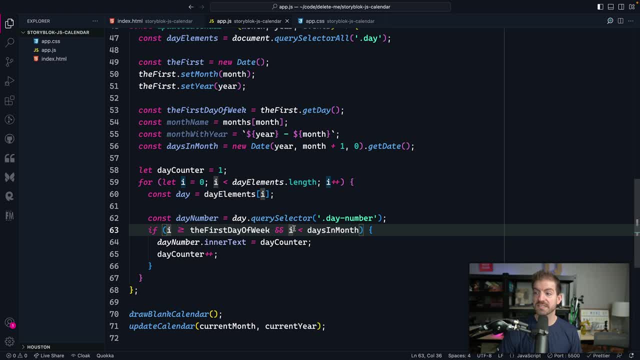 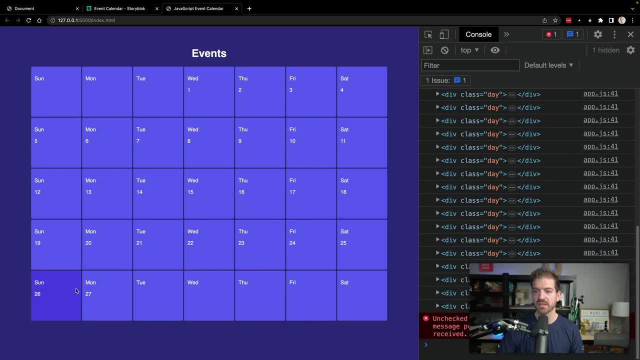 So I think what we want is inside of our condition. we want to check the day counter. So as long as the day counter is less than the total days in the month, we should get almost all the way up. But one more thing: we want this to be: 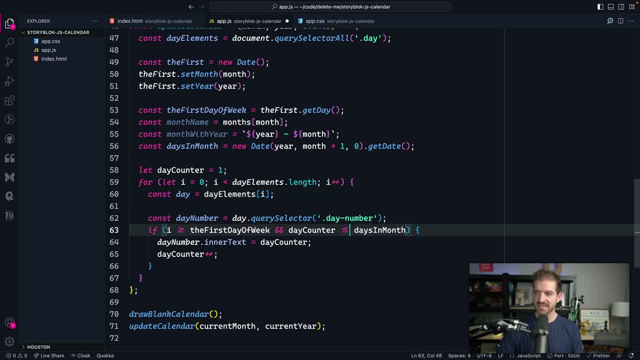 less than or equal to. So in this condition we'll check: less than or equal to the days in the month, and now we should have for February. we have one through 28.. So those days are coming through, which is exactly what we want. Now, when we get into actually updating the months, the dates will 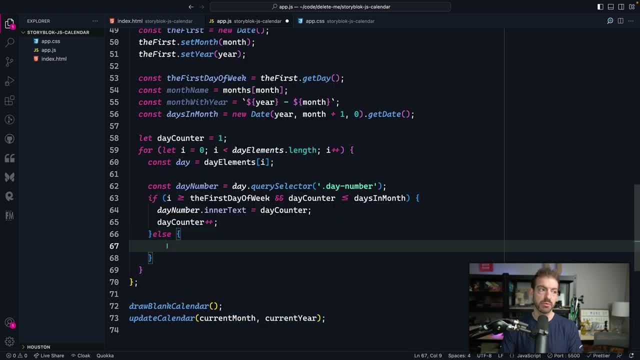 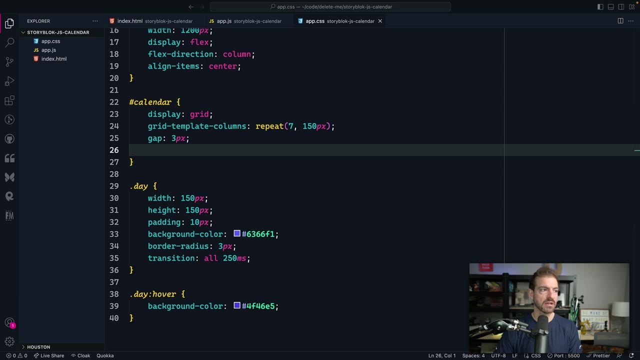 change. so we kind of want to reset if it's not a day in this month. we want to reset the inner text of day number. so inner text to be nothing. we want to get rid of that, all right. so this should be kind of the basics of our calendar. now we can go into our css and we can style the day number a little bit. 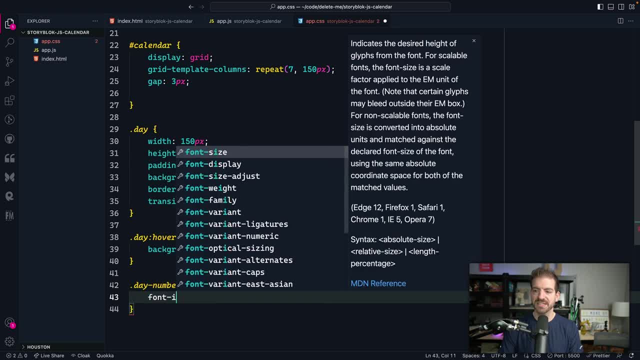 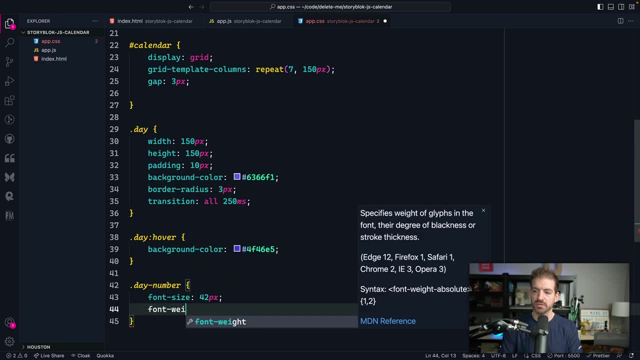 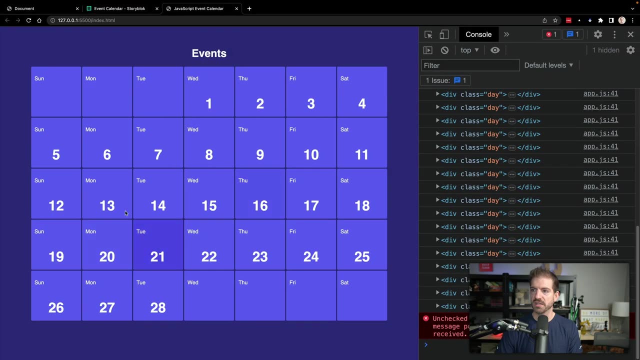 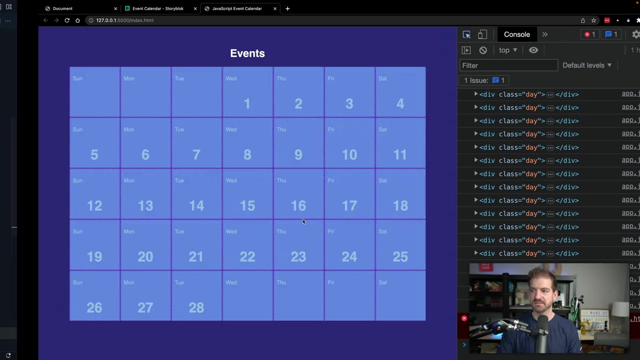 be a little bigger, basically. so we'll say day number, say font size is 42 pixels, we can say the font weight is bold, we'll text align center, all right, and that should be a little bit bigger. now. the one thing that is interesting is this is taking up a lot of space, so we can set the margin. 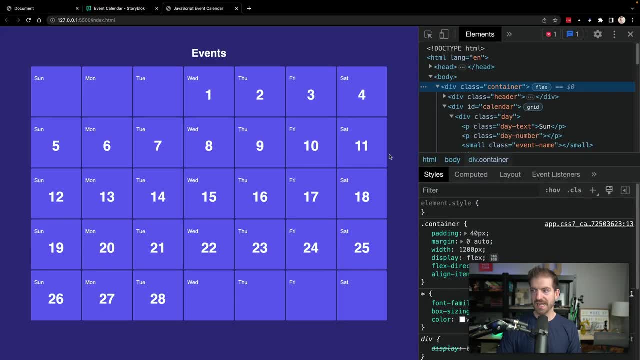 to be zero, and that actually looks pretty good in there. there was another thing i was going to do with: aligning this using a fancy css grid property, but i think that isn't necessary in this case, because it's just doing that kind of takes care of it. so this is working for us. now the next thing we can do: 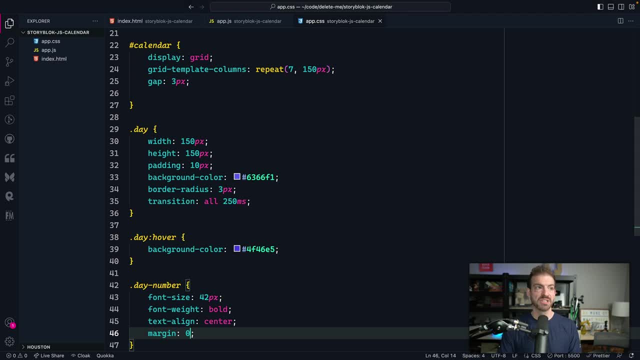 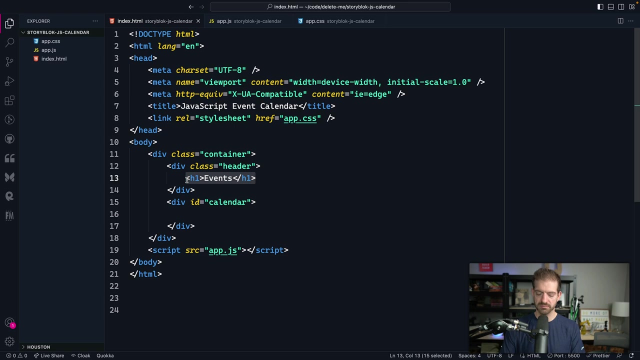 is work on changing months. so to change our months, we're going to add two buttons in our html and i'm going to just copy these in because they're going to be fairly straightforward. but inside of our html file we're going to add into our header two more things. so we still have 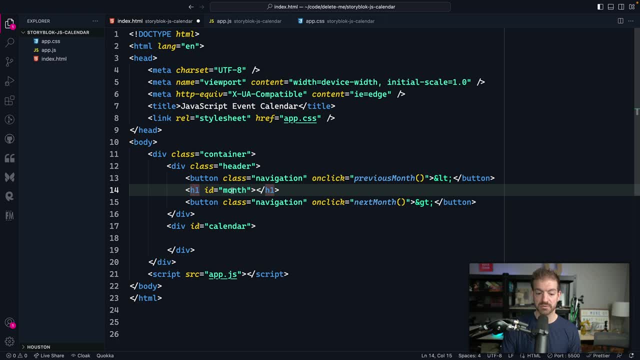 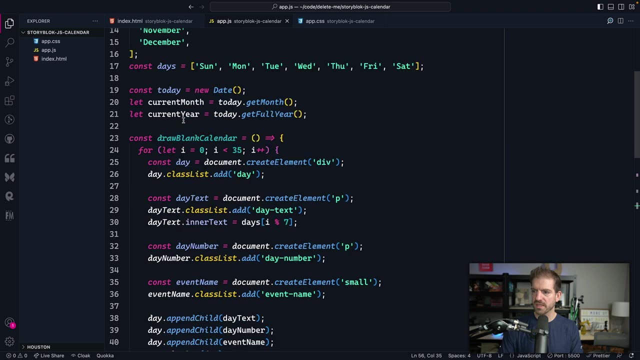 our, our h1, with an id of month which will get updated. i can't remember if we updated that appropriately or not. it looks like we didn't, so let's go and make sure of that. so let's go into our javascript and we query. we aren't querying the month yet, so we get a reference to the month. 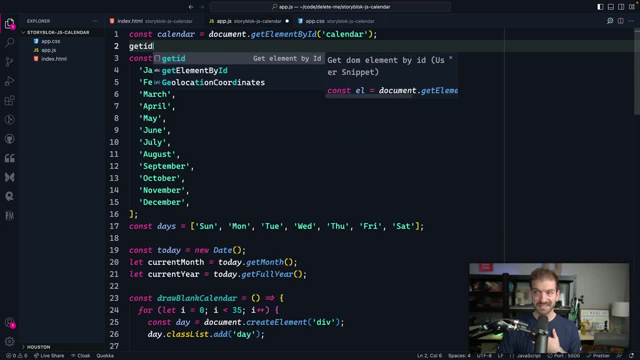 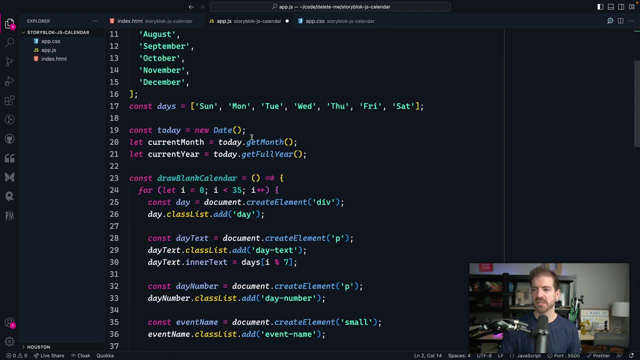 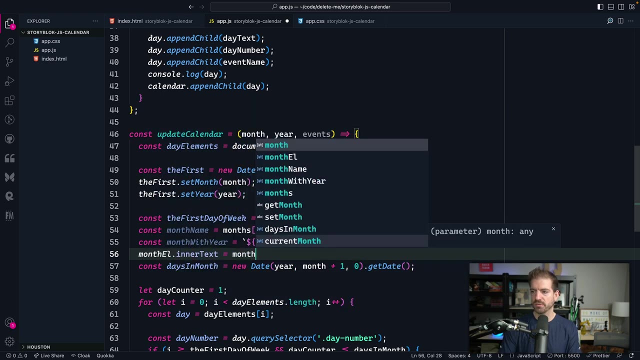 with year, but we don't actually use that, so we can do our get id. this is a snippet again that i have. we can query that month and i'm going to call this month l for month element and then down here we're going to update month l. dot enter text with month, with year. all right, and this should. 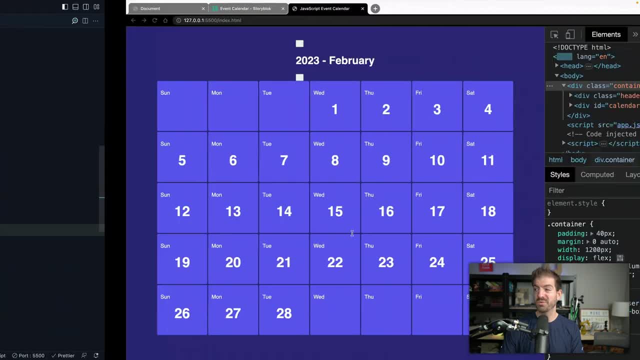 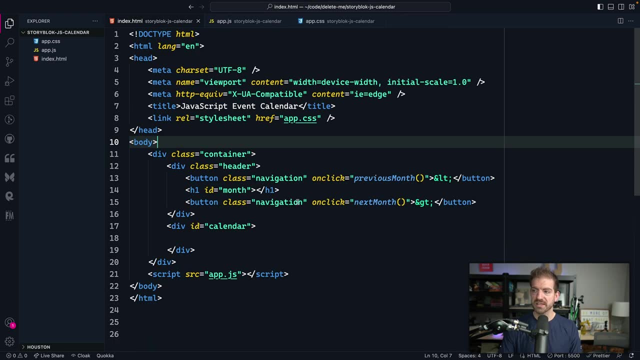 actually be a month name instead of month. so now we should see that displayed 2003 or 2023 for february. that's good. and now let's go back and look at these buttons. so these buttons just have left and right arrows. we are calling functions for previous month and next month, so we need to 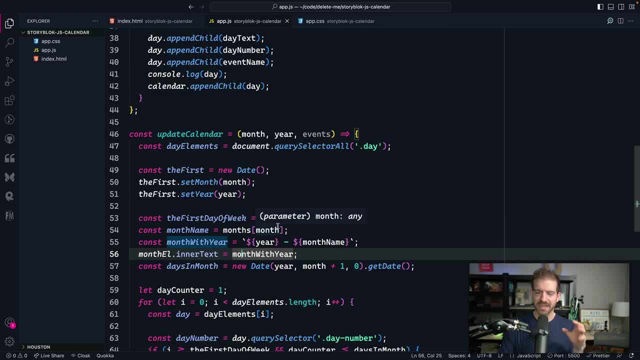 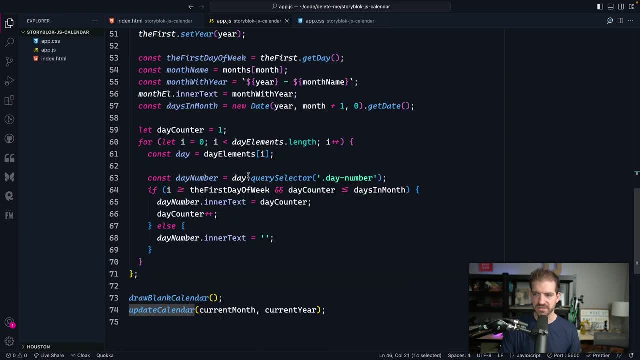 go and create those functions and hopefully you can see that we're going to be able to do that. or maybe take a second and pause and think about how are those buttons going to relate to the update calendar function or how are we going to leverage those. so let's create our functions for 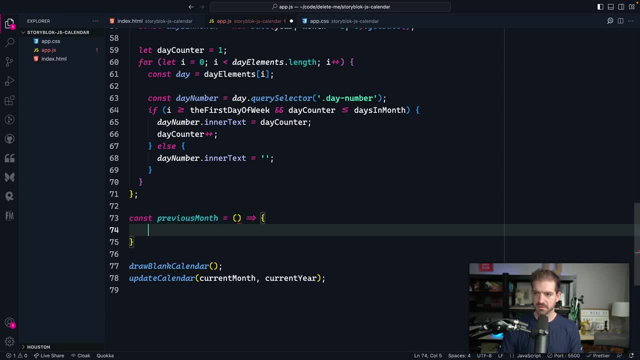 previous month and next month. all right. so what will next month do? well, when we change the month, we need to call update calendar, and then we have these variables for current month and current year, but we need to change this to the next month. so what we can do is increment. 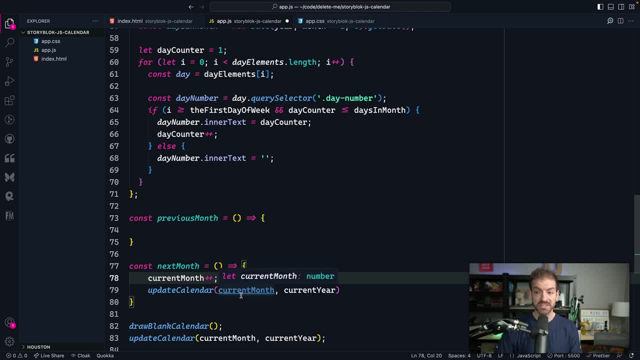 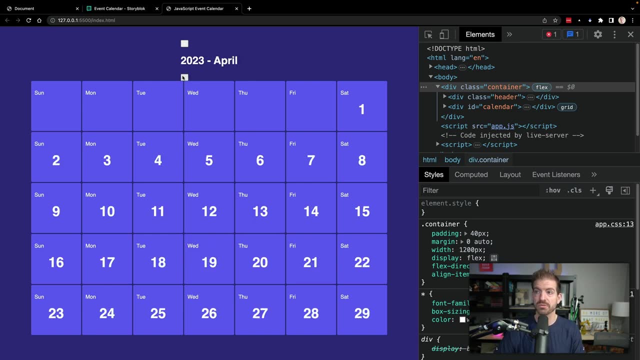 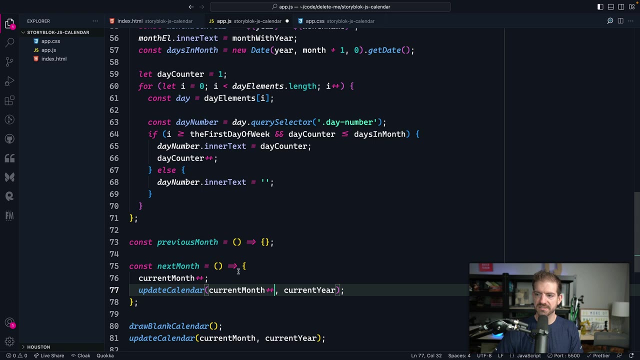 current month first, before then calling this. so this should work, i believe, so let's call. the next one is here, so let's march the days update, which is great. we can go through and through and through, so that looks good. the other thing that we could do is we could just add this plus plus in here, but 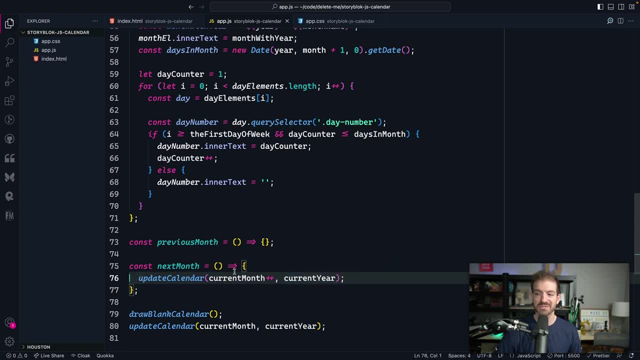 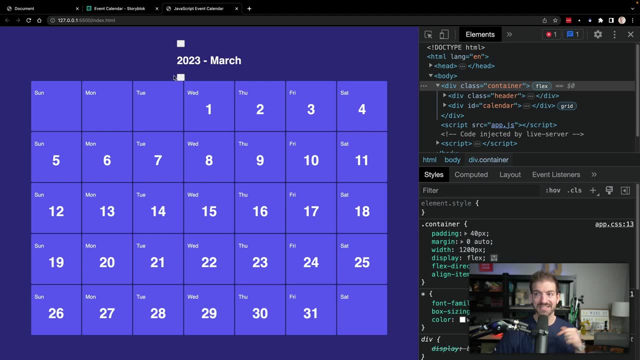 this won't quite have a perfect outcome, because what this will do is actually pass this variable and then, after it, will increment it. so you'll see, one click won't do anything, the second click will. so instead we could prefix this with plus plus, so that it does the plus plus before than incrementing. 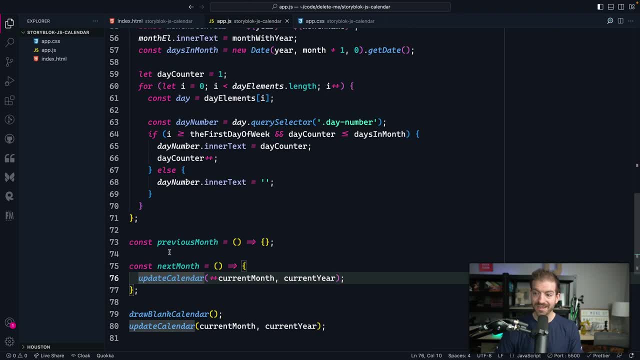 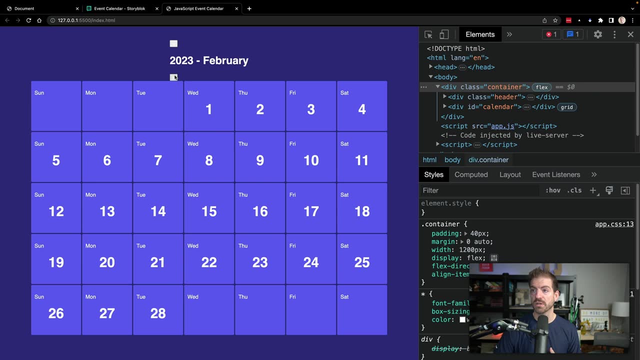 so one click now will do it, which is what we want, and then you can imagine. the opposite of this for previous month is we just do minus, minus. so we want to go the other way. so in this case we can go forward, backwards, backwards, but then we hit a problem of switching years and 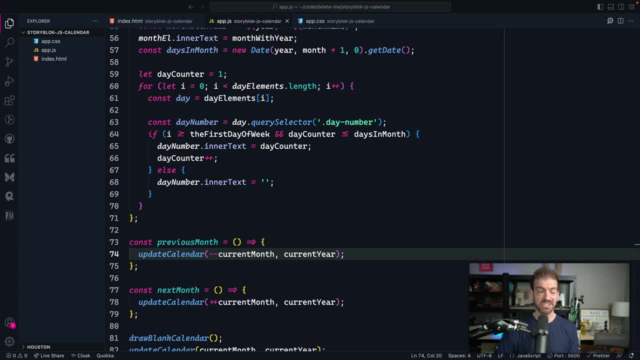 this is where we need to add a little bit of logic in here to handle this. this would be a good challenge for you, a relatively simple one, if you want to pause this and kind of take a guess at how to solve this and then come back and i'll show you how to do it. so for the previous month, the thing 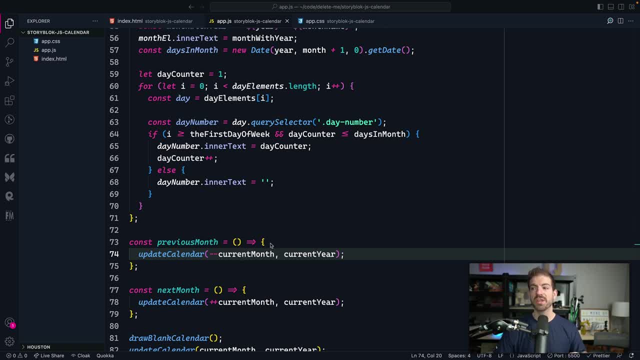 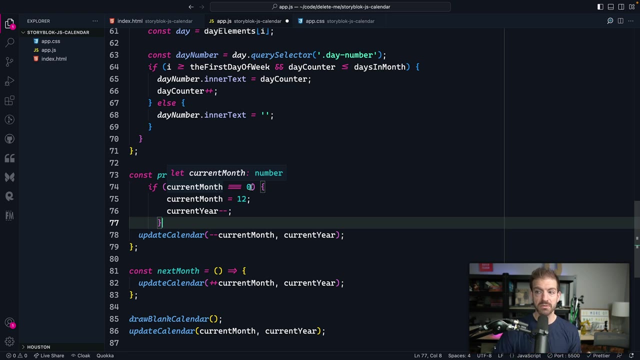 we want to check is if it is a month of zero, we then want to subtract a year as well. so if it's a month of zero and we subtract one, we want to go back to 12 and then set the month to subtract one. so what we can do is we can say that exact same condition if the current month equals zero and we 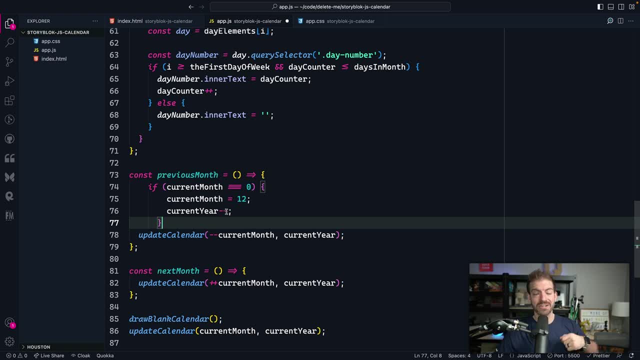 press previous. set the current month to 12. set the current year to subtract from itself and then come in and update. keep this exact same call but then update current month. so current month is zero based indexing. so 12 gets subtracted down to 11, which represents the 12th month, and then similarly with: 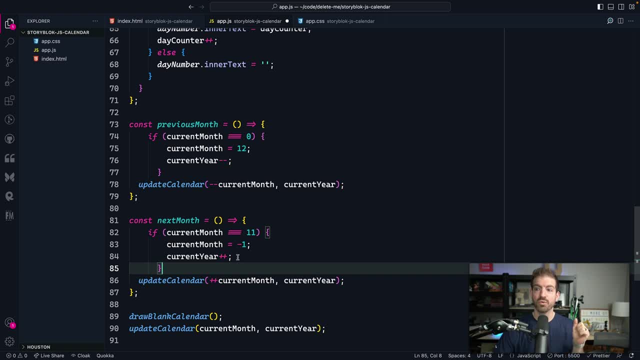 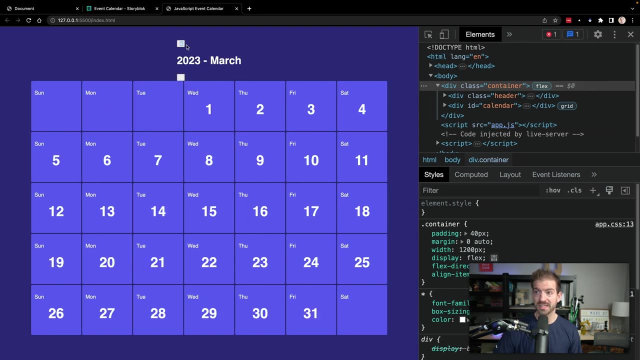 the next month. if it's 11, we will set the current month to negative one. it looks weird, but that means then when we increment it it will come up to zero and then we increment the year. so now we should have this like pretty good looking calendar that is able to iterate through months and years. now notice these things. 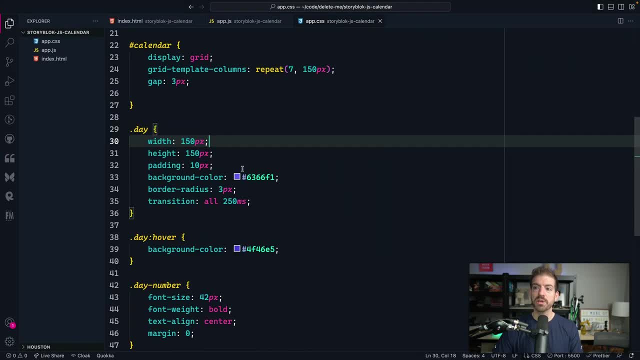 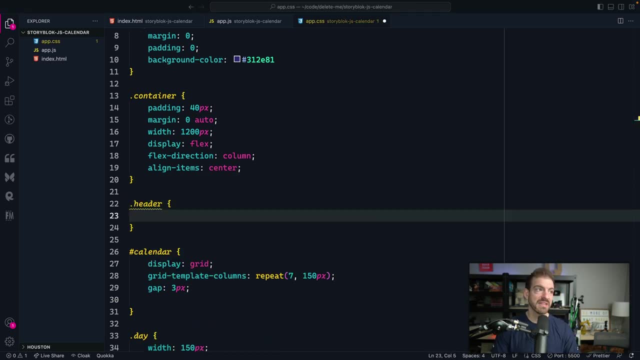 are kind of jumping around. we actually need to add some styling to these, so we put all of those inside of a header class so that we could be able to style them together. so we want these to kind of be in line with each other. we want these arrows to sit next to our text so we can 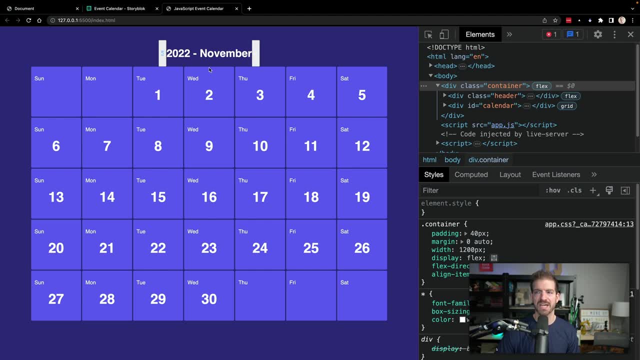 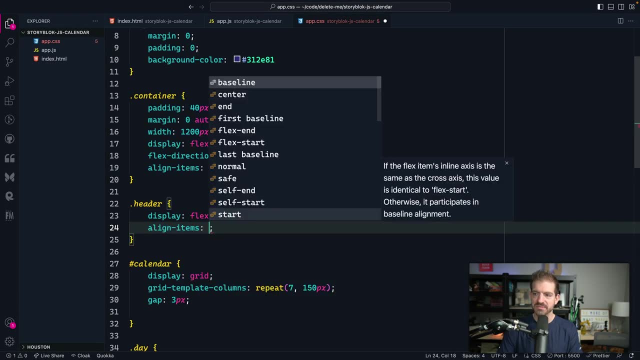 use display of flex for this. we did this earlier, but now you see it sets them side by side, but in this case, instead of having them stretch out or vertically, we can say, align, items is centered, so this is going to align all of these items in these across the main axis vertically. we can also give: 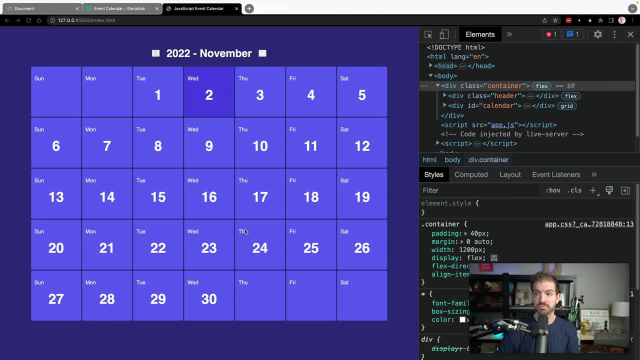 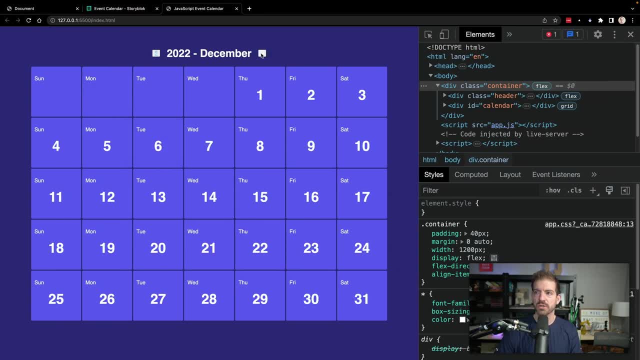 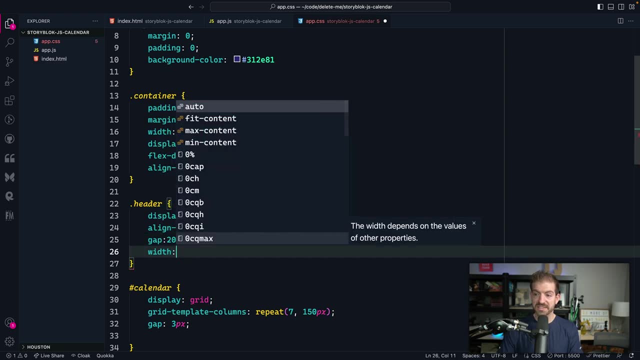 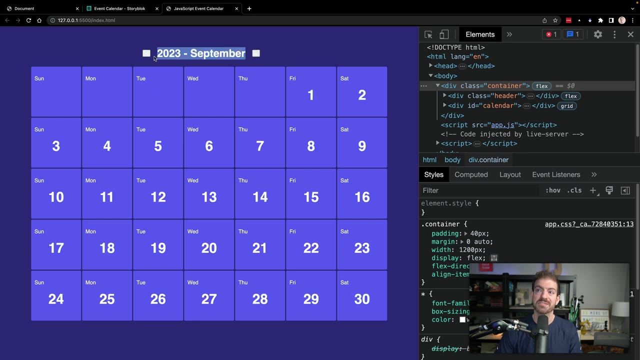 them out a little bit so that looks good. and then one of the things we'll notice is: this is going to kind of shift the width a little bit, which we don't want. so we can set the width specifically to 400 pixels. all right, so we still see this shift. so the thing that we can do is we can spread out. 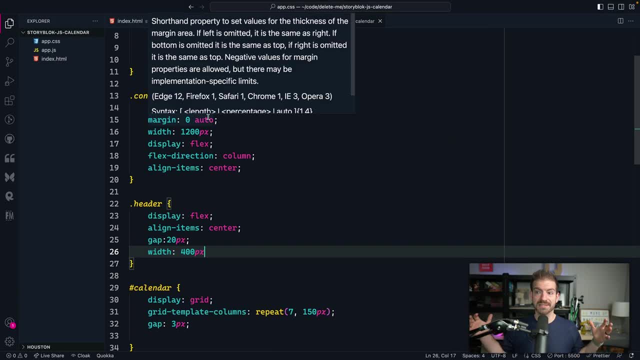 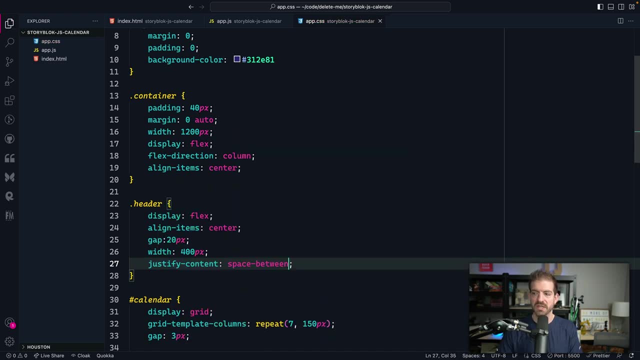 these elements- the buttons and the text- across all the open space that we have. so to do this, we can say: our justify content is space between. this is going to spread those out, take up all the space, and now that text and the button stay in the exact same spot the whole time, which is pretty neat. so there is also a little bit of styling for. 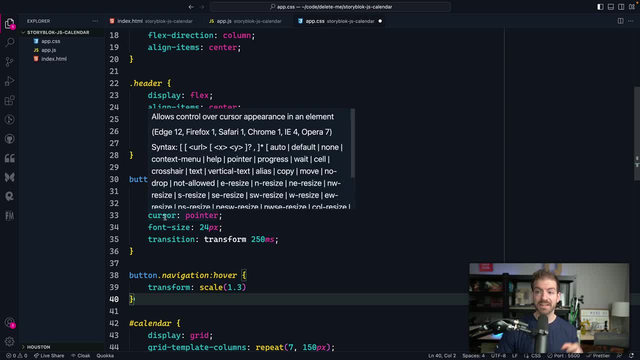 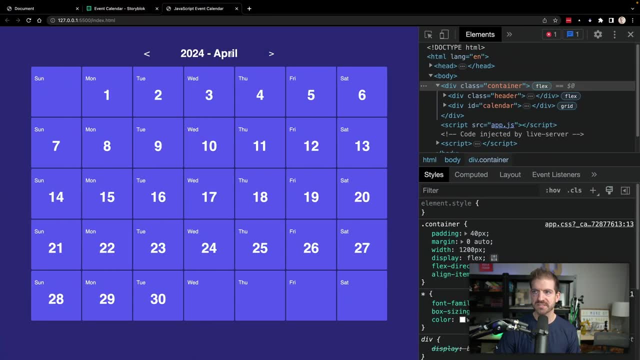 the buttons: just getting rid of the background, getting rid of the border, adding a cursor pointer, font size, a transition, and then to scale them up to make them look a little bigger. so we hover at scales and these buttons work the exact same way. so we have our calendar now, the next thing we want. 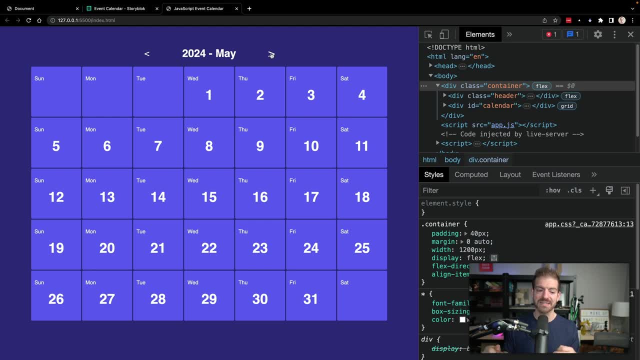 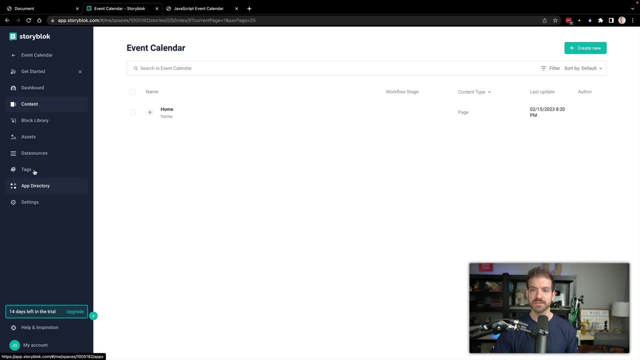 to do is actually connect this to start the calendar. so we're going to go ahead and start the story block so that we can display the events inside of this calendar and it's live data coming all the way from story block. so let's go into our story block here and inside of content we want to 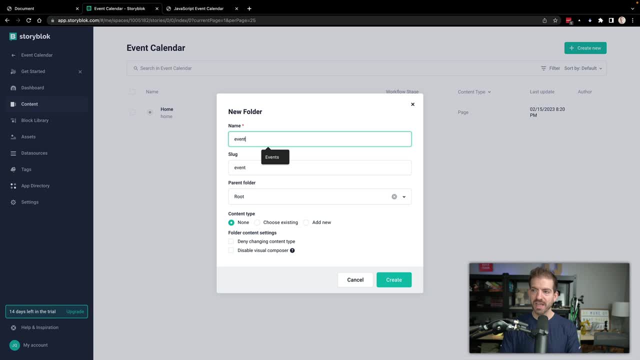 create a new folder. so we want to create a folder for all of our events and story block kind of thinks of content in relation to it being on your website, because that's kind of the point of this is: it's going to be on your website so you'll see things like slug, which is basically the url for. 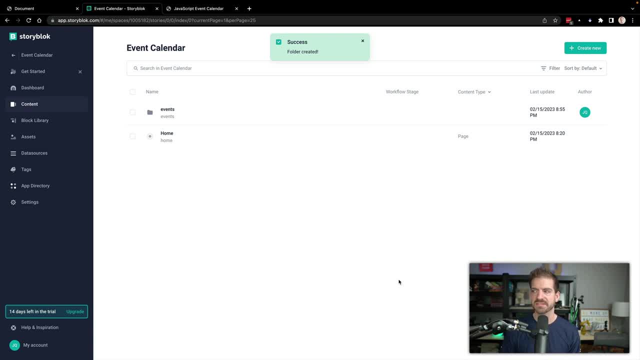 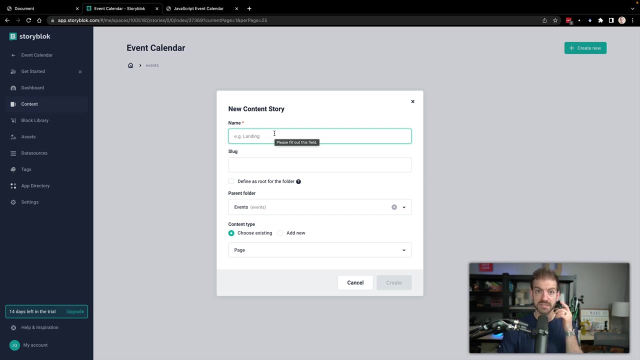 this, and so we're saying all of our stuff is going to be inside of an events folder. now, before we can put events in here, we can say: we're going to create a new story. that's kind of what one of these individual pieces of content are. we're going to create our first, first event, so we'll call this meetup one or 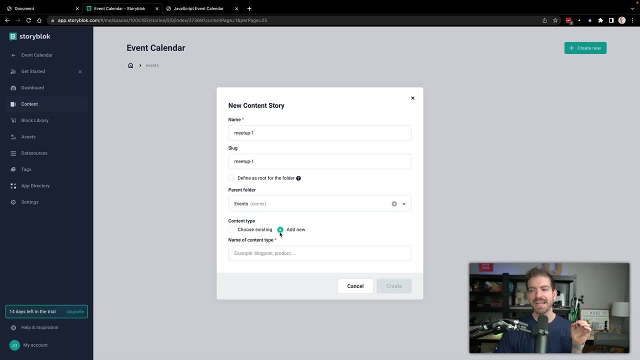 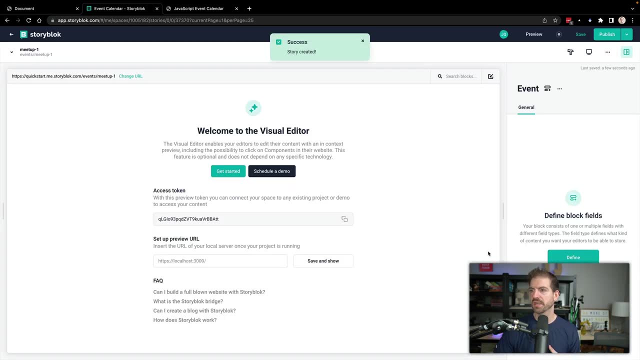 something. this is going in the parents directory and then we want to add a new content type, so the content type of this is going to be a, an event. that's going to be the name of it. so we're going to call it an event. and then we're going to add a new content type, so we're going to call it an event. 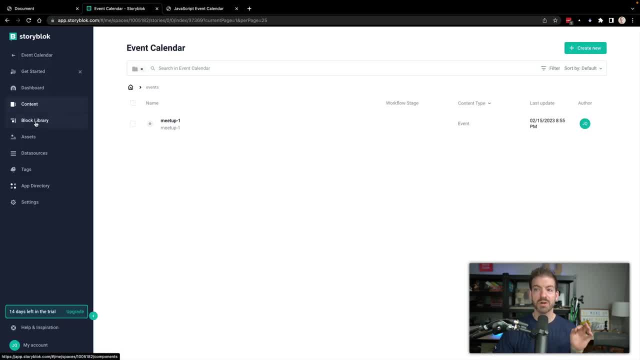 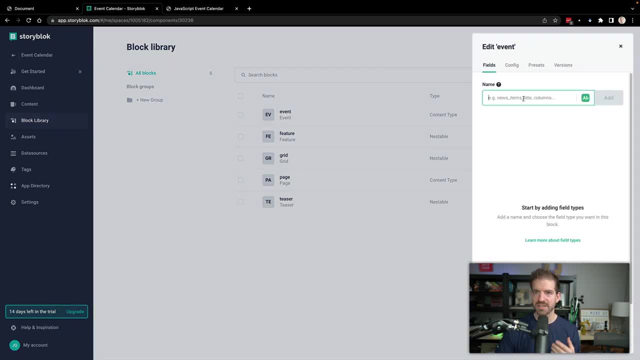 so let's actually go back and go into our block library. this is where we kind of define what the different content types are that we have. so see, there's event here, but it doesn't have any properties associated with it, so we can add a text property. so here's all the different types that. 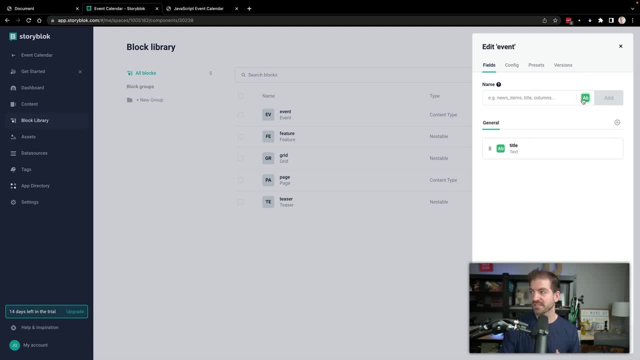 you can add. there's a lot of different things in here. we can add a title of this, we can add a link, if we wanted to, so a link to the actual event, and then, lastly, we can add the time. so we can add a date time in here. so there's our date time. we'll go ahead and add that and 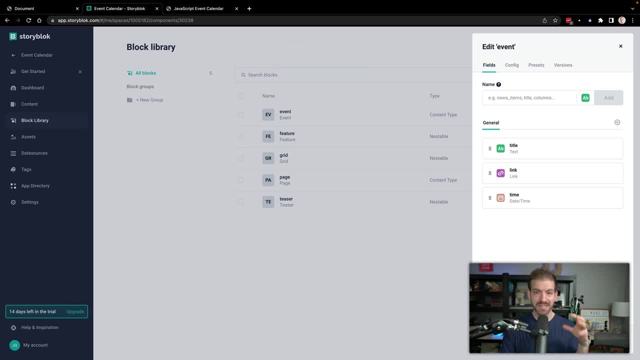 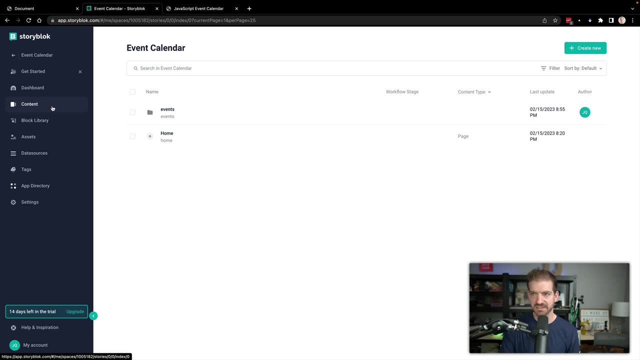 those are the three different properties that we want. so again, creating content inside of story block is very, uh, very, very easy to work with, and then we can pull this data in using just a basic fetch request in our application. so inside of events, we should have one event already, so this: 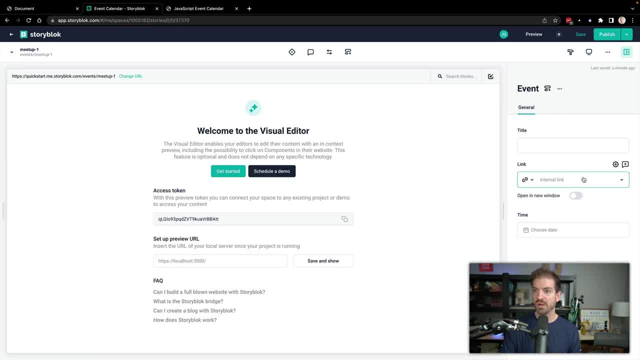 is meetup. one notice: now that we defined what this uh, what events look like, what, what sort of properties they're going to be, and then we can add a date time in here. so we can add a date time in here. so this is meetup. one notice: now that we defined what this uh, what events look like, what sort of 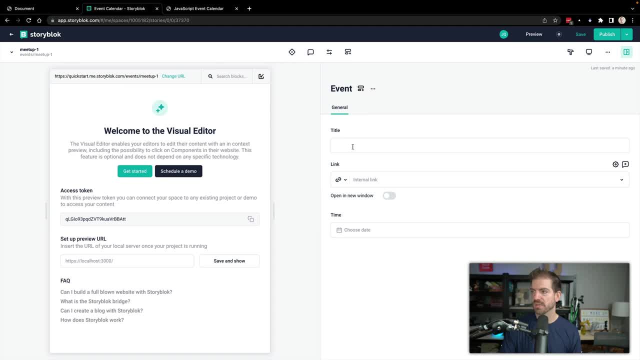 they have that. we have, uh, this over here trying to make this a little bit bigger. so we can call this my first meetup. we can have this be an external link and i'm just going to link to my website for now, and then we can choose a time. so when is this first meetup? well, we can say: this is: 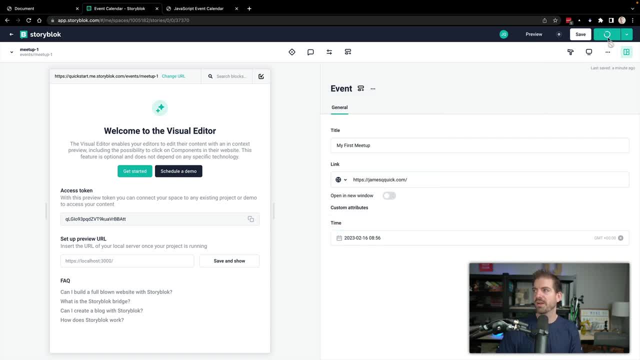 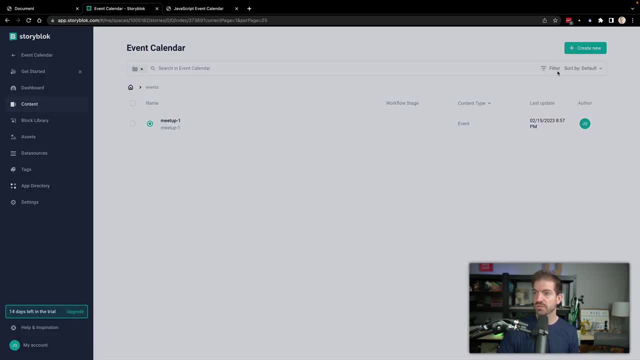 on thursday, the 16th, at a specific time. apply, publish this and that record is out there. now we can go back and we can create another event. so let's create a new story and this will be, uh, wins of the week. this is actually something we do inside of my discord, where we 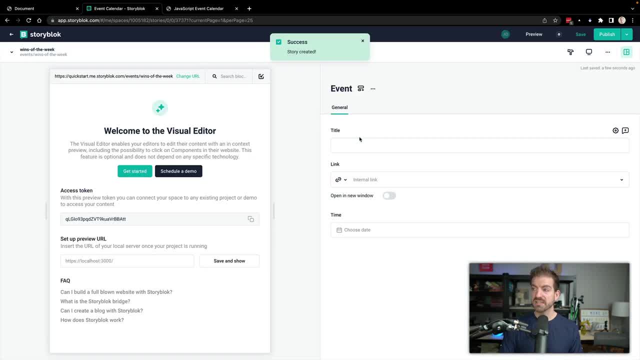 celebrate everybody's wins every week, so we can create a wins of the week. we can call this wins of the week one. we can have this, uh be an external link, so url, to the learn, build, teach website. and then the time of this: they're on fridays and specifically at 9 am central. 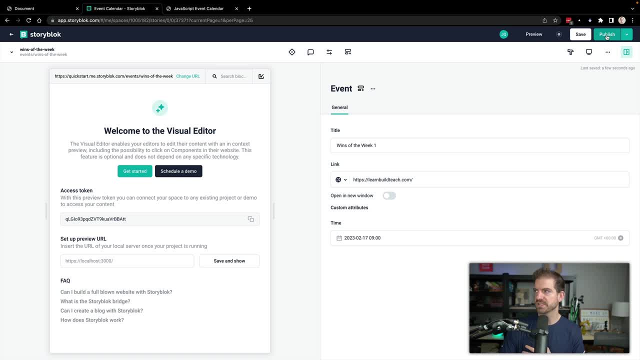 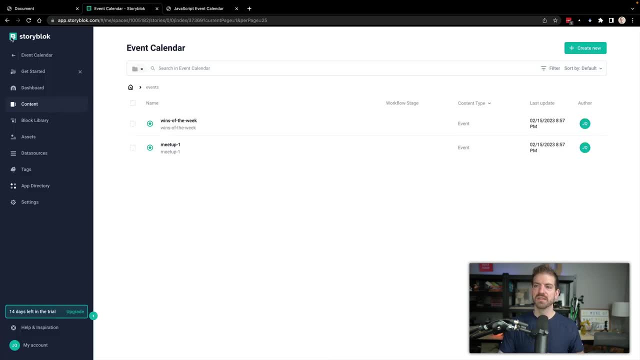 so that's where that's my time zone, that's where these events are. we can go ahead and publish this just to prove out that we have, uh, two events of stuff that we can work with. so going to a meetup and then i've got my wins of the week session coming up, so one of the things 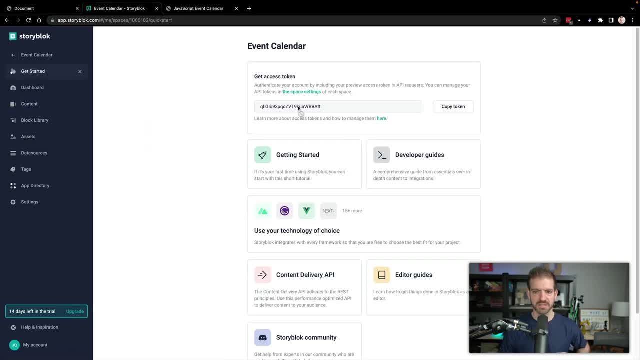 we'll need. i think it's under: uh, getting started is an access token here. so an access token. this is read only: this is what we're going to include in our request to storyblock to be able to get the data that we're looking for and then be able to work with it. so inside of here we'll go back to. 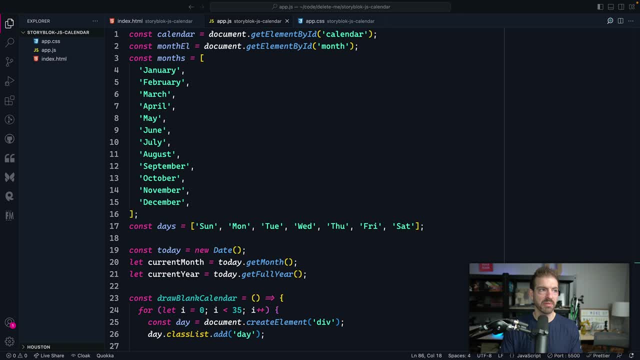 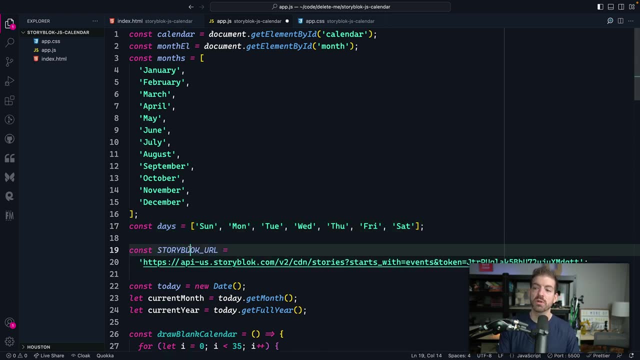 our javascript file and at the top of our file i'm going to paste in a variable for- let's do it right in here- for the storyblock url. now you can- uh, you can- figure out what this url is. it's pretty standard up until kind of this point, and the one thing that's specific in the us is, if your 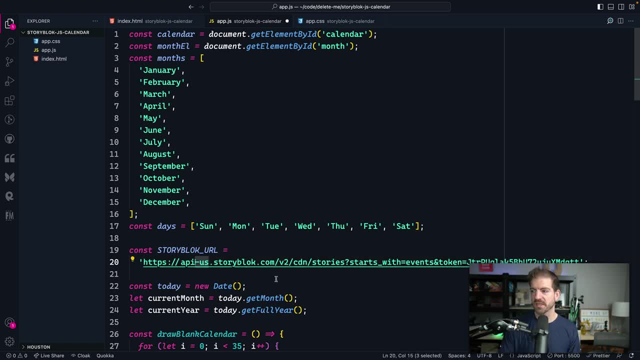 instance, is deployed in the us. you have dash us, otherwise you don't need it, and so we're looking to query stories, and then we're looking for stories that start with events. so this is: they're in the uh, in the events folder, and then we need to paste in our tokens. this is the old token, so just replace. 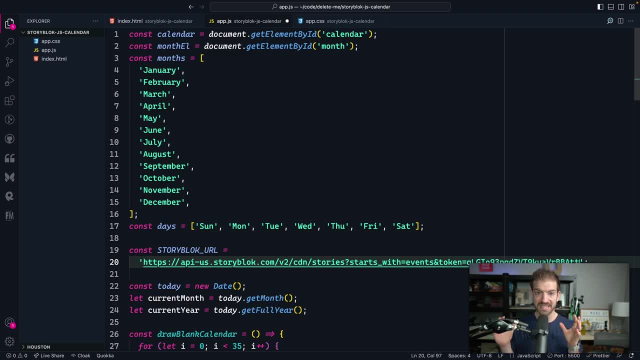 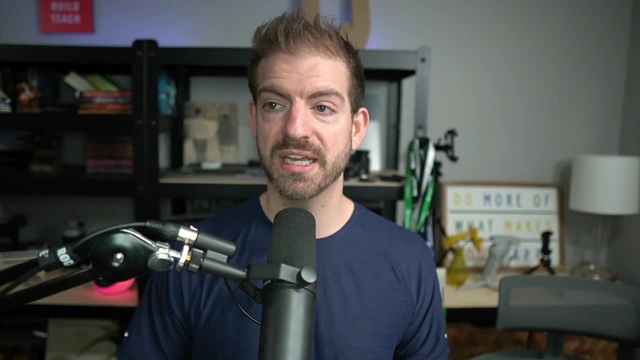 your uh. replace that with your token. that is specific to this space. so this is the url that we're going to make requests to now. it's worth noting that storyblock has uh npm packages for different libraries and frameworks, so if you're using react or svelte, 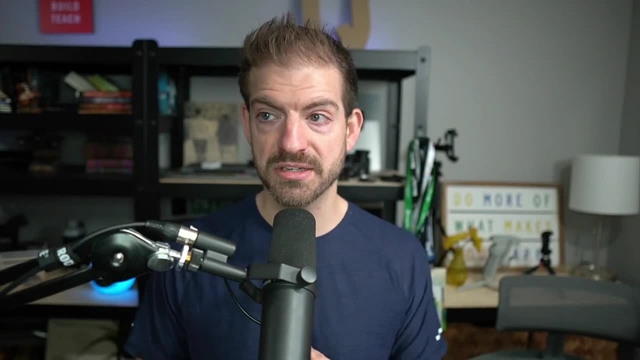 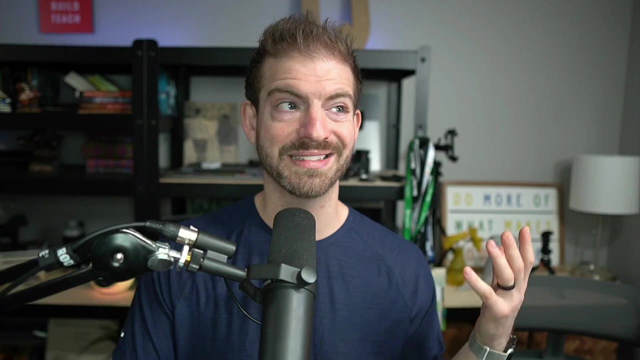 kit or something like that. they have uh sdks to make this easier for you. this is just a fun exercise in my mind to do this with vanilla javascript, so without the help of sdks, to show you that it's still really, really easy. so let's go down and we're going to create a new function. 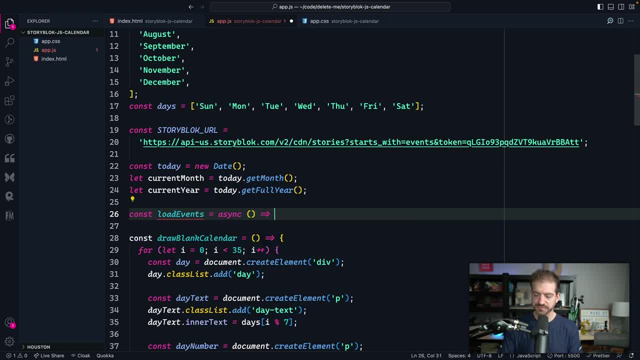 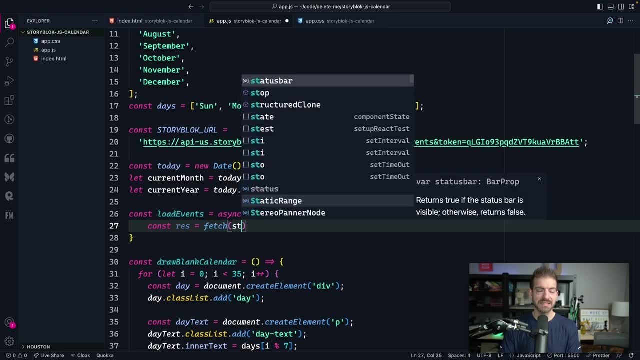 for load events. so this is going to be an async function and we're going to make a fetch request inside of here. so we're going to call this function and we're going to call this function, call fetch and we're going to pass in the story block url. this is returning to us a promise which 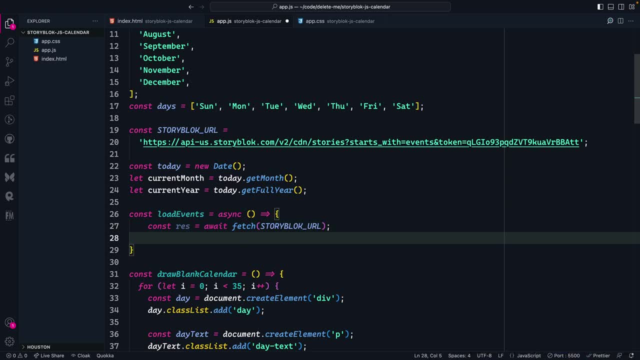 means we need to await that to get the response and then from there we're going to get back data by taking uh the response and then converting that to json. so we want to get back the json response and then we can log out data. just to see what this looks like. 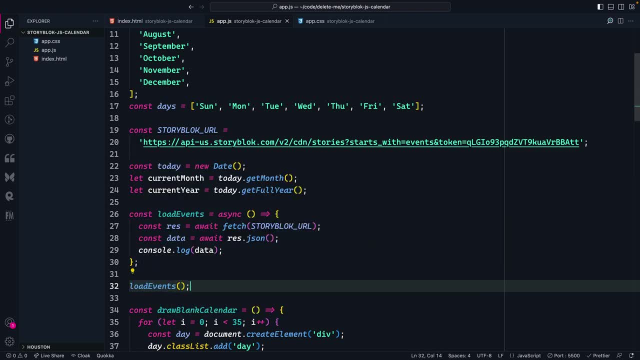 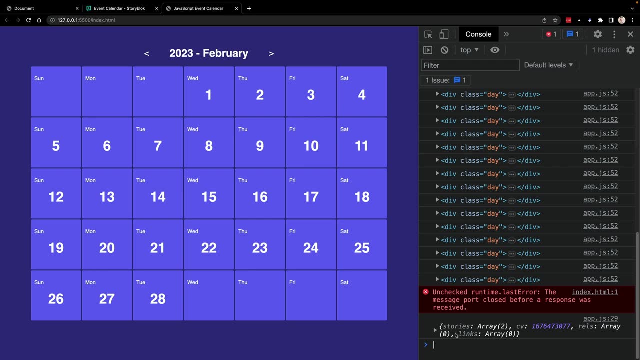 so the last thing we need to do is call the load events function at the same time. so we'll call load events, we'll go into the console and we should see that we have an object come back with a property called stories, and inside of stories there's our 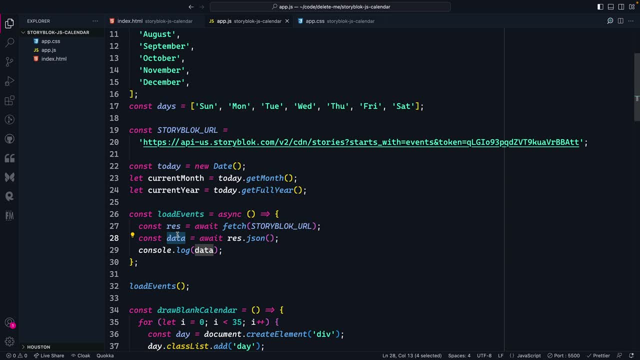 two pieces of content that we care about. so with this, one thing we can do to get access to that stories variable is just destructure it directly. so this is the equivalent of doing this. so if we got data and then we said stories equal to json, we're going to call the load events function and 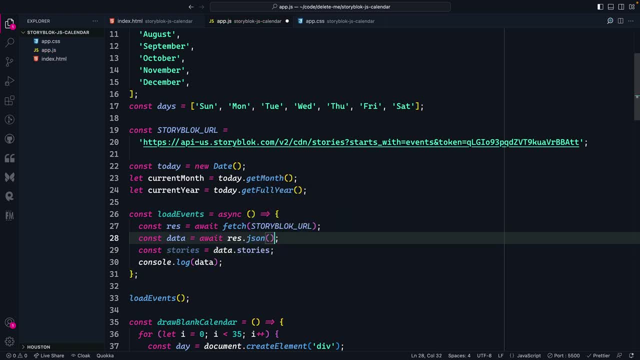 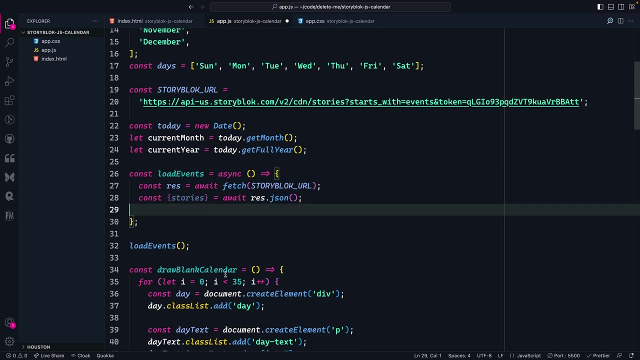 that would be the exact same thing as uh just doing this, and i just think this is a little bit simpler. so we'll get access, uh, to these stories, and then we want to. we need to have some way to associate as we go through each of these stories. how do we know if it matches the day that we're? 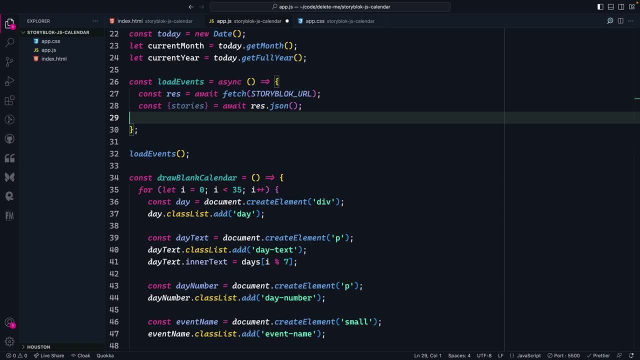 looking at when we create our calendar for that month or when we update our calendar for that month. so this may be a little bit more complicated than what we're looking at right now, but we're going to do this in a way that's a little bit more complicated than what we're looking at right now. 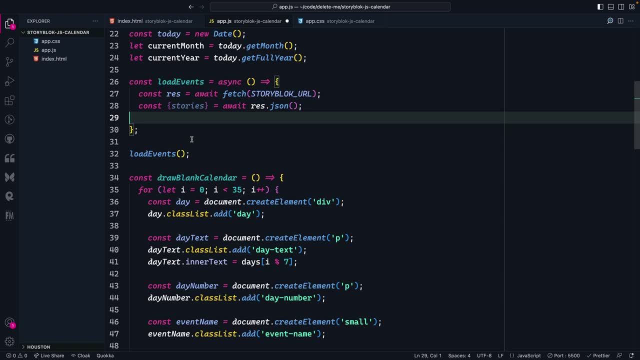 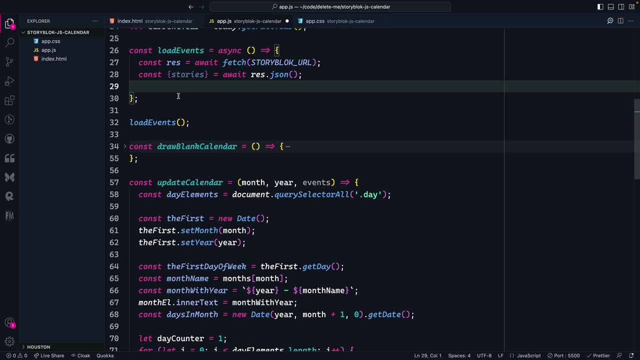 but i want a quick way to figure out whether or not the day of the story or whether or not we have an event for each day as we iterate through uh and update the calendar. so to do this, we're going to transform this story's data and we're going to build up, uh, what we can kind of call a map. it's. 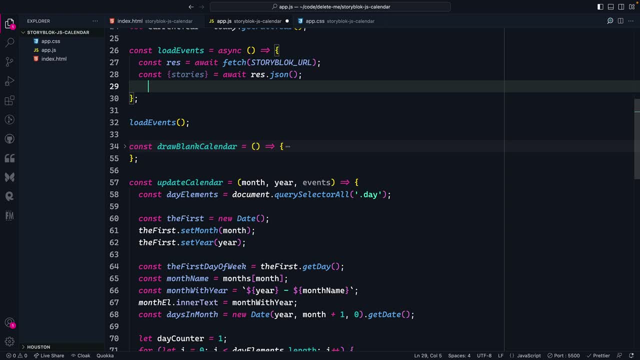 not a. it's not a specific map inside of javascript, because they have a different thing for that. but objects in javascript are key value pairs and we can uh search to see if an object has a key value pair by the key which we're going to use as the date time. so maybe a little complicated, let's. 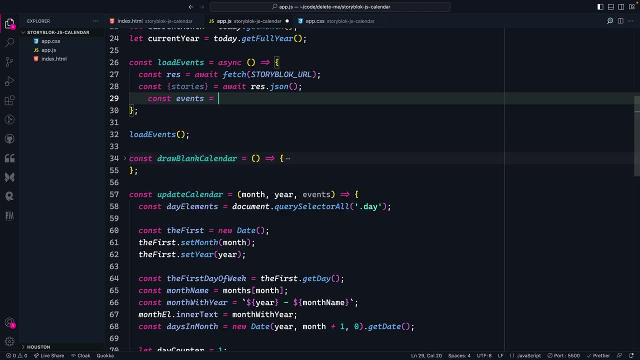 actually, uh, go ahead and walk through this. so we're going to say our events is going to come from our stories array and we're going to call reduce. now stick with me. a reduce is a function that takes in a callback function, and that callback function takes in two parameters: the 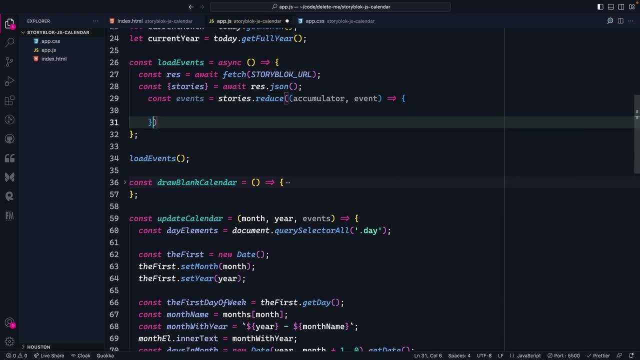 accumulator, and then the individual event that we're iterating through, and then the second parameter is: what is the data that we're going to start with? so we're going to start with an empty object and then for each object, we want to add a key value pair, where the 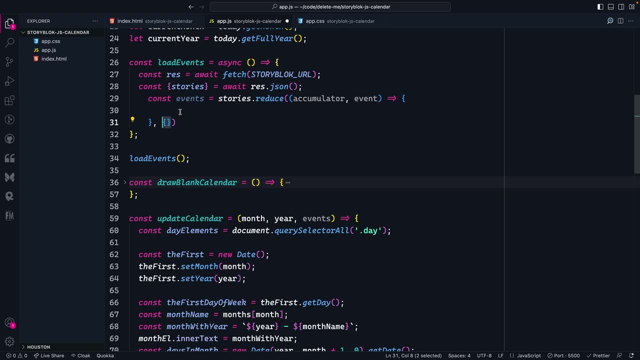 key is the uh date without time, so just the day, and then the value is the actual content of the event itself, if that makes sense. so we can start with the event time and we can create a new date from eventcontenttime. so those properties that we 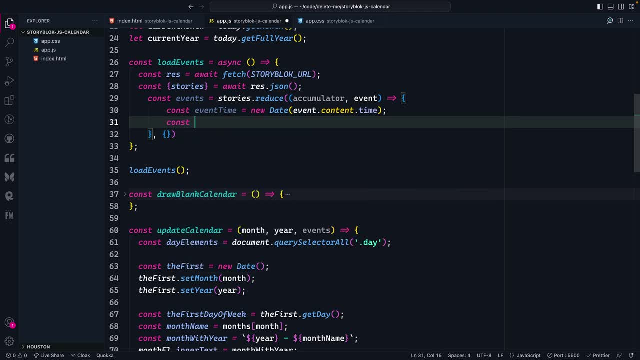 are on the content property of the event and then we can say the event date is going to be a new date and we can say: event date, event time dot to date string. so basically what we've done here is we've created a date from the time of the event and then we convert that to a date. that is date string. 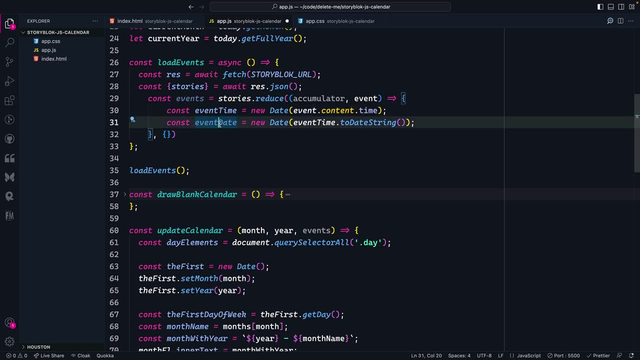 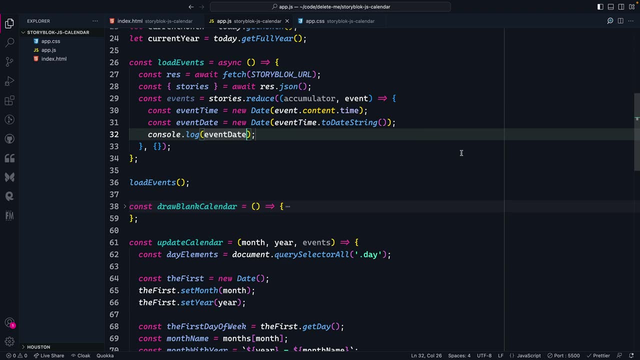 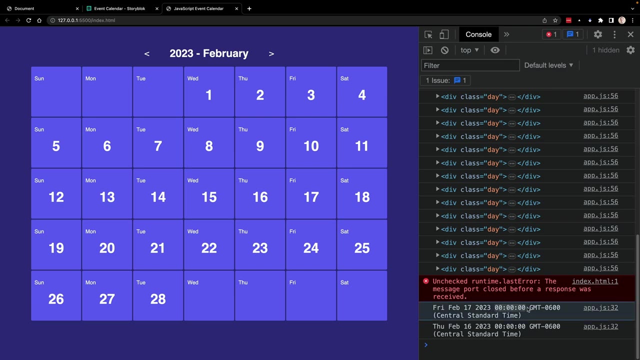 format which gets rid of the time. so this is just the. this event date now only includes month, day and year, so if we actually log this out, we should see each one of these. so you see, this is friday, february 17, 2023, but then the hours, minutes and seconds are all set to zeros, which is what we want. 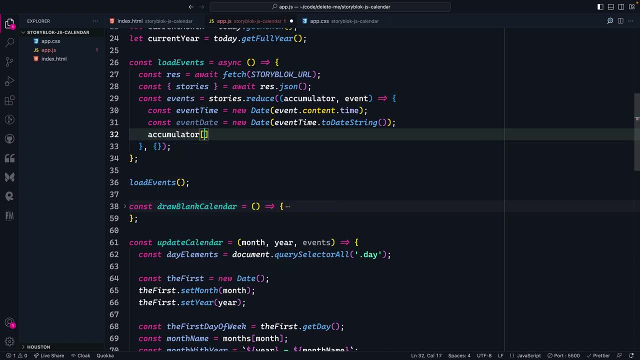 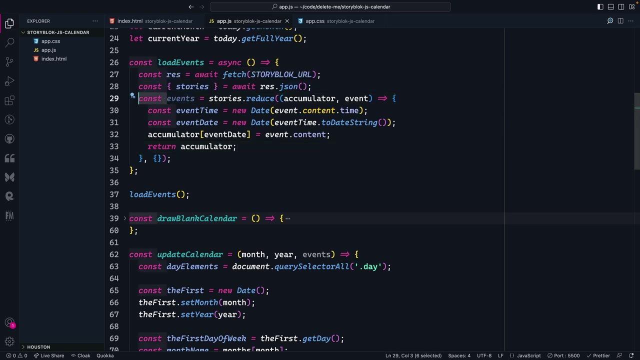 so, when we have that string now, we're going to take our accumulator and we're going to set the event date as a key and the value is going to be eventcontent. lastly, we're going to return that and, instead of setting this to a local variable, i'm going to create a global variable for. 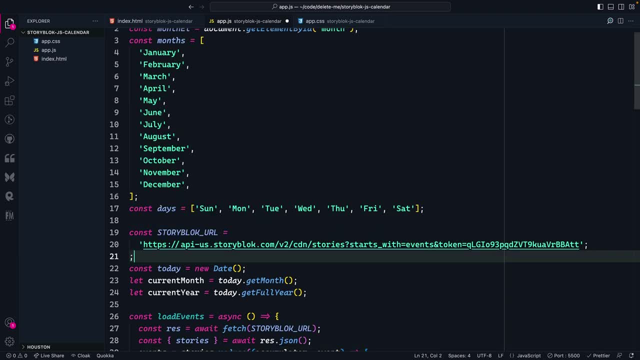 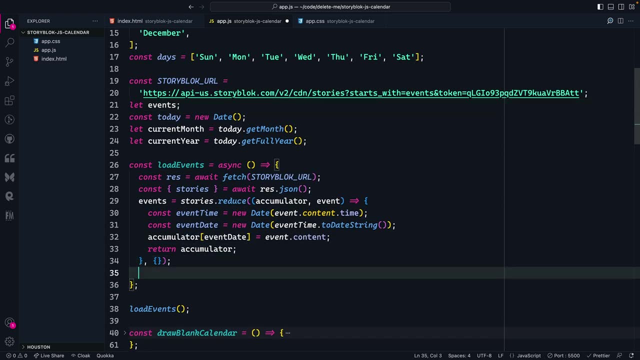 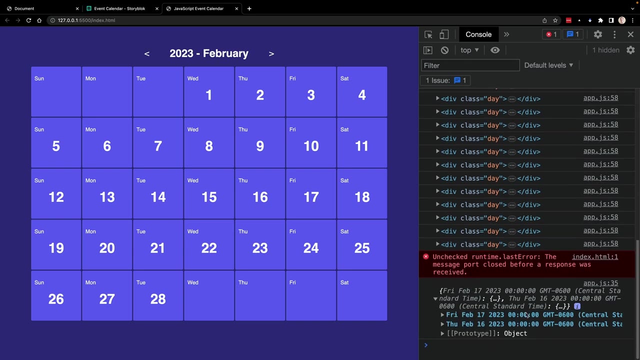 events. so i'm going to create a variable up here, just say let events, and that will get updated when we actually load those events. so at the end of this let's log out events, just to see what this looks like. so this is an object where you have the two keys, which are those dates without the time, and 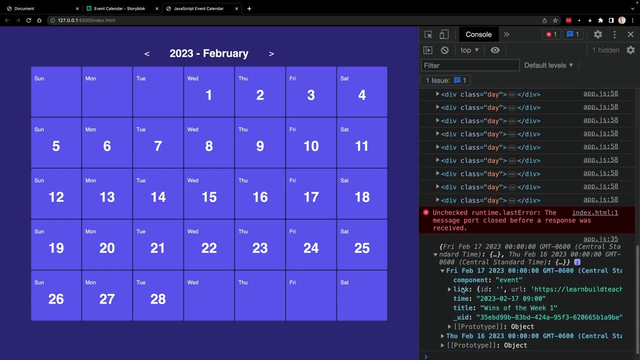 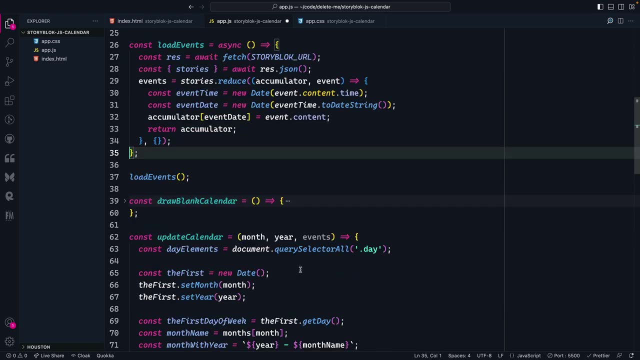 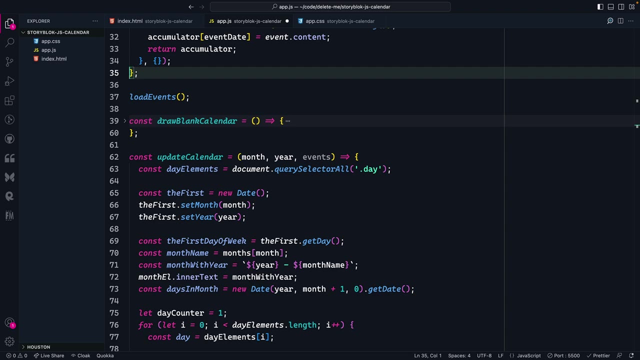 then inside of here, you see the actual content of that event, so the link, the time, the title, etc. all right, so that is working well. now, when we update our calendar, we want to know if, for the given date that we're on, if there is an event that matches that. so let's scroll down. 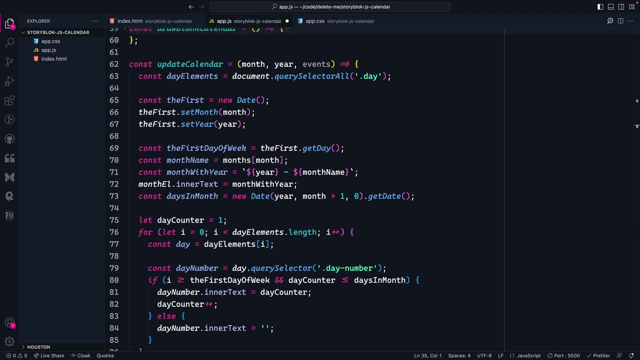 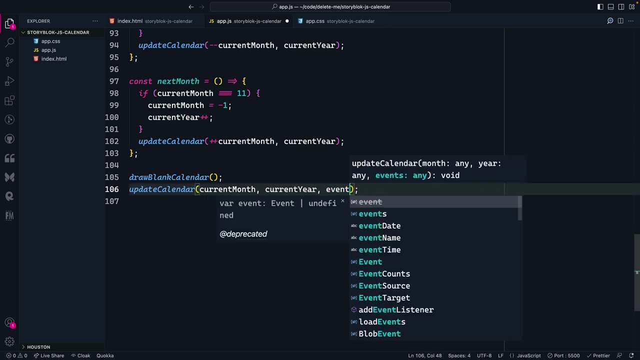 to. actually we were in the right place. so to our update calendar function and remember we said we were going to pass in the events, so we want to pass in the events here. the problem is these events haven't actually been loaded yet. so what we'll do is: we will make sure. 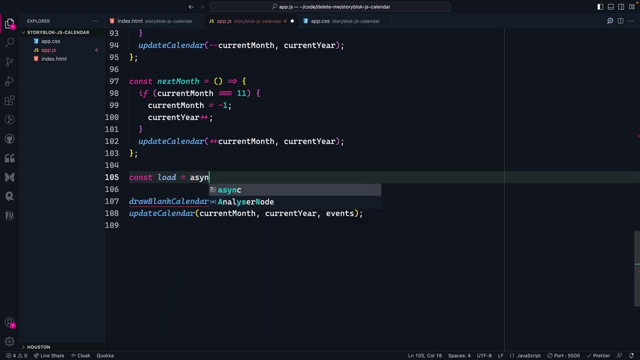 they're loaded by creating a load function. this is going to be an async function and we're going to await load events, so we'll make sure that all those events are loaded, then we'll draw the blank calendar, then we'll update the calendar with the events and then, lastly, we'll call load down here. 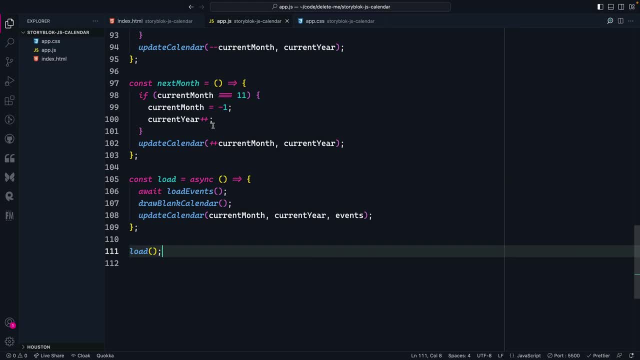 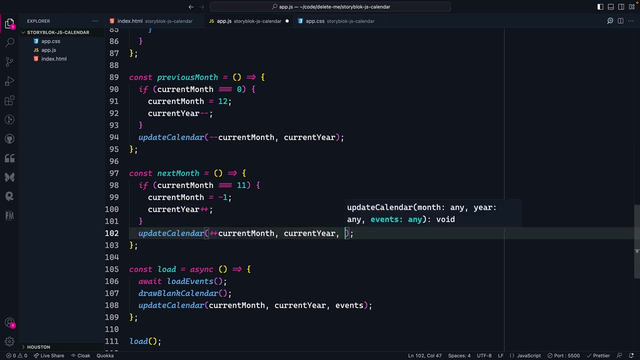 so everything should still work the exact same, but now we should have access to our events inside of the update calendar function. now the other thing we'll need to do is also update the next and previous to pass in events as well. all right, so those will get passed in. 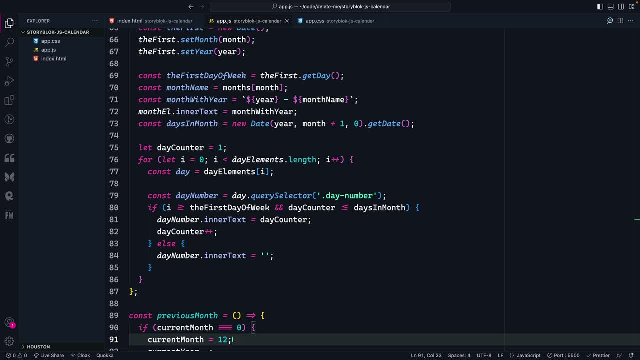 now we need to add the logic in here to decide if there is an event for a specific day. so to do that, we need to get a representation of the day that we are currently iterating through, in the same format as those keys that we mentioned earlier. so to do that, we can. 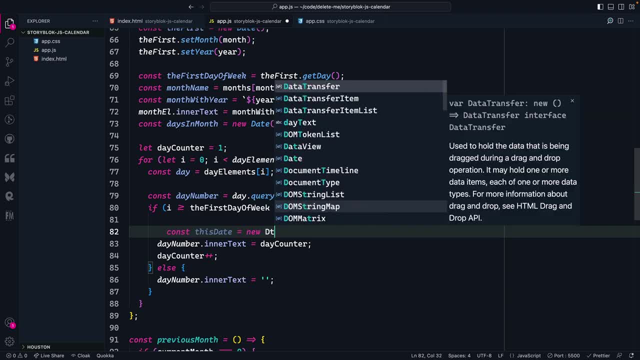 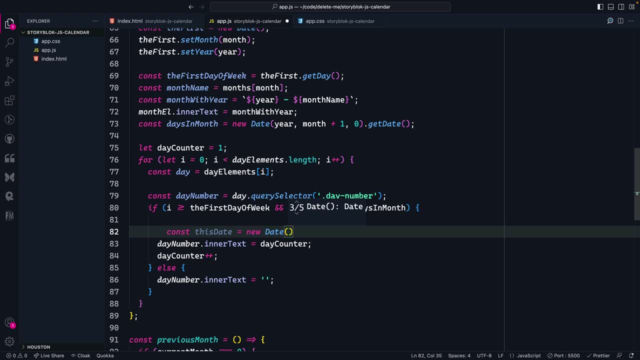 create a variable called this date. so the one we're currently working on and we'll say: this is a new date and i think we can set: we can pass in the day, month, year. so if we pass in day, counter, the month and then the year, let's log this out and see if that is what we think it is. so this should. 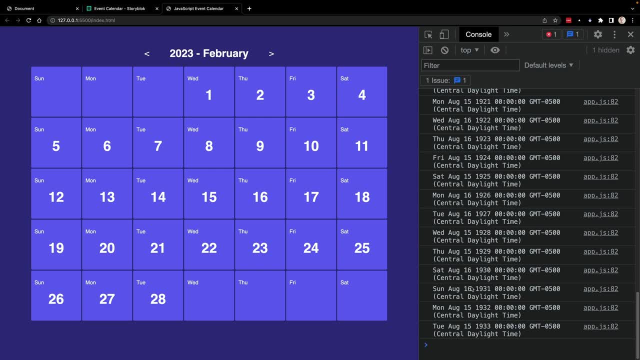 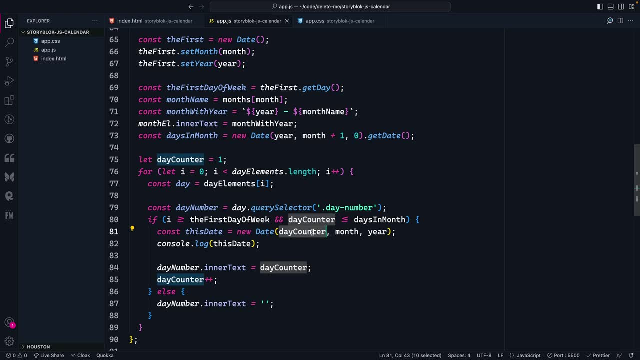 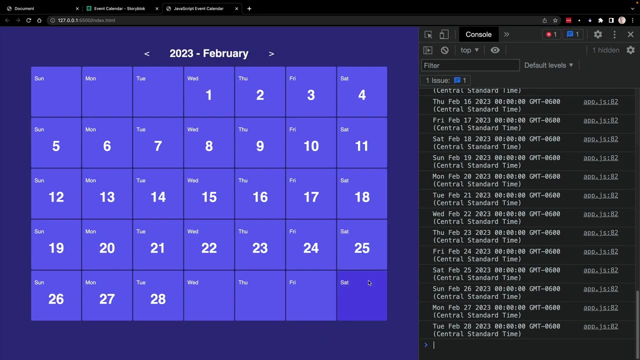 be more of the year, since we could just start over here. now. what happens is you? we've got a bunch of these and it looks like it's almost right, but not quite so. it looks like the day on here or the year we're passing in in the wrong order, so maybe it's year, month and then day counter. 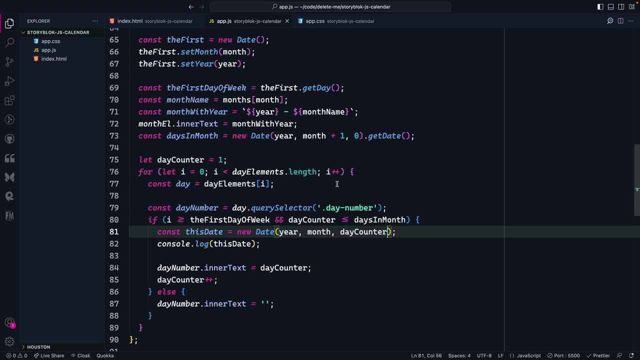 all right, so that looks right. so we've got. we're iterating through each one of these. notice. the time in here is zero, so that should match what the we just formatted. So now we want to check if that exists So we can say if events of this date. 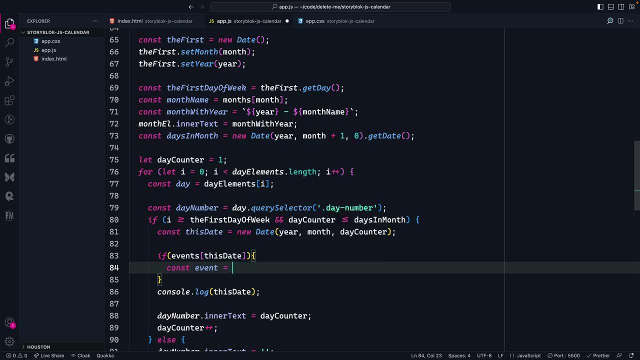 if there is one now we want to get the event. So we'll say: event equals events this date, All right. then we'll say the event name is the element, is the day query selector. So we're querying that event name And then we can take our event name and set the inner. 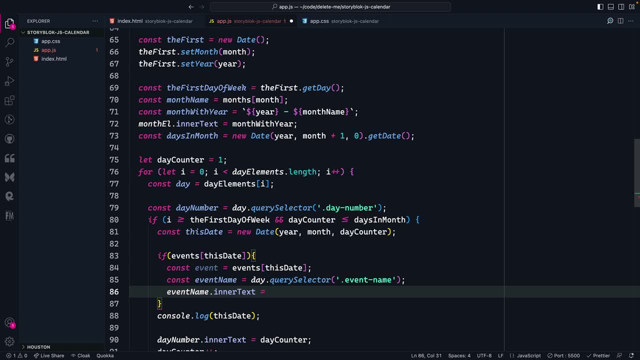 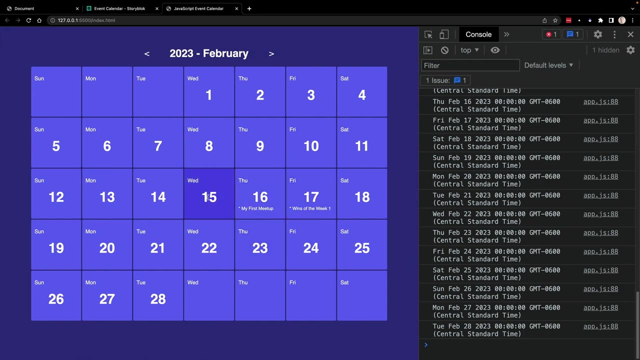 text property to be. we could just set it to the event title. I'm going to add just an asterisk or like a bullet point to this, basically, and then add in the event dot title. All right, so now if we go back we should see that it is showing my first meetup and wins of the week. 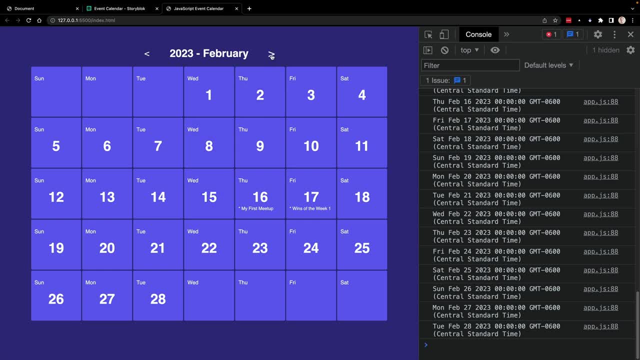 which is really nice. This is pulling live data from Storyblock. Now, one issue here is that it's showing my first meetup in Wednesday of the week, So we're going to pull a little bit of that in here And then we're going to go to the next month. notice it still shows. 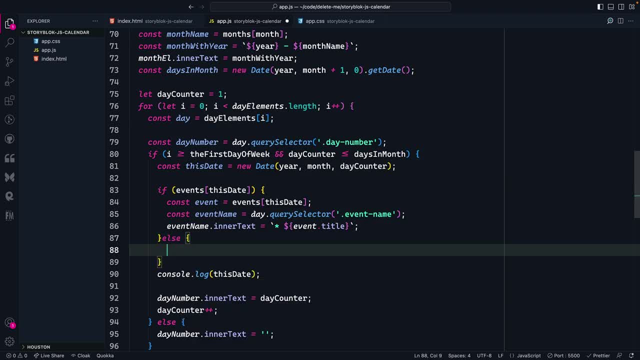 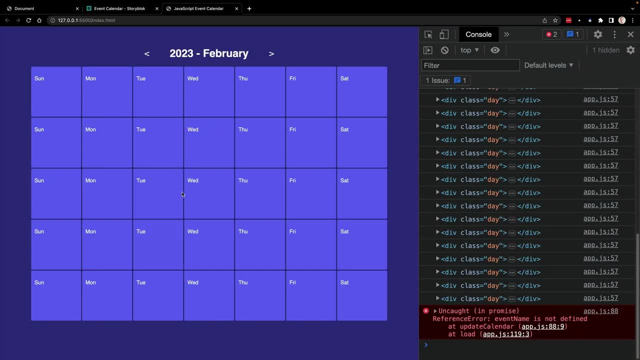 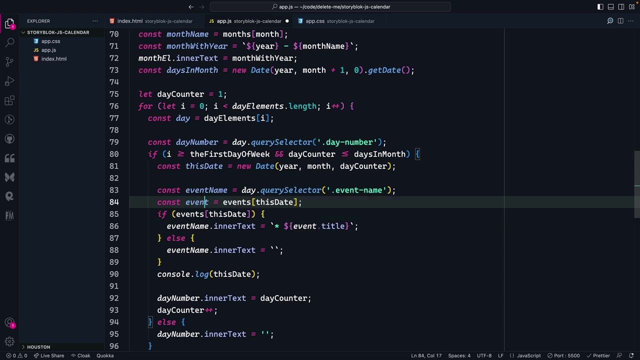 those same events. This means that we need to come down and do an else. So if it, if there's not an event, we need to reset this back to nothing. So we will do that. So on February, where do we say event name, dot intersect? Oh, this should be queried up here. So, like this, like that, I. 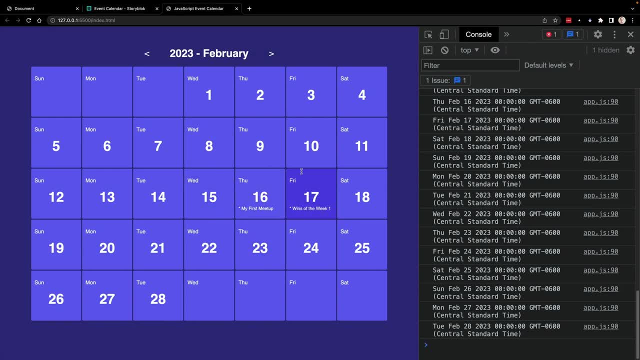 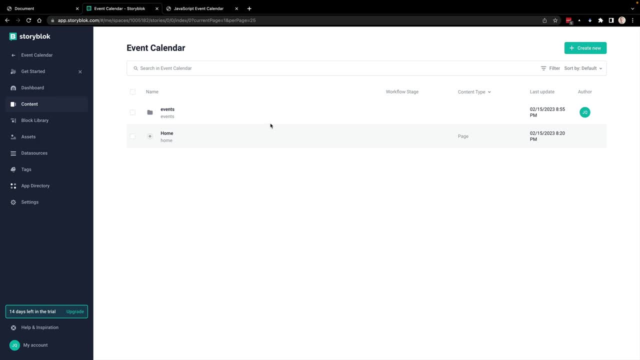 believe. So we'll get that event name and then we'll update it regardless. So we'll see: first meetup Wednesday of the week And then we'll do our next one. And there's nothing there Now to show that this is still live. Let's go back to content. Let's go into events. 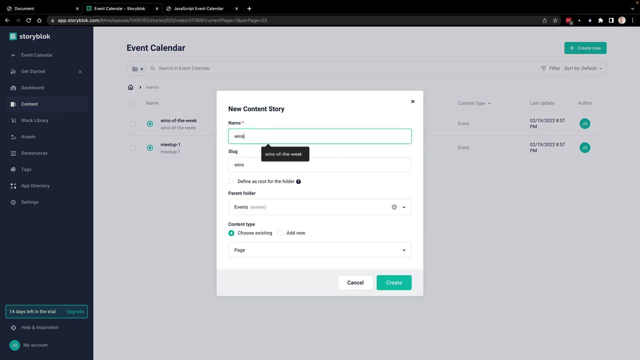 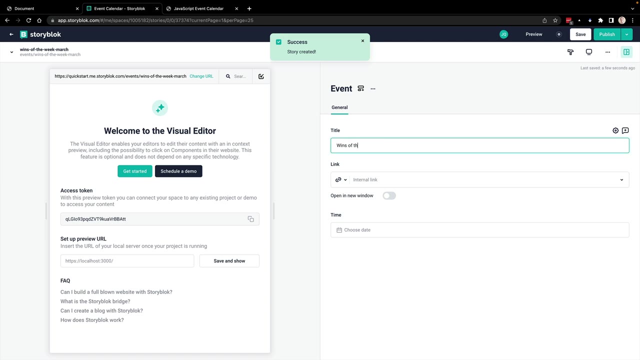 Let's go create a new story. This is going to be inside of, inside of the events as well. We'll call this Wednesday of the week, March, for example, and we'll say: this is going to be of type event. We'll create that. We'll call this Wednesday of. 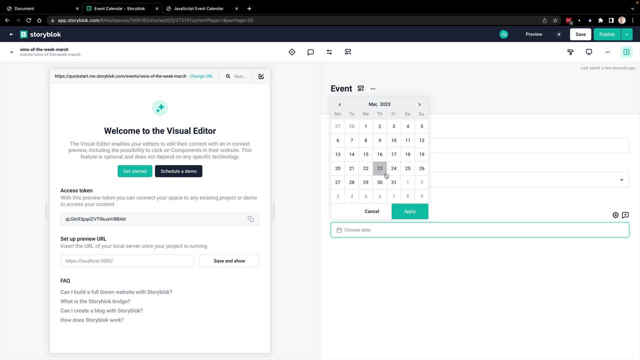 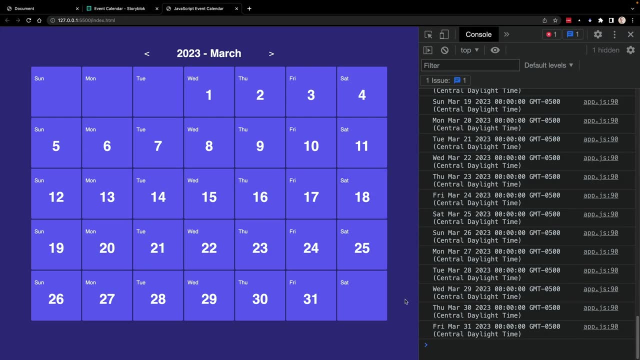 the week. We'll then choose a day in March, So March 9, apply. publish this. let's go back and refresh our calendar. So right now in March, it says nothing. we refresh, we go back to February meetups there- And then, if we go in to March now you see that it's loading all the data each. 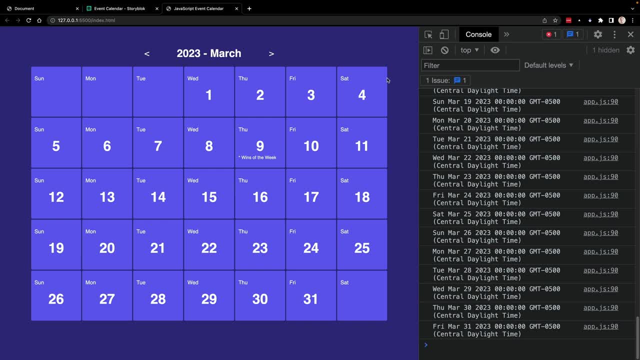 time from Storyblock. So I just think this is a really cool exercise to practice your vanilla JavaScript to get comfortable with DOM elements, querying API APIs and then working with external data sources like Storyblock, which I think is a super, super common thing to do. I use headless. 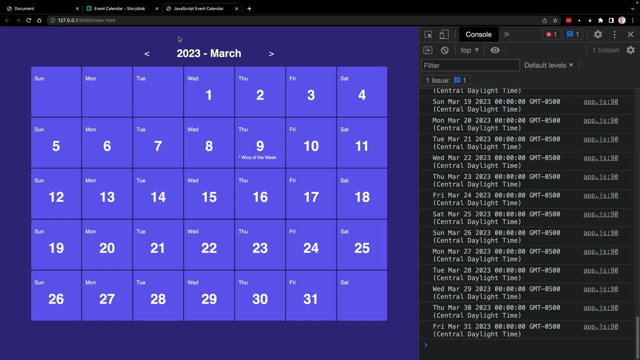 CMS is for a lot of the projects that I work on. Again, big fan of Storyblock, Thank you to them for sponsoring, but they've got an awesome product, So I hope you enjoyed it. So let's talk really quickly about what could you do next. What are some of the things that you could do to kind of 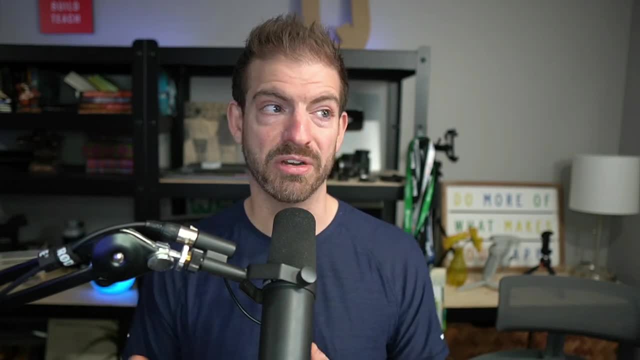 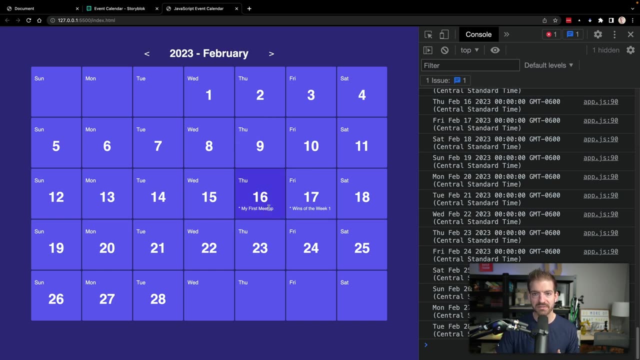 take this to the next level, to add some additional features, because this is not perfect. So one of the things that you could do is for these events, add like a sidebar of some sort So you can see the details of the event. you can make this little piece of text, you can make this little piece of. 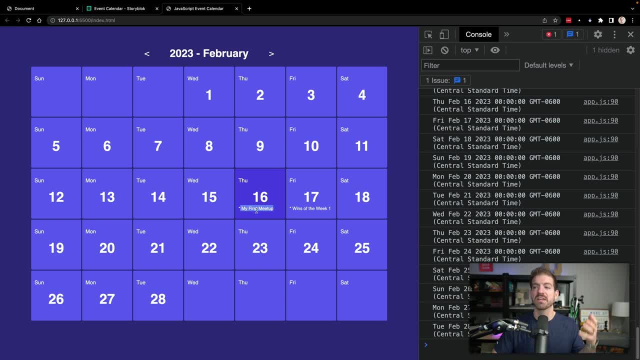 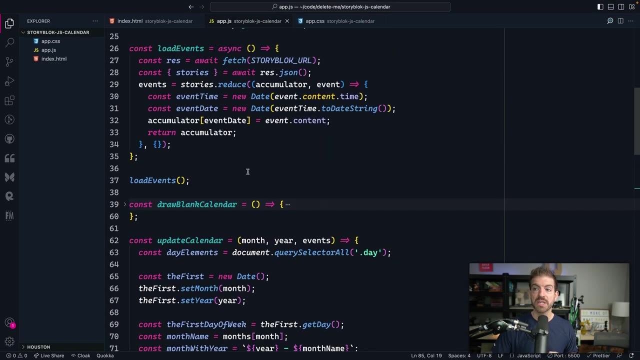 text clickable. you already have the link in the data. in Storyblock you can make this an anchor tag and actually click on that to be able to open it. Now the other thing we don't have is the ability to do multiple events on one day. So this is tricky. because we created that, we converted 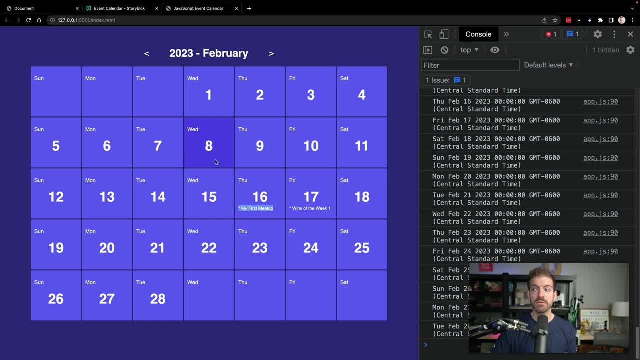 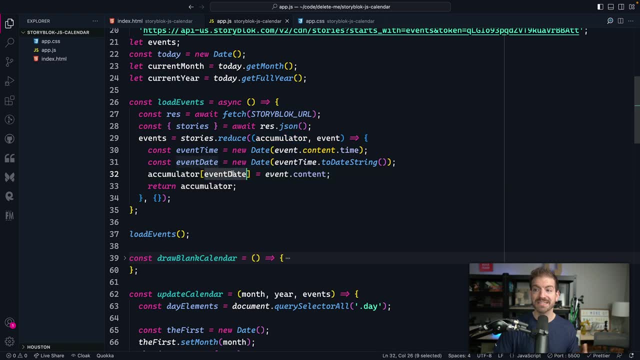 the events into this key value pair thing, where the key was the actual day. So what would you do if you had multiple on that day? Well, for that key, you could set the event date to an array, for example, that includes the content inside of it, But then you'd have to check in here. 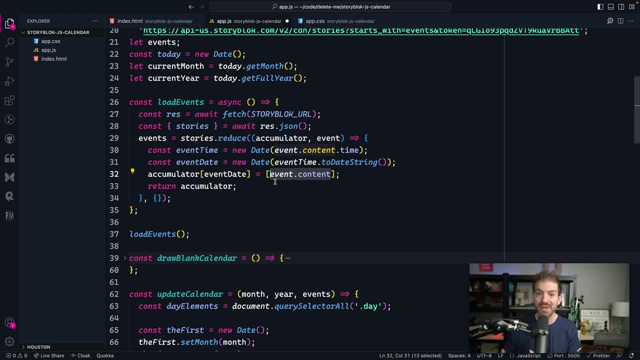 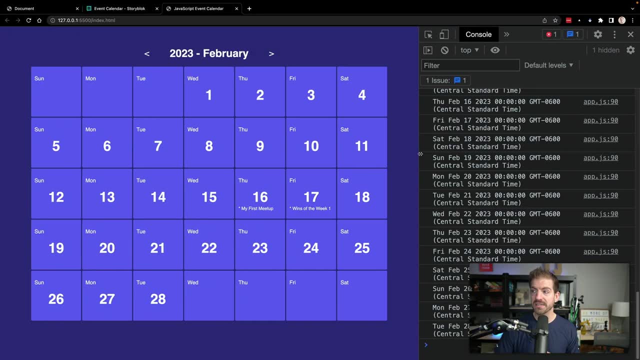 if that key already exists. instead of creating a new array, you add on to the array. So that would be a fun challenge that I think would be really good. Mention the sidebar idea. Again, you can make this, come out all the way and create a sidebar to view the details of the events. 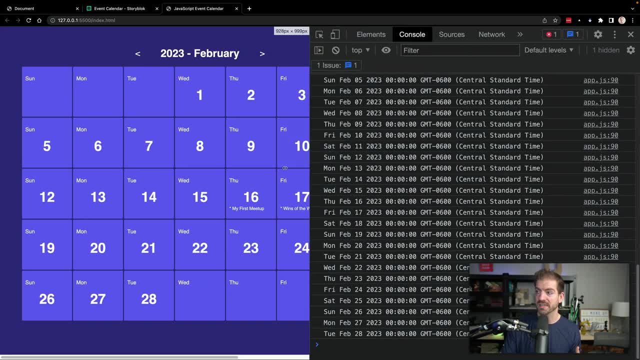 you can make the calendar more responsive. So this is not responsive at all right now. if we just scroll down, we're just going to miss it. So how could you make this smaller? Could you add a new key? Or could you add a new key? Or could you add a new key, Or could you? 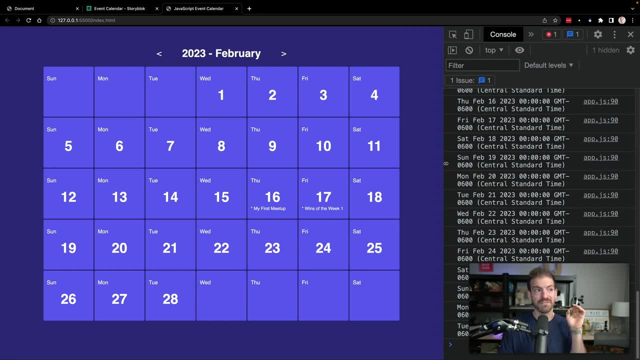 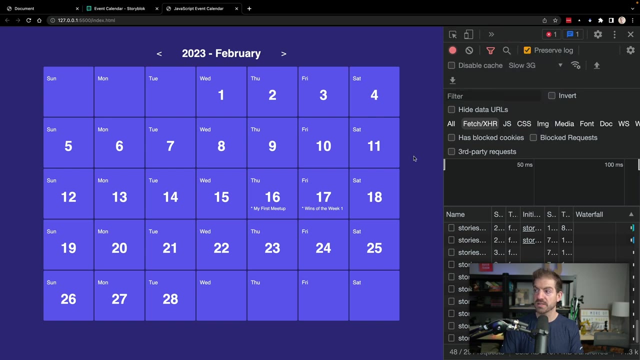 add a week view. Could you toggle between the view of the week and the view of the month, example, or stuff like that? And then, lastly, if you notice, we what's? let's do a slow internet connection. So if we go to network and throttling and do slow 3d, 3g, what we'll notice is this is going to not show. 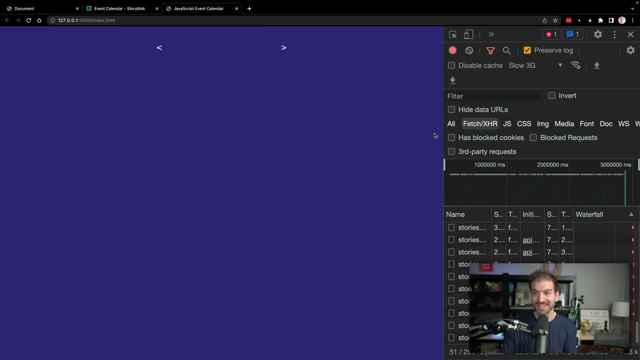 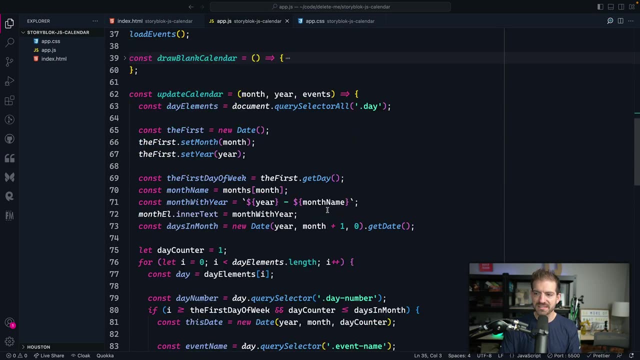 anything, basically for until we load our data from Storyblock. So if you see in here it's trying to load the data, it finds the data. it's trying to load the data. it finds the data. it's trying to load the data. it finally gets it. So one of the tiny things that we could do is when we actually 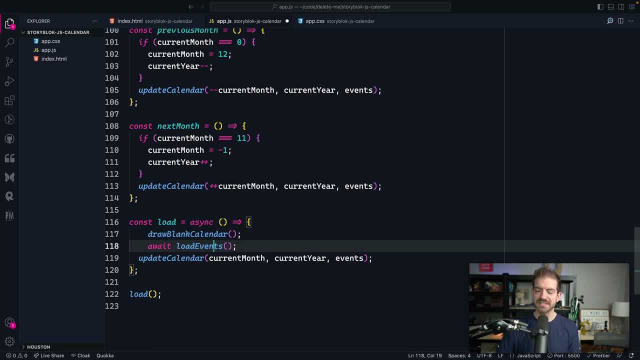 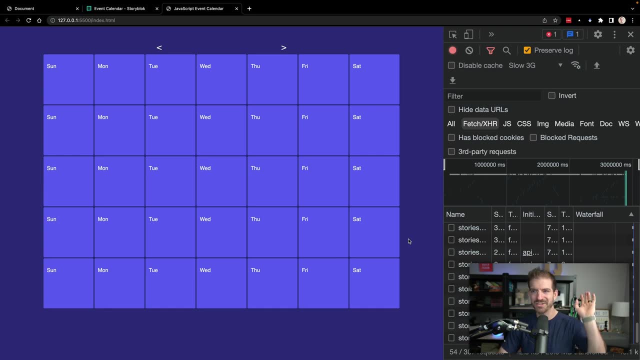 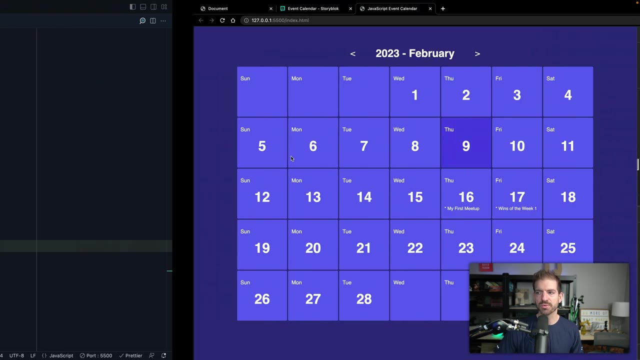 do our loader. we could load events after the draw blank calendar, So that would at least show the blank calendar first, So we'll see the link calendar there, And then we'll load in the event. So that works. The annoying thing about that, though, is we don't have the actual numbers. 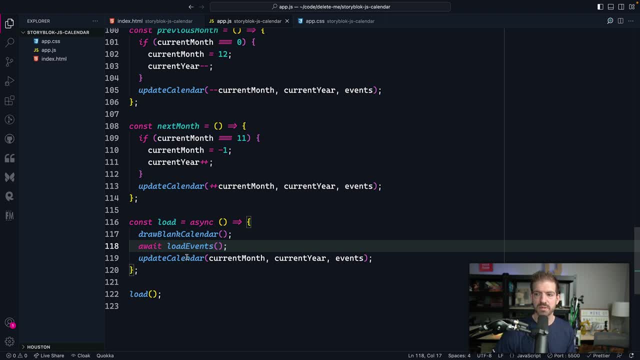 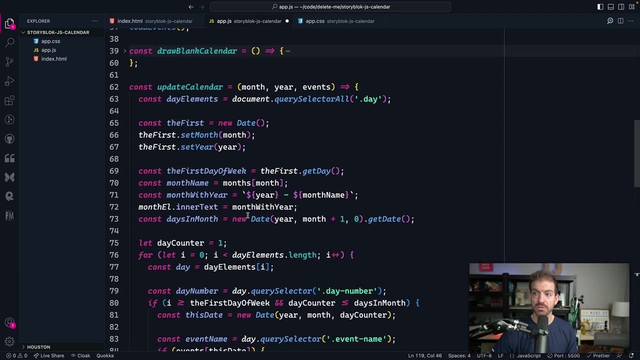 either. So an additional thing we could do is we could not call, not call update calendar here, or we actually would call update calendar but we could pass it in events thing of basically an empty object And then when the when the events are loaded up here, so when we actually 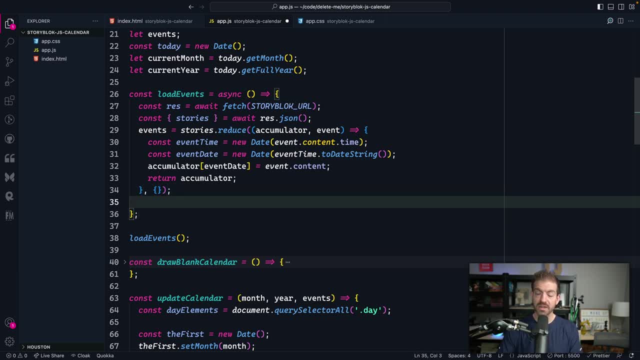 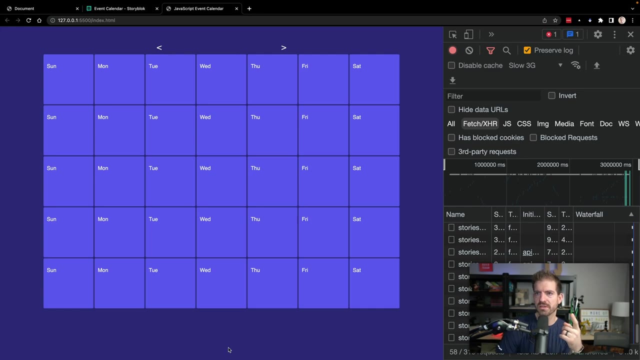 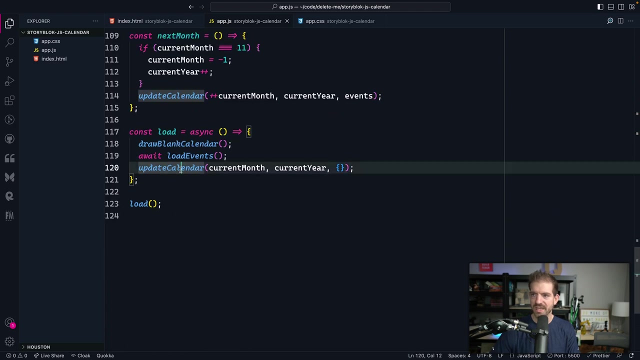 load all of these events and format them. we could call again, update calendar and pass in current month, current year and then events. I believe this will do what I think it will, So this should show all the numbers as well. maybe not. did it not do that? I think I forgot to move them. Yeah.